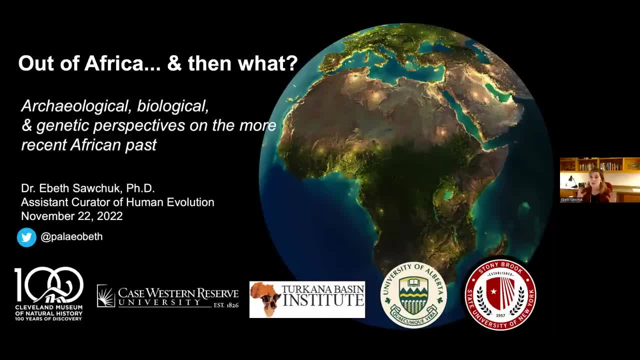 works with a lot of different topics in human evolution and trying to understand the history of our species, Homo sapiens, And I just want to say before I start, as a content warning, that I am going to show images of archaeological human remains from my work, and I do so with 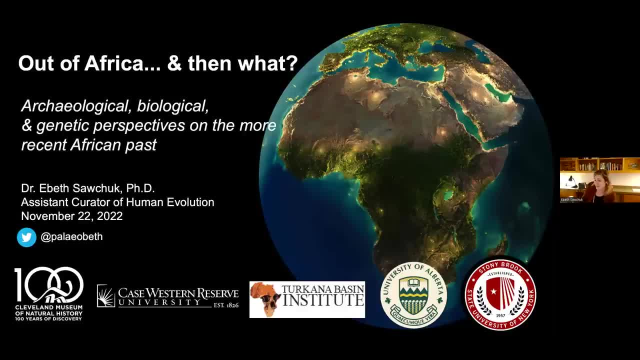 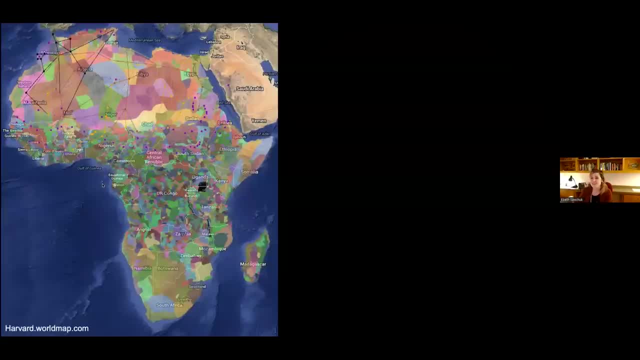 respect in order to tell the stories of those individuals. Okay, Africa is really big. That's the take home from this presentation. Not only is it really big, but it's one of the most diverse places I've been to, but it's also a very different place to be The place. 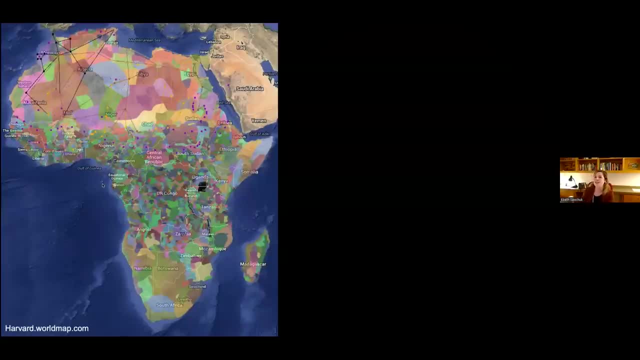 the planet Today. it's home to over 2000 distinct ethno-linguistic groups and over a third of the world's languages, And this makes complete sense. It's where our species evolved. It's where we've been around the longest. However, that also means that African diversity is often talked about. 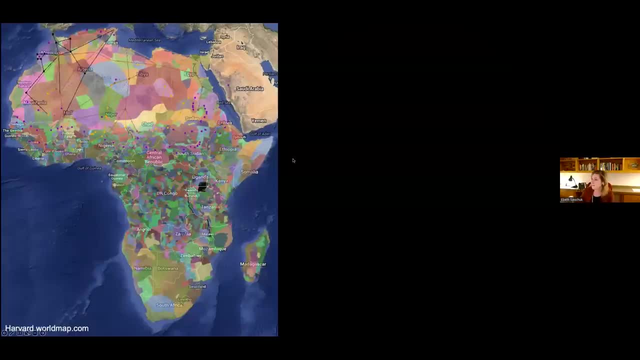 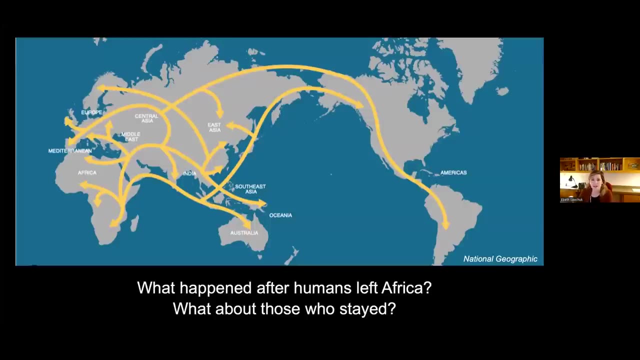 our deep past. So images more like this. We're also not so great as anthropologists and scholars of the human past about talking about Africa after our species, Homo sapiens, left. So what happens after out of Africa? We are more likely to talk about kind of that big migration and when. 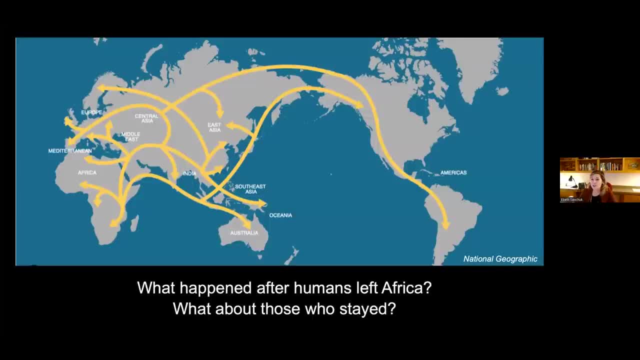 humans spread around the world. We're not great about talking about what happened on the continent after our species left about 60 to 80,000 years ago, and about the many things that happened on the continent afterwards and the impact that had on the rest of the world and our species. 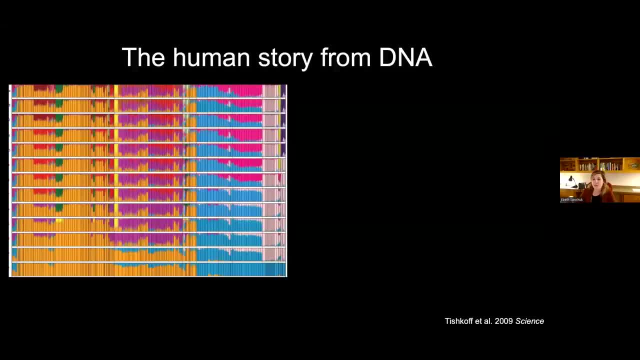 biological diversity. But particularly in the past 20 years, and especially the last 10,, our understanding of the history of our species has really become a lot more nuanced with the addition of various genetic and genomic methods, And so things have changed a lot with advances in DNA research. So we know from this 2009 paper: 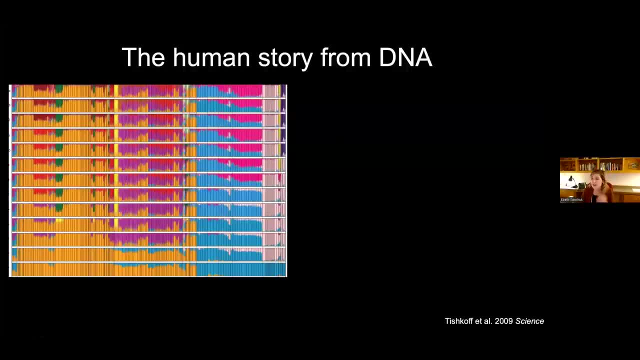 that African genetic diversity is really great. This is an image from a 2009 science paper that shows modeling modern human genetic diversity. All you need to know about this figure is that it's really great, And so we're not so great about talking about African genetic. 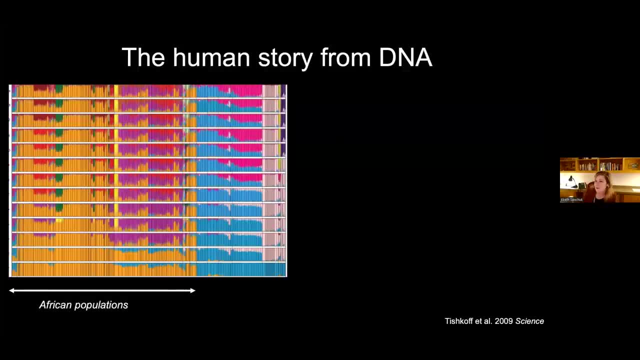 diversity, And so we're not so great about talking about African genetic diversity. All you need to know is that more colors equals more diversity, and you can see, here we've got African populations and then the entire rest of the world. So, according to everything we know, this makes 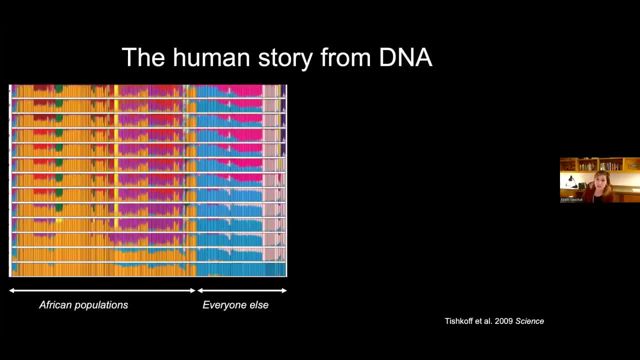 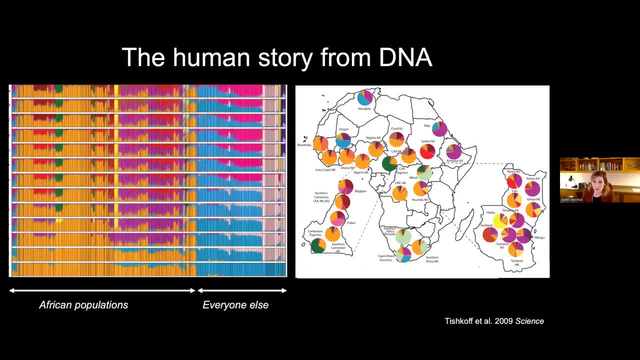 sense Humans evolved there and have been the longest, that African human populations today have more diversity than the rest of our species combined. and we also know that this diversity is very regionally substructured and that some of regions of Africa are particularly complicated. So again, this is from the same paper and it shows, again, modeling living people: human. 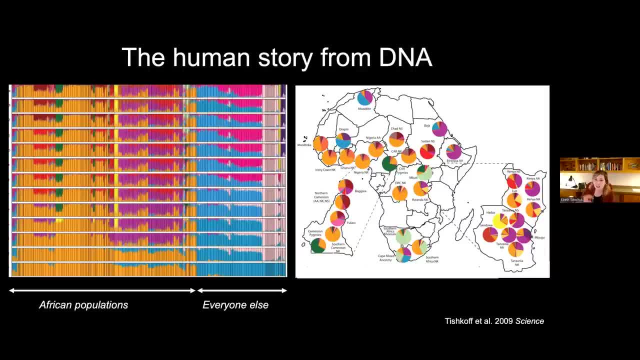 diversity in these series of pie charts and some places they actually had to blow out sections of Africa, So for example Kenya and Tanzania where I work to fit more pie charts. So we know some parts of the continent were particularly complex in terms of structuring this genetic diversity. 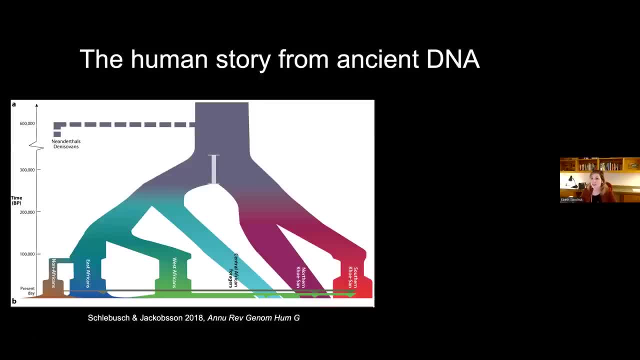 So, more recently, ancient DNA has entered the chat, so to speak, and this has allowed us to look at the genetic diversity of African populations. So we know that this is a very complex population, and we know that this is a very complex population and we know that this is a 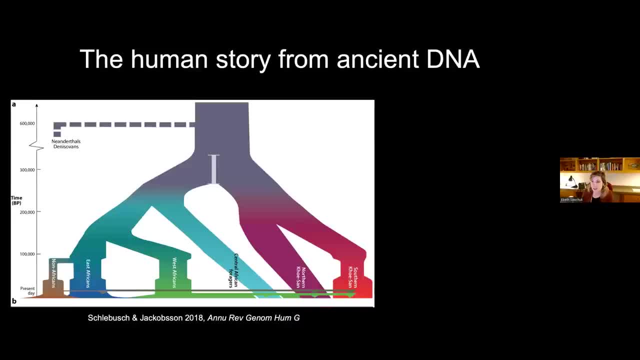 ancient individuals and estimate the timing of our species evolution. So all of these branches here represent deeply divergent African populations that all coalesce around 300,000 years ago and this suggests this is when Homo sapiens emerged. Of course that's a very contentious. 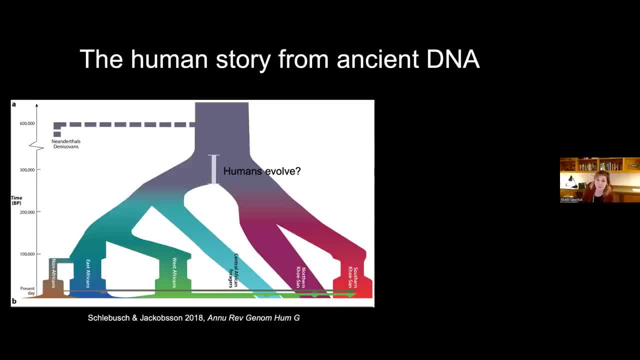 topic about what that exactly looked like, but this more or less accords with the fossil record, and so we're pretty sure this was important timing in terms of the appearance of people who looked more or less like us and had the same population. So we know that this is a very complex population and we know that this was important timing in terms of the appearance of people who looked more or less like us and had the same population. So we know that this was important timing in terms of the appearance of people who looked more or less like us and had the same 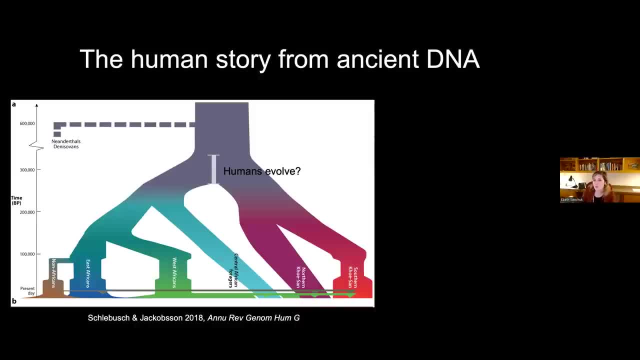 capacities more or less like us. But there's also something important: when we look at a map like this or a figure like this, Not only are we looking at the coalescence of our species, but we can see that in the last 5,000 years in particular, all these lineages start blending. 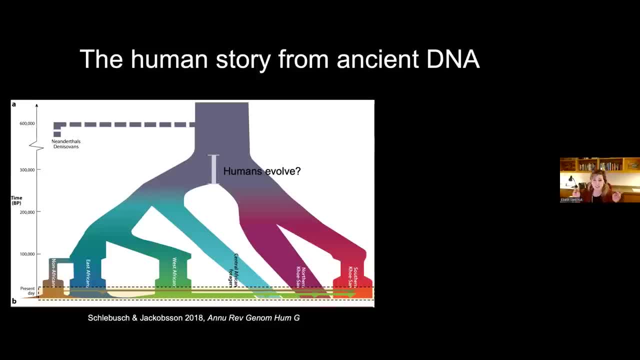 together. You know, I would characterize this as when the figure gets fussy. it's a scientific term. but you start to see a lot of things start blending together, a lot of boundaries become indistinct, and so it really begs the question: how have things changed in the past 5,000? 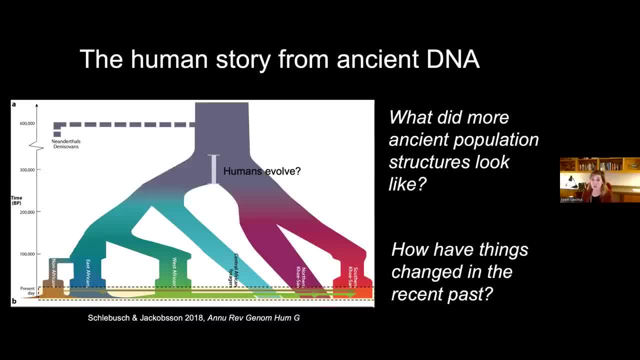 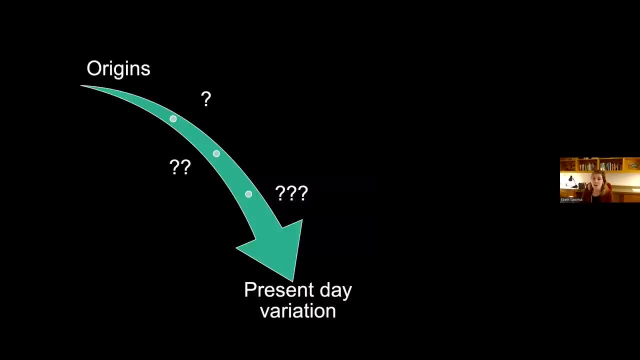 years in our species, Homo sapiens. And then, of course, an even more dire question: what did more ancient population structures look like, if we know there's been massive demographic reorganization in the recent past? And so kind of setting up the big concept of my research and 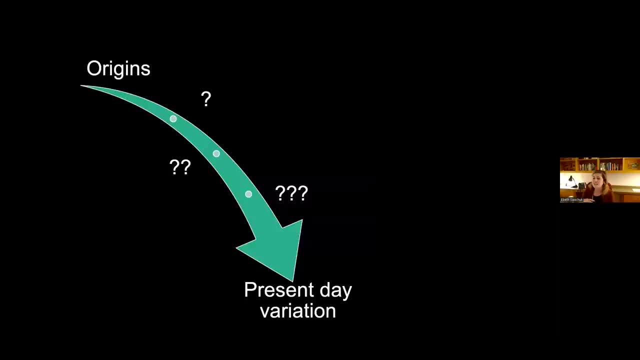 my curatorship here at the Cleveland Museum of Natural History is: there's a lot that you miss if you focus on origins, and then there's a lot that you miss if you focus on the present day. There's a whole big, meaty cheeseburger of interesting things. 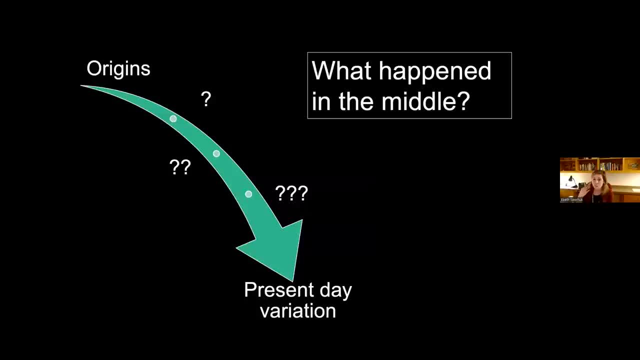 There's a lot of things in the middle that happen to our species, and this is really important for understanding the world that we live in today and why we see the patterns biologically and genetically around us within modern human variation. And so, for me particularly, I like 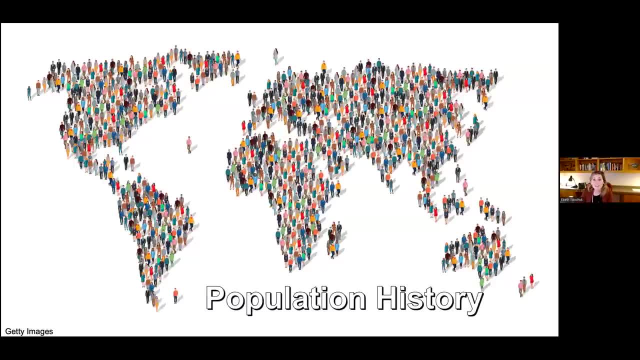 to take on this concept of population history. It's more commonly used in the genetic literature, but I think it has a great application when we study biological anthropology and archaeology, because it really just means everything that happened to our species that make us us. We're not just interested in the beginning of the story, because evolution is ongoing. 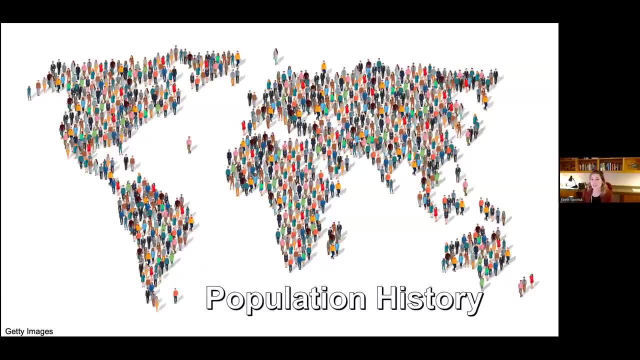 We're interested in the whole story and everything that has structured us and everything that makes the world look like it does today, And so my work is really focused on not only the history of our species, Homo sapiens, but really trying to understand particularly the last 50,000 years. 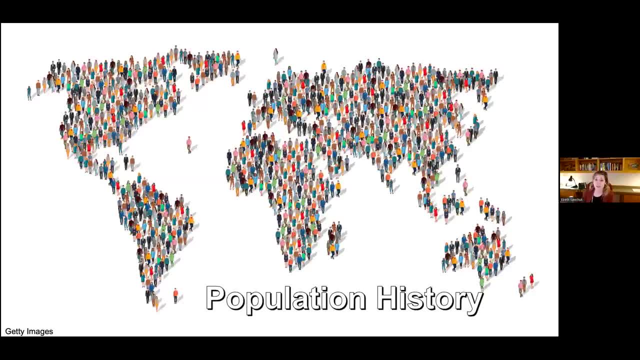 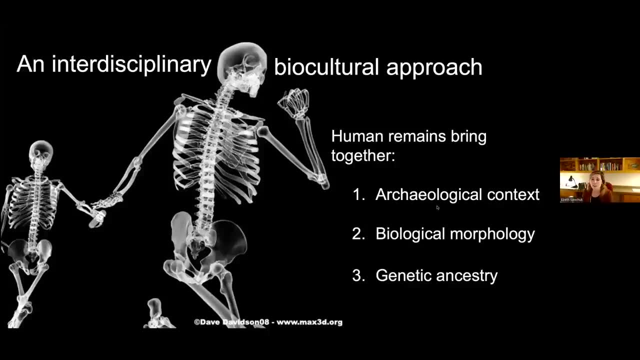 which were really, really meaningful for structuring the patterns of diversity that we now study. And one thing that I think is really important in this kind of approach is really understanding the role that ancient human remains play in this. So my background in training is as a bioarchaeologist, So I study the archaeological context of ancient 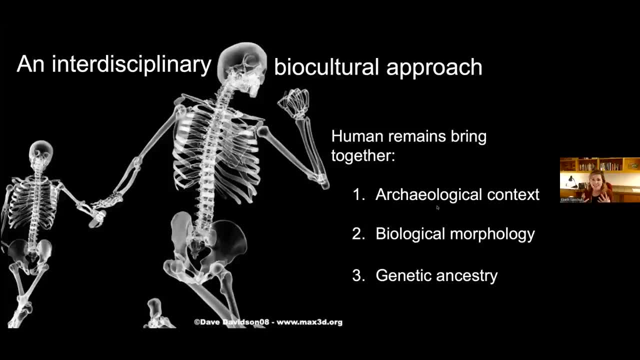 human remains. And that's really important, because humans are kind of the nexus of a bunch of different lines of evidence that help us understand the past. They bring together archaeological context, So understanding how an individual entered the archaeological record and the cultural practices that surrounded that, Of course, understanding biological morphology at 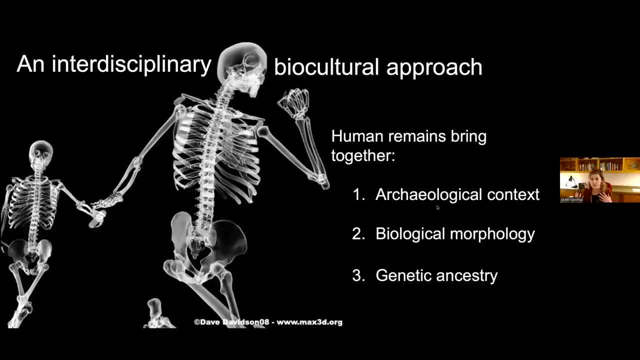 both the micro and macroscopic stages, And so that's what I look to use to answer those questions: level understanding, metric and non-metric traits, looking at evidence of habitual activity and all those kinds of things also, growth and development, And then finally, you know, if you're lucky you. 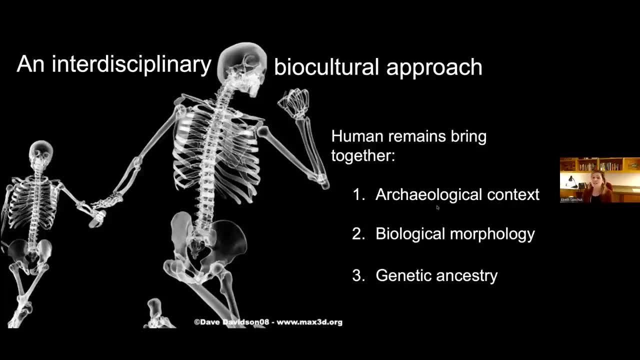 can also combine another line of evidence, which is genetic ancestry, to try to not only understand the lived experience of that individual but also the lineages, genetically, that they come from and what that suggests about the population history of our species. And this is really important because 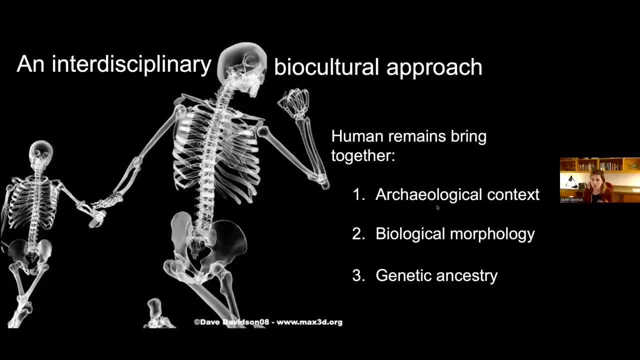 when you put all these different lines of evidence together, you can try to understand what the past was like for the people who are actually witnessing the events that you're really interested in, Because, of course, humans are biocultural creatures. Our biology influences. 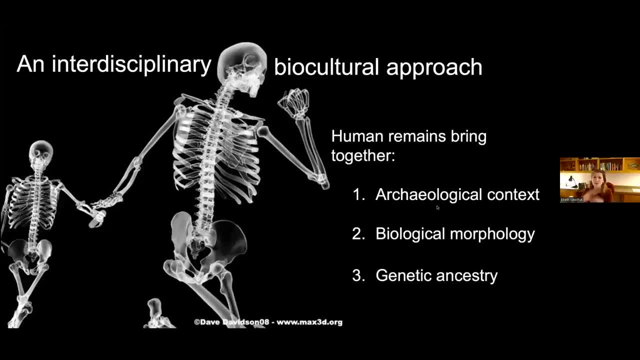 our culture. Our culture then influences our biology. We're a very messy two-sided coin, and you can't quite pull those two parts of us together, And so, in a way, humans are really our best and only direct connection we have to the past. They're the people who were there. 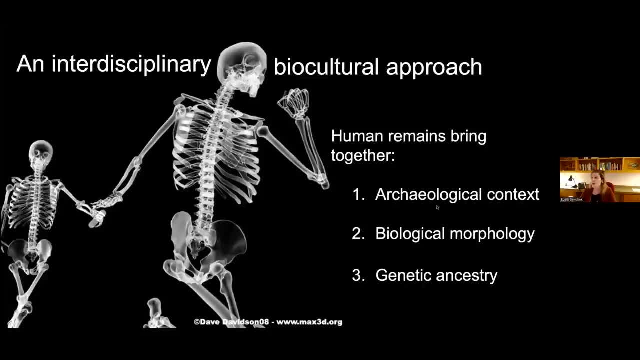 and it's really, really an enormous privilege to get to learn from them, And they really contribute to our culture, And so I think that's really important. They really contribute to the conversations about evolution, something that we can't learn from looking at paleoenvironmental records or artifacts alone. It's something more special. 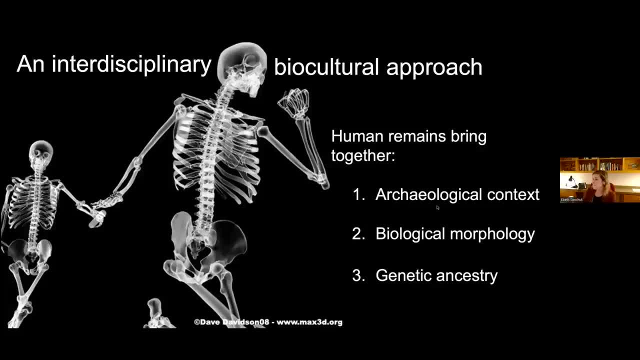 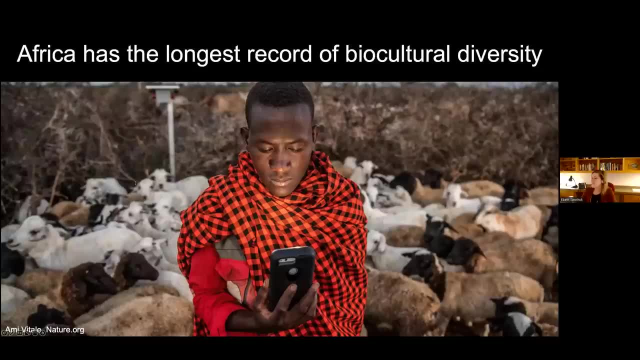 and something really, really rare to look at. There's a big bird of prey sitting up on the telephone pole. So of course this approach could work anywhere, but one of the places that I work and that I enjoy looking at is the African past, because there's the longest history. 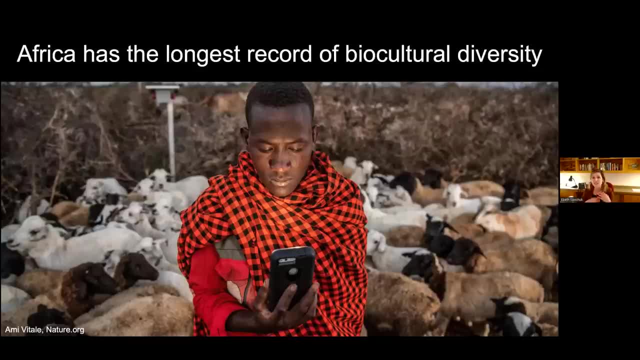 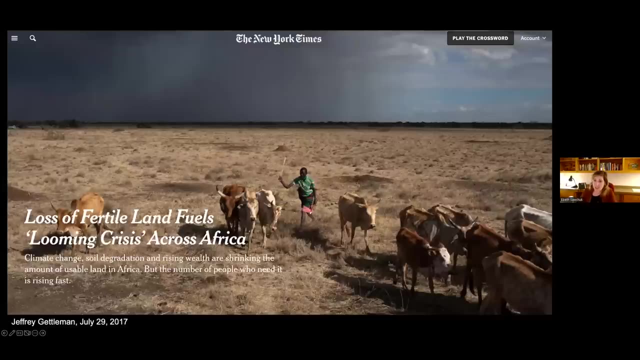 And it's really one of the places that we see so much diversity in terms of both behavior and culture, And it's really interesting to think about how the more recent African past has structured the world that we live in today. Africa is also important in terms of present-day. 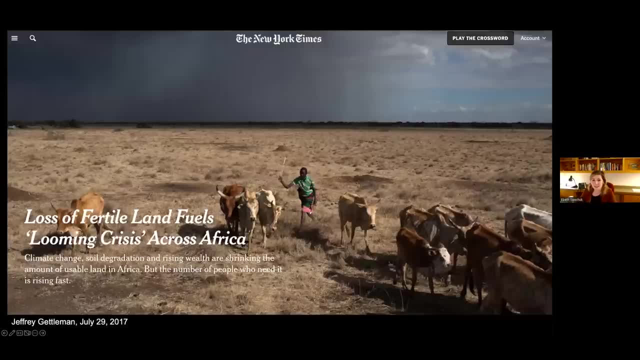 global issues. I don't think I need to tell anyone that global warming is affecting every single one of our lives, but the impact is felt more severely across Africa and many parts of the global south. The situation is particularly dire, and I think it's really important that we 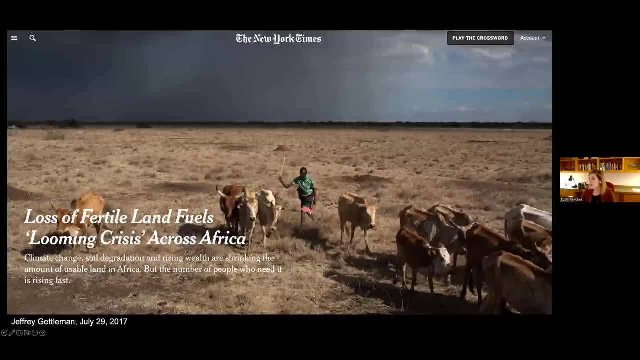 think about that. It's particularly dire across much of dryland, Eastern Africa, where I work, where millions of people live as mobile pastoralists. So this is a traditional way of life centered around herding domestic animals such as cattle, sheep and goats, And it's actually 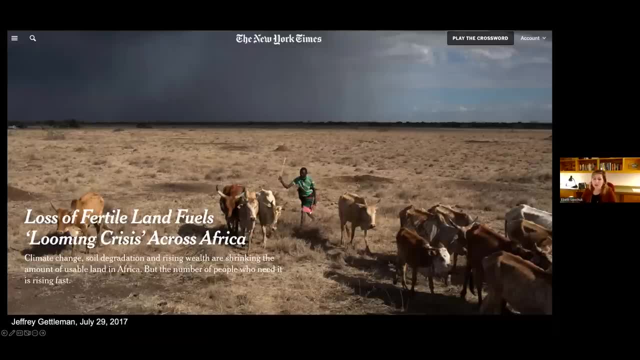 highly adaptive in arid environments with unpredictable rainfall, because it's more efficient to move your animals to resources like water, pasture and salt, versus trying to move those resources to your animals. However, it's becoming harder and harder with global climate change, And this is something that we have to. 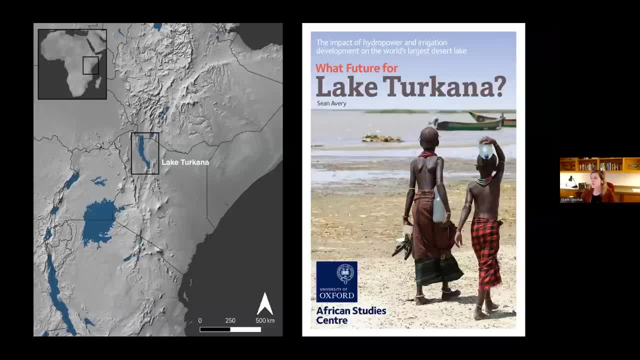 take into account when we work in places like dry land Eastern Africa, because many of the people who live there today have been profoundly impacted by these climate differences, And so one area in particular is Lake Turkana, around where I work. Many of you who have studied under Marc Dallar 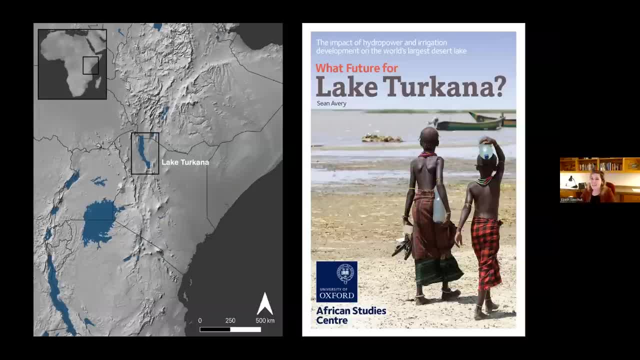 will be very familiar with the Turkana basin, But the lake has been profoundly impacted not only by recent droughts and global warming, but also human activities like hydroelectric dam development on the O'odham River, And so this is a causing the lake to shrink. Now, the lake supports millions of people, most of whom are pastoralists. 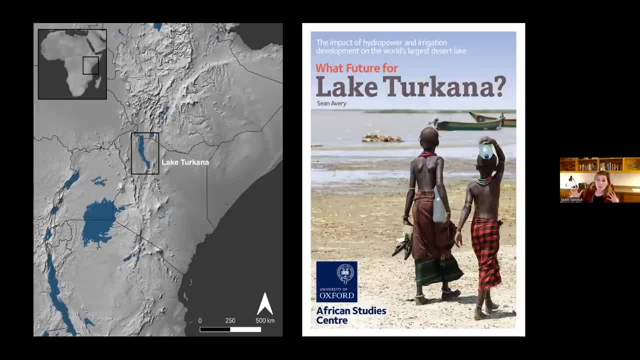 and so it's starting this bigger conversation about the sustainability of mobile pastoralism going forward as water becomes harder to find in many parts of dryland eastern Africa. But what's talked about less is how the fact that this is not the first time that lake has shrunk- 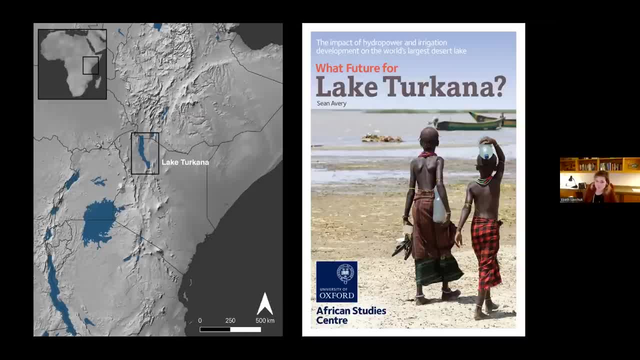 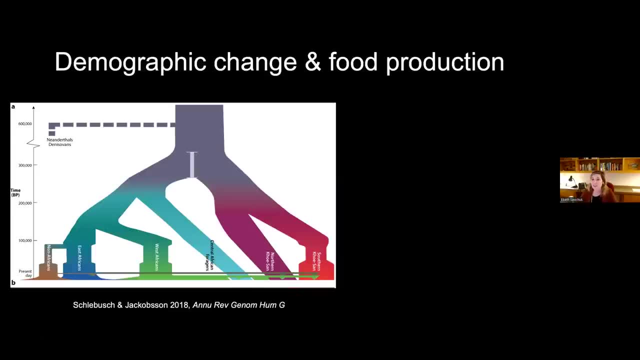 and, in fact, how herding originally spread to this part of the world. So before I can talk about that, I need to give you some quick background on food production. So this is probably a much later time period than your speaker series usually gives you, but this 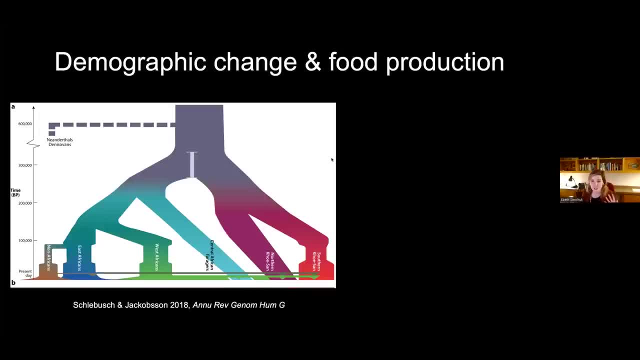 is what I'm illustrating to you, that it's the later parts in human evolution that are still very interesting to understand: population history of our species. So back to this figure. we're talking about the fussiness of the past 5,000 years, all of this demographic change and a lot. 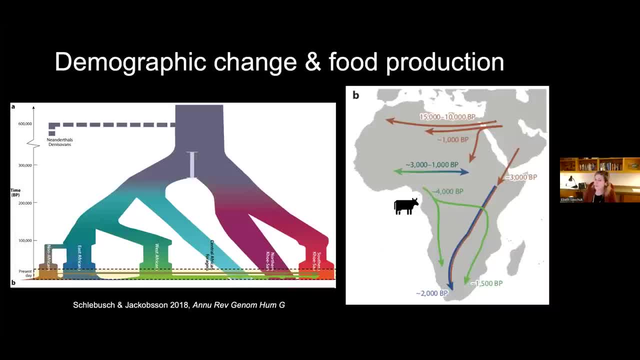 of this can be attributed to the spread of food production, specifically herding and farming, across Africa. So archaeologists have been studying these processes for decades. that's not new. what has changed is now with the addition of bioarchaeology and, more importantly, genetic. 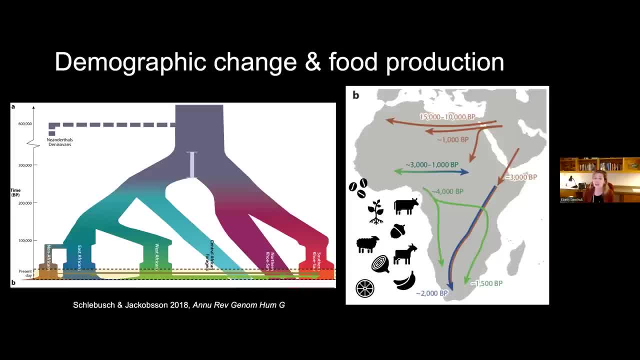 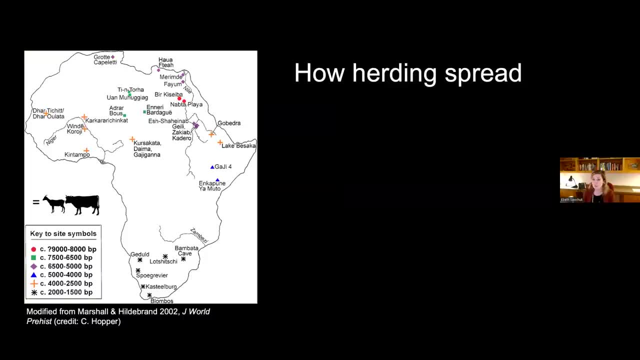 research we can start to see how humans were moving along with domesticated plants and animals, which is really interesting again when we're trying to get at those axes of human variation. So in brief, this is the Coles notes of food production in Africa. Food production first. 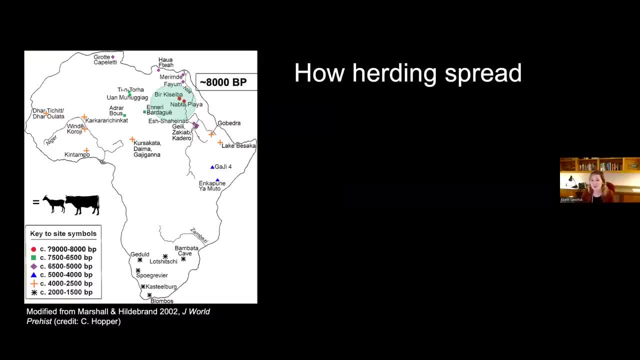 emerges in the Sahara about 8,000 years ago, during the African human period, when it was much wetter, there was lakes and rivers that dotted the so-called green Sahara. everything must come to an end eventually, so global climate change kick-started the end of the. 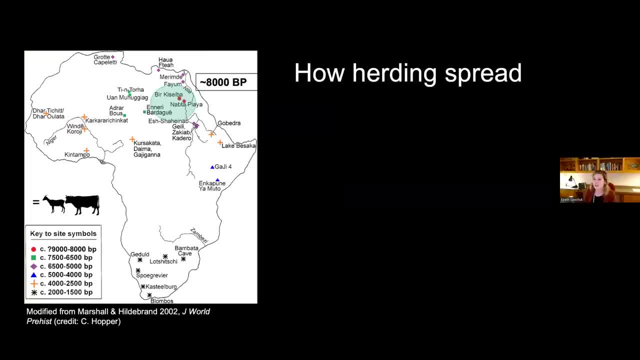 African human period about 6,000 years ago, and then livestock, and presumably also herders, spread west and south over the next several thousand years, showing up at the tip of South Africa about 2,000 years ago. So there's a few important things to take from this process. 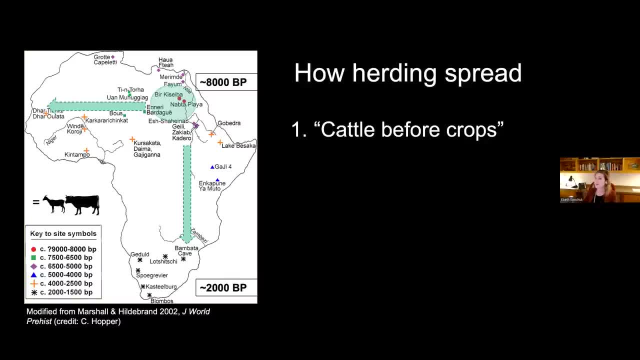 One. unlike in parts of Europe and Asia, cattle are spreading well before crops, so it's mobile pastoralism before farming, which makes sense again when we consider the ecology and the environment of many parts of dryland Eastern Africa, When it did spread. 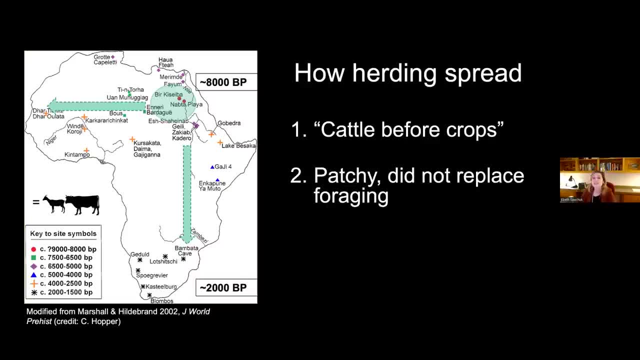 it was quite patchy, so food production did not replace pre-existing hunter-gatherers. in many parts We see actually a mosaic developing where hunting and gathering still continues up until the present day in some areas and herders kind of engage with these hunter-gatherers in different 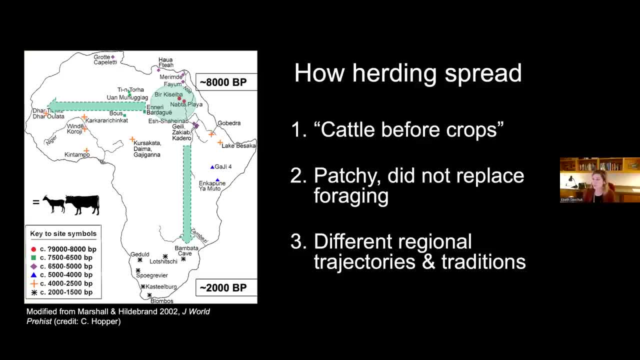 ways. And then also when herding does spread, we see different regional trajectories and traditions, so it's not like one wave of people that's spreading across the continent. It's actually a bunch of different origins for different species of plants and animals at different times, with 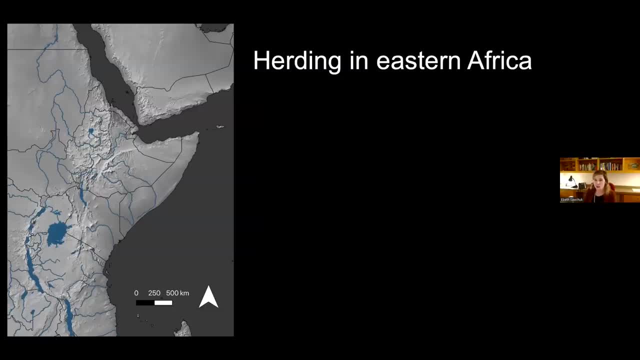 different outcomes. So when we look at Eastern Africa, which is where I work, this patchiness is very much the case. So as the Sahara dries out at the end of the African humid period, herders probably followed waterway south. We don't actually know the route and it's very difficult. 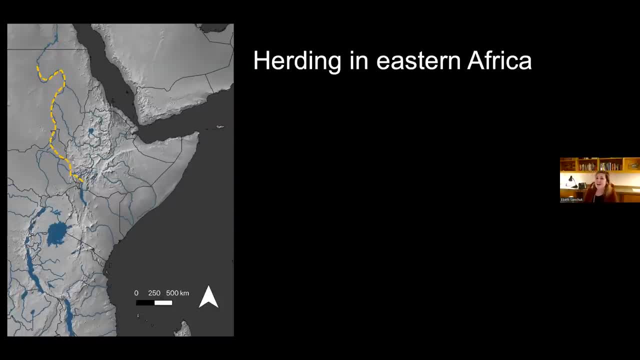 to do archaeological research in South Sudan right now, but they ended up in the Turkana basin, which is what we know, And then for about a thousand years we don't really see the movement of cattle, sheep and goat further south- A little bit of goats trickling down as well as some pottery. 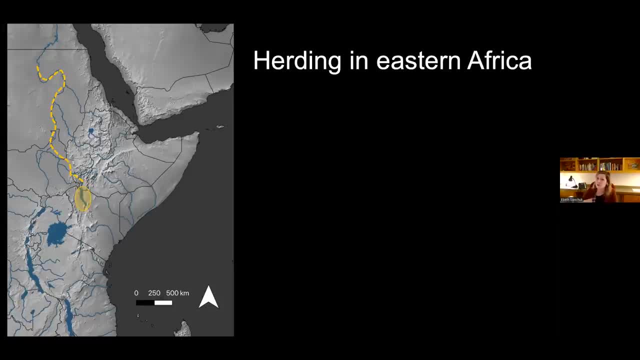 that I'll talk about. But for some reason herding didn't really spread for a while. maybe because of some zoological factors, maybe because of some disease vectors, We're not really sure. But by about 2,000 years ago herders have figured this out and it starts kind of this grand era of 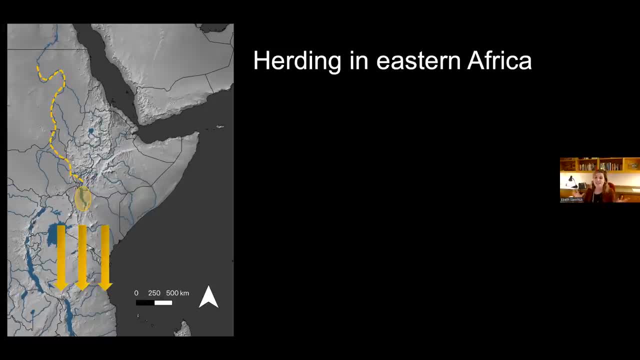 herding in Eastern Africa, called the Pastoral Neolithic, where some of the sites here have like 99 percent cows right. So people are very intensively herding at this point. So the part I find interesting in this story is right when herders get to the Turkana basin about 5,000 years. 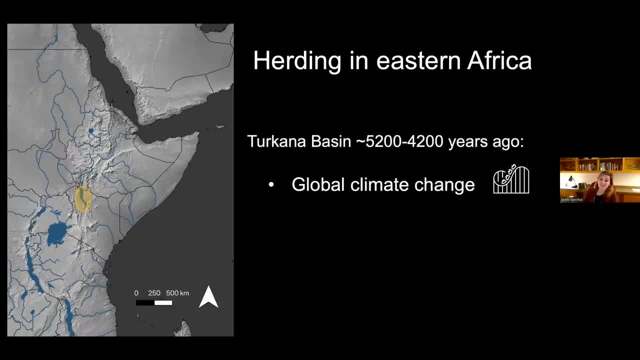 ago, because it's kind of a roller coaster of a period in African history. One: we've got global climate change happening. So the same things that are making the Sahara expand, the same factors of the African humid period ending, are also shrinking Lake Turkana by about 50 percent. We also see an 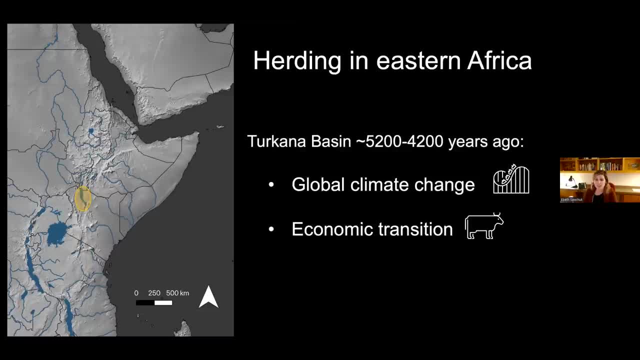 economic transition. So right around this time we have the first evidence of cattle, sheep and goats, and so we see herding starting to spread around the Turkana basin, although we're not quite sure the mechanism yet. And then, finally, with this environmental and economic change, we see massive 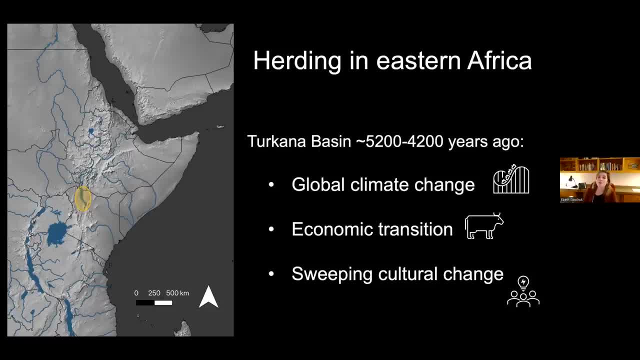 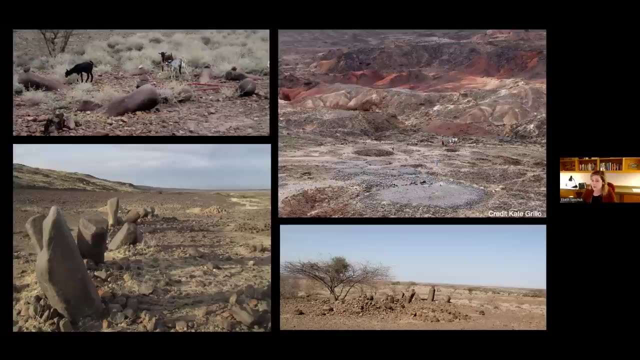 sweeping cultural change. So new types of pottery we see new types of stone tools and then, of course, the first monumental architecture in Sub-Saharan Africa. So these are the earliest megalithic sites that we know of so far in Sub-Saharan Africa, but they're around the Turkana. 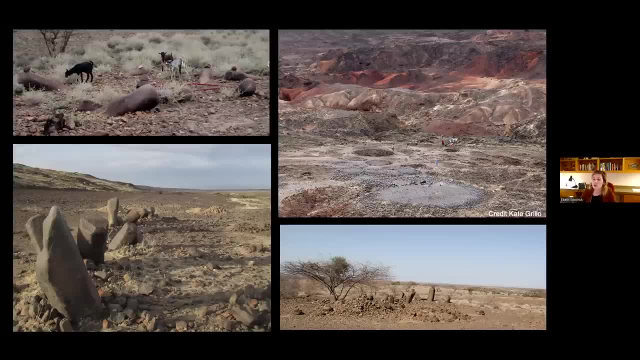 basin between about 5,200 and 4,000 years ago. And then finally, with this environmental and economic change, we see the first monumental architecture in Sub-Saharan Africa. but they're around the Turkana basin between about 5,200 and 4,000 years ago. They're called pillar sites or in the Turkana. 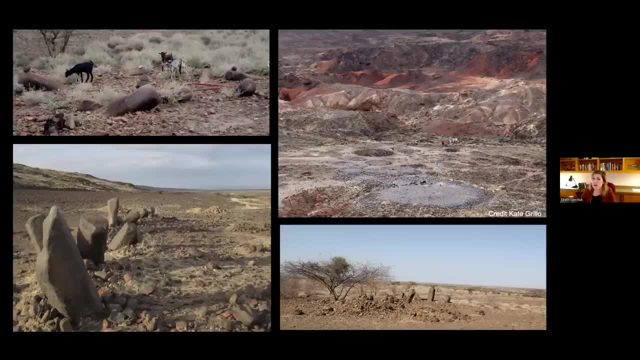 language, namuratanga. They're called pillar sites because they are these naturally occurring pillars of columnar basalt and sandstone that people would have quarried and then dragged up to two kilometers away to put into these stone platforms in arrangements of semicircular and 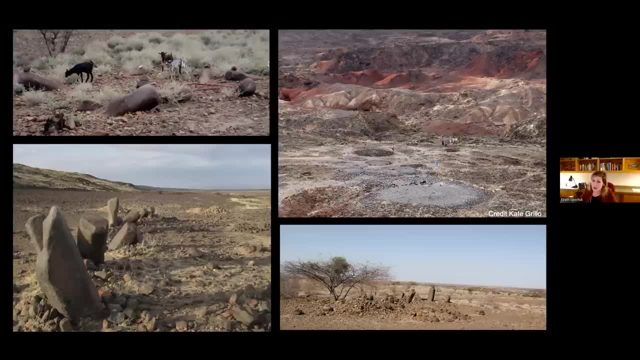 linear arrangements. They're really heavy- They weigh about 800 kilos each- and we have no evidence that people would have been using animals to transport these. So this is a really important thing to keep in mind. And then, finally, with this environmental and economic change, we see the 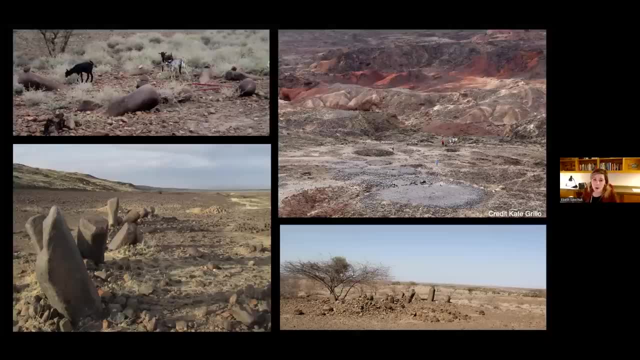 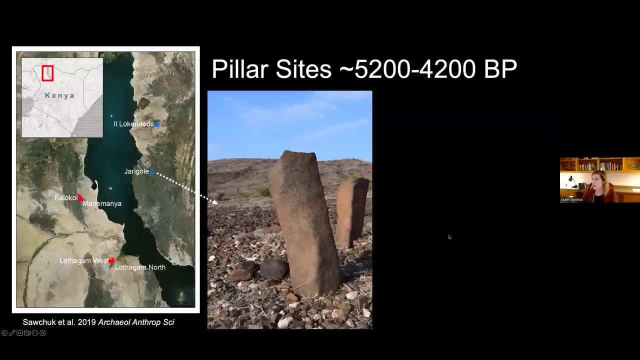 first monumental architecture in Sub-Saharan Africa. This is a huge effort on the part of small scale societies. So we have about six of these sites around the lake. There's at least one more, so there's seven, And although these are the first monumental architecture in Sub-Saharan Africa, 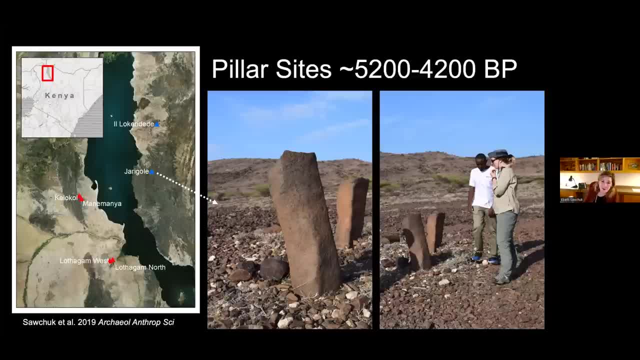 this is probably a good time to be honest with you that the scale of their monumentality is not perhaps what you would expect. So these are actually pretty difficult sites to find on the landscape unless you really know what you're looking for. And, as you'll see, all of the work that went into these sites is really underground. 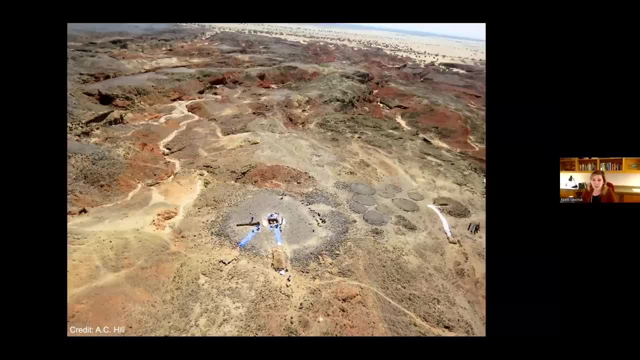 So this is a site that my team- the Later Prehistory of West Turkana project- has been working on for about 10 years now called Lofagham North. It's on the southwest side of the lake And you can see that it's a 30-meter diameter stone platform with a bunch of associated. 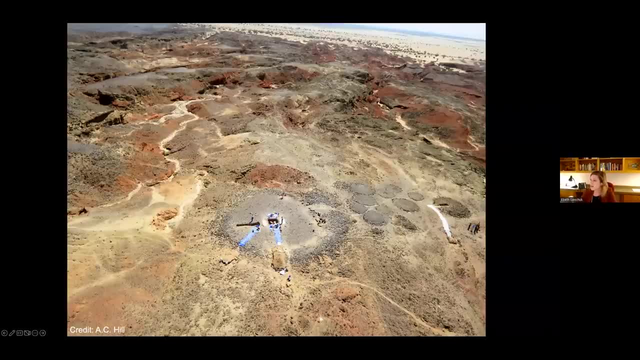 circles and cairns- And the line of pillars is right here, if you can see my cursor- And although these sites have been known since the 1970s, up until recently there had been extremely limited excavation, So it really wasn't clear what they were used for. 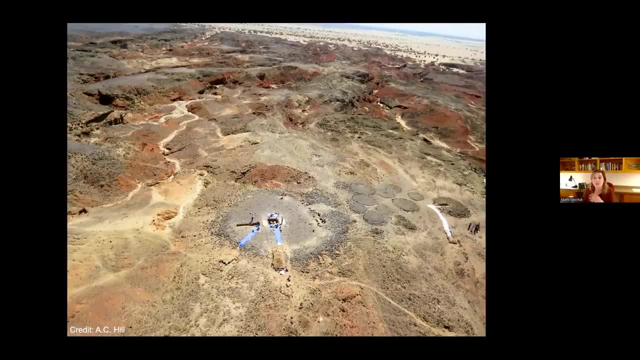 Our project has been excavating at several of these sites to try to understand how they fit into this story of the spread of herding into eastern Africa, And what we found has completely defied all expectations. So in the middle of this platform, here, this is a two-by-two-meter. 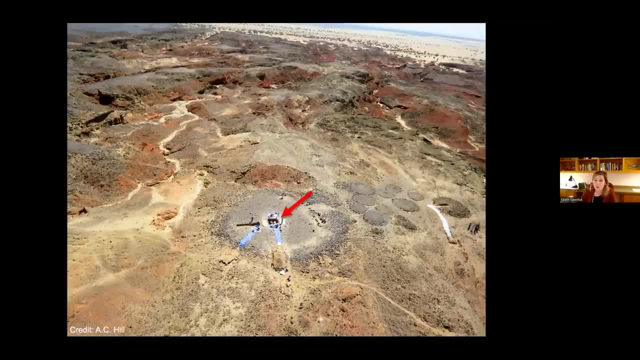 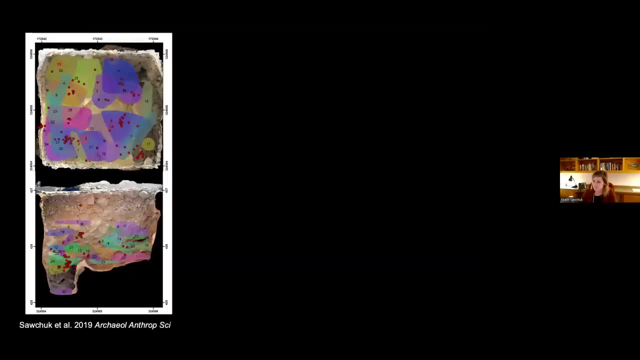 excavation unit that went down 1.7 meters. I'm like the red dot in the hole here. And then, when we look at that, a schematic of that two-by-two excavation unit, each of these ellipses represents a buried individual. So within this very small 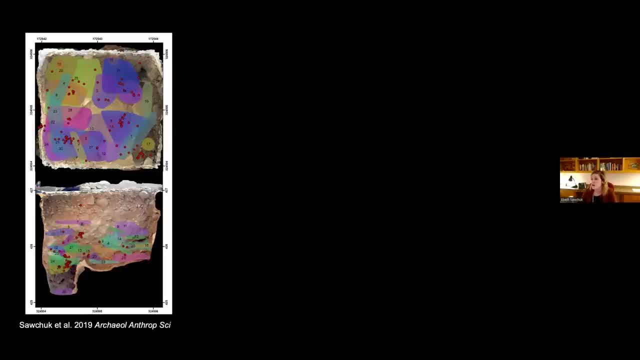 excavation trench. we excavated at least 30 individuals. All the red dots indicate stone beads that they were found with, And so this is an extremely dense cemetery of people buried over. based on the radiocarbon dates, we think a few hundred years, So that's quite enormous to 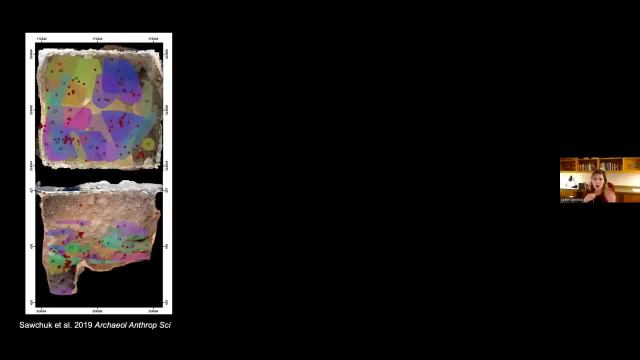 consider the effort that went into these cemeteries. The people buried are men and women, ranging in age from little little babies to very elderly individuals, And they're all in different body positions and orientations, and they're all in different places, And so we were able to maximize the number of people who 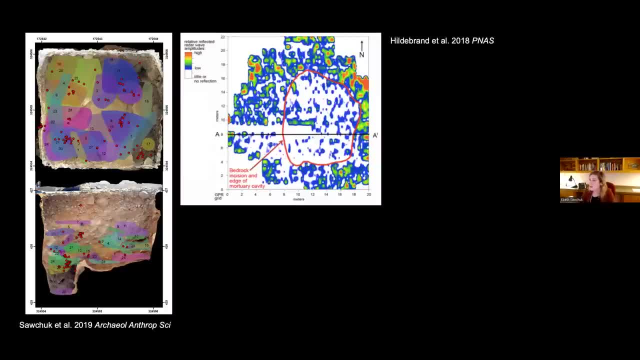 could fit into this central mortuary cavity. So another thing that we did was we looked at ground penetrating radar. This is all published in 2018.. And we're able to estimate the size of the mortuary cavity And then, based on the 30 individuals, from that two-by-two-meter. 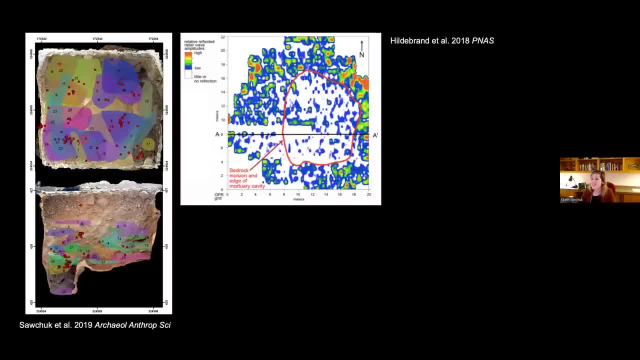 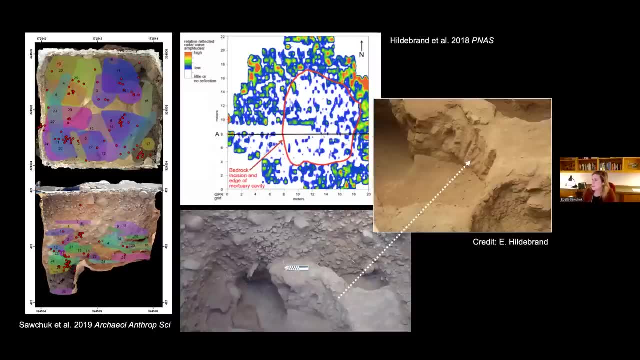 excavation unit. we estimate between 580 and 1,000 people are buried at this site And the deepest burials are actually dug into the soft sandstone bedrock at the bottom of this mortuary cavity. So this is kind of a picture of the main area of the site before iron reaches the area, But you can actually see the 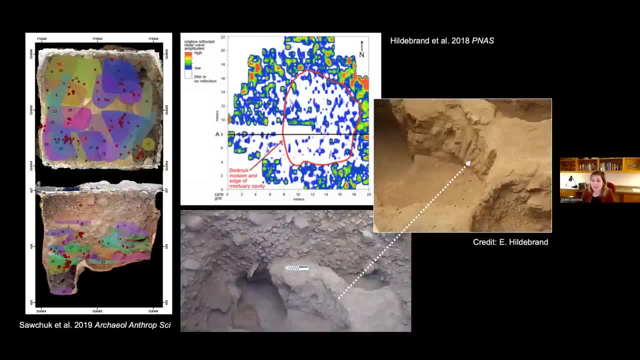 gouge marks that people would have dug out these pits probably with some kind of animal bone or horn. So the amount of effort at these sites is absolutely staggering. to consider that this big 700-meter cavity was dug and then, over many, many generations, people put in members of their family. 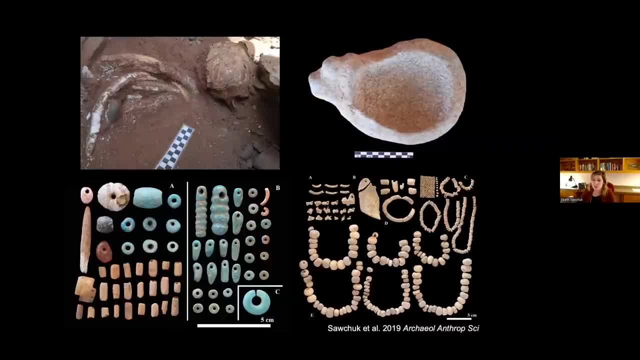 together in this amazing communal cemetery. I also found a bunch of different interesting material culture within this. So the person in the top left is an individual who's buried with 12 perforations of iron created hippo tusks. Hippos are terrifying, so that would have been quite the feat to assemble. 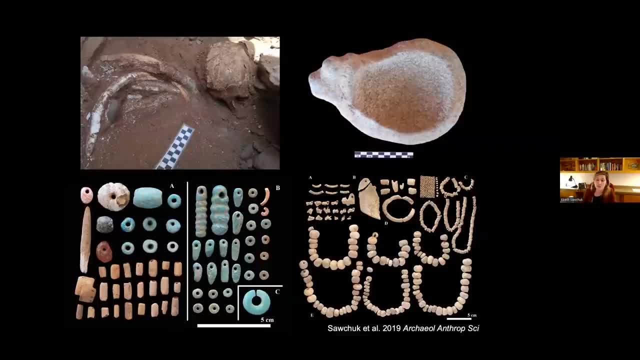 that Also, as I mentioned, lots and lots of people are buried with stone beads. It doesn't look like there's any accumulations of wealth with, you know, particular ages or sexes. I mean, almost everybody is buried with something, even the little little babies. We also found this. 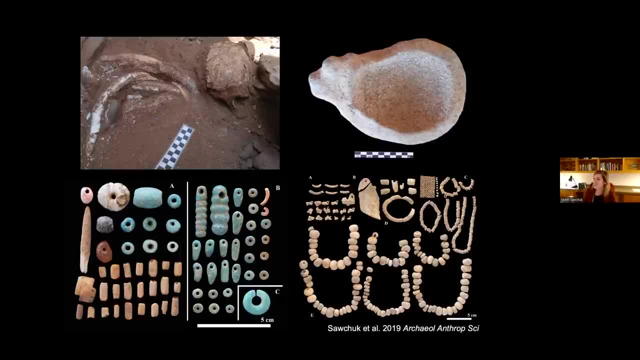 very interesting zoomorphic palette which, you know. there's some arguments within our team and otherwise, if this looks more like a cow, which is what I think it does, versus looks like a hippo. So that's ongoing. We don't find a ton of evidence of herding, but then again, these are mortuary. 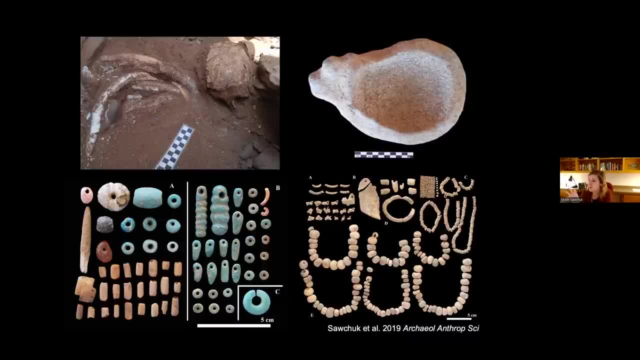 sites. And then there's one woman on the bottom right here. Those were all of the beads and other things that were buried with her. So she even had, like, a caned tooth bracelet of over 40 different caned teeth, which we're currently studying to determine if they're dogs or jackals. So just 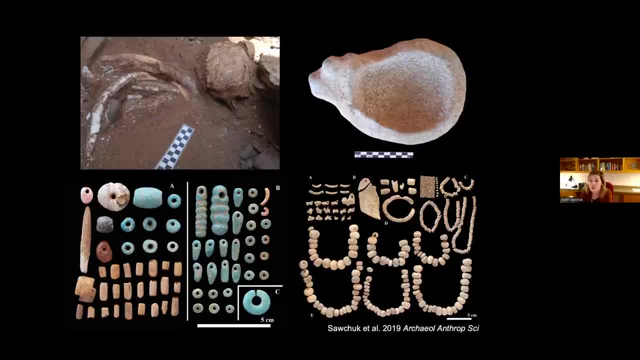 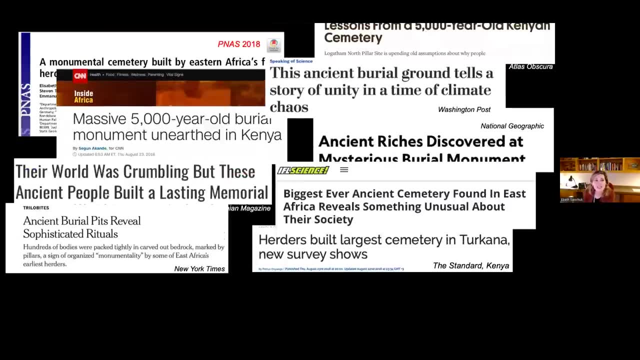 absolutely amazing amounts of material, culture and effort that went into these sites and went into individualization. So, as I mentioned, we published this paper in 2018, and we got lots and lots of cool feedback about this, because it's a really great story. It's a really interesting story that resonates. 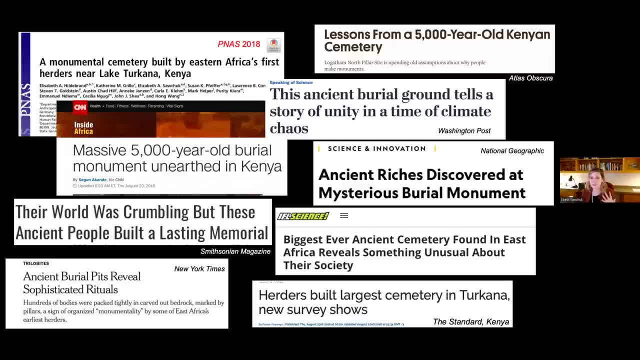 with a lot of people During this time of major environmental and economic change. instead of people turning against one another- you know incoming herders, fisher foragers who lived around the lake- it seems like people put their energy into coming together and building these. 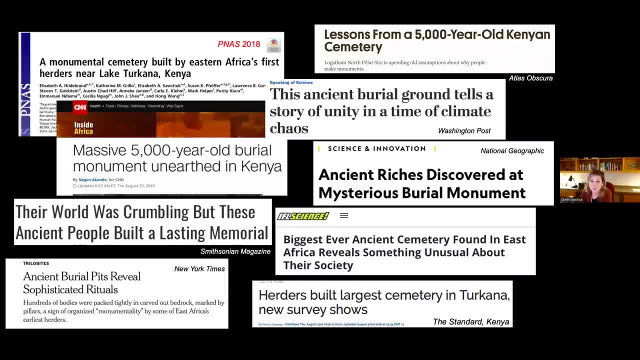 monuments to their communities. But really, this is just the beginning of the story, because there's so much more we can learn about these things And I think it's a really interesting story And I think there's a lot to learn from these people, especially because, in addition to the amazing, 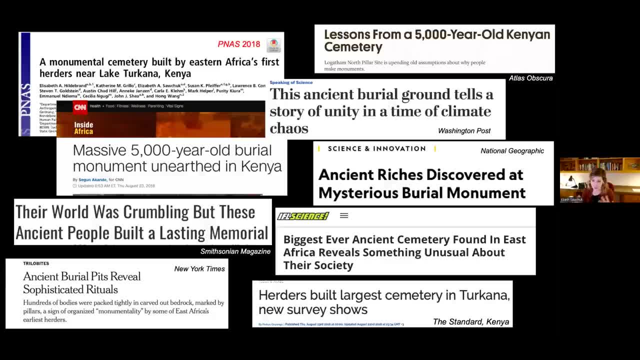 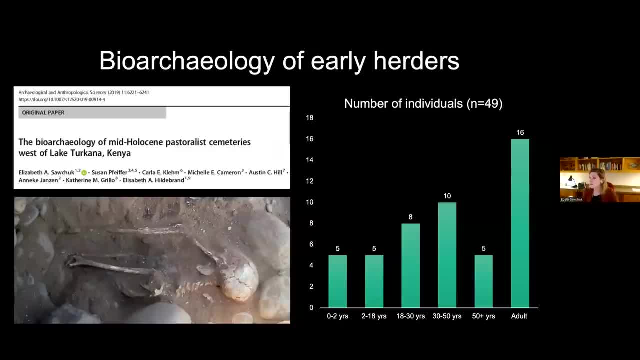 archeological sites they created and left for us. we also have the remains of the people themselves who are buried inside. So this is really where the bioarchaeology comes into the conversation. You know, we can look at the individuals who are buried at this site and other sites. So this is a paper about three pillar sites. 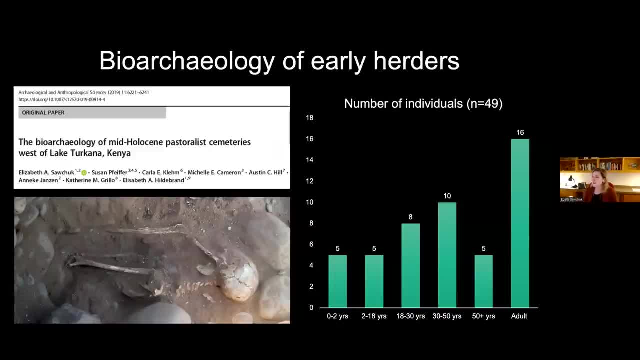 on the west side of the lake And you can see the cross-section here is really again full age ranges, both biological sexes estimated, And so you can really try to understand why people are buried at every site. And so we're going to go over the whole history of the lake and then we're 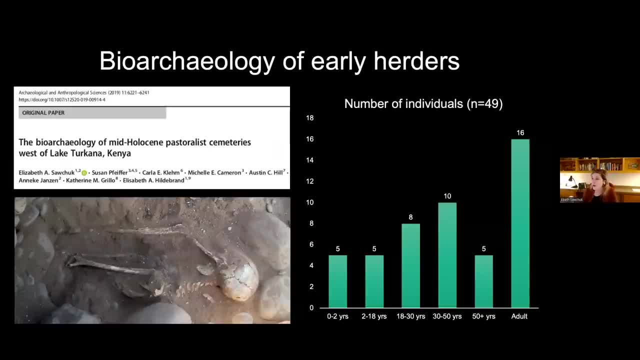 going to cover some of the most important sites that are buried in the lake And then we're going to to understand who these people are and what their community looked like demographically. We can also ask questions, specific and test hypotheses about how herding spread. So this: 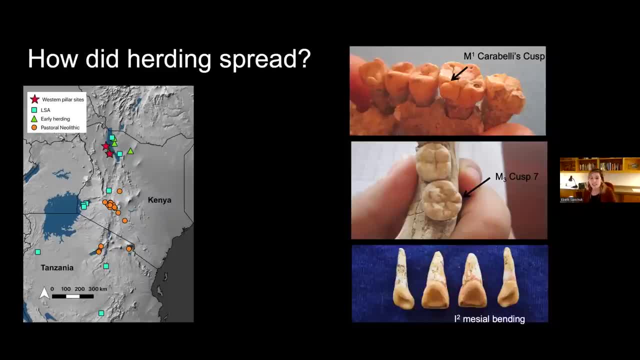 is a little bit of work from my dissertation. I was really interested in testing the hypothesis that these people who built the pillar sites, these early herders presumptively- and there's some good indications that they were engaged in herding, So we do find good. caprine remains at. 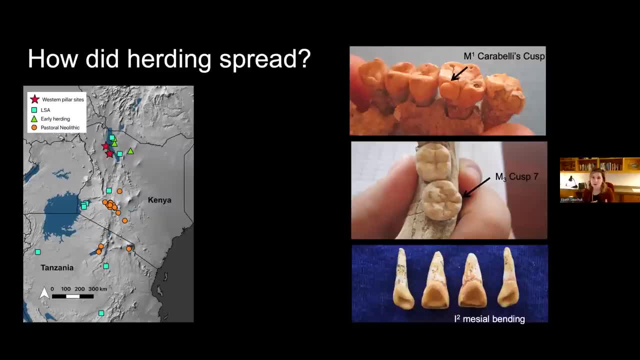 these sites And of course there's also connections between the material culture and the pottery and derrit pottery, between these pillar sites and then a habitation site called Dongodian, on the eastern side of the lake, which has cow bones in it. So we're assuming that these 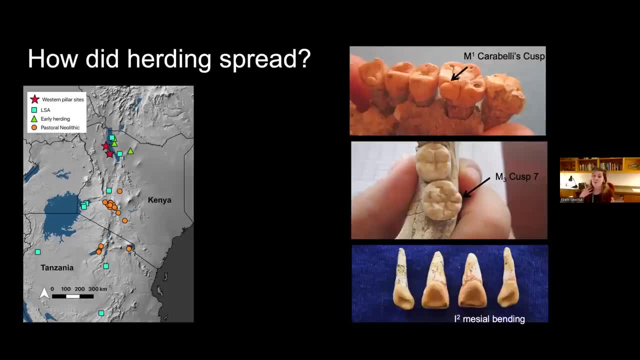 people based on timing, based on context, are probably the first herders in eastern Africa. So what I did is I wanted to compare these individuals to the later Stone Age fisher foragers in Turkana before herding arrived, and then those pastoral Neolithic herders in the 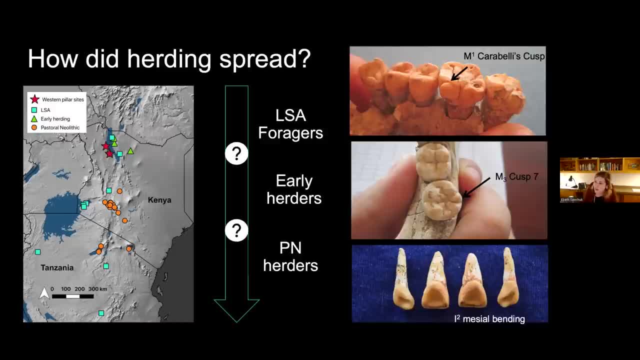 south-central Rift Valley afterwards to see if there's any big breaks in there. that would indicate that a new group of herders would be able to come in and herder. So I wanted to compare these people to see if there's any big breaks in there that would indicate that a new group came in at any one. 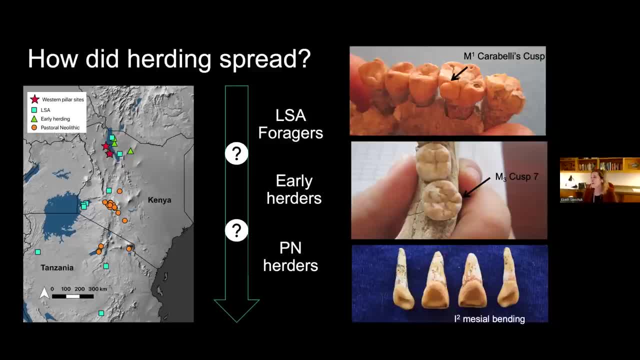 time. This was before we had ancient DNA in Africa, and also Turkana has been very resistant to yielding DNA because it's very hot, And so I used dental morphology to do this. You're all biological anthropologists, so you know that dental morphology is a reasonable proxy for. 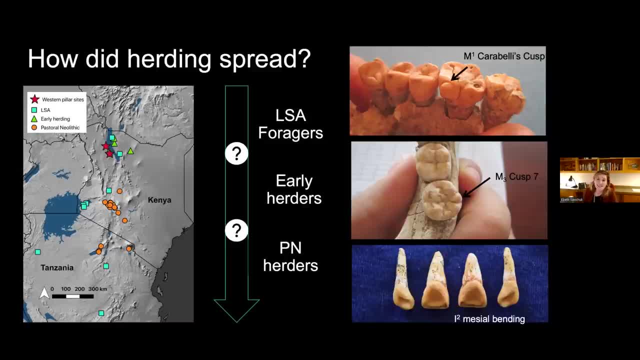 biological affiliation If you don't have DNA. everyone has teeth. They all form at pretty regular times. The bumpiness and size of our teeth are more likely to be related to the bumpiness and size of our family's teeth, versus groups who are more likely to have teeth. So I wanted to 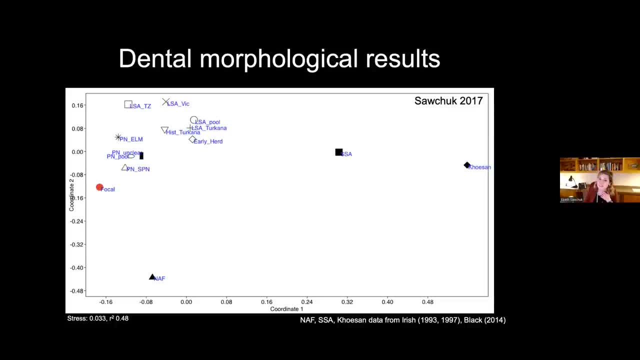 compare these people to see if there's any big breaks in there that would indicate that a new group or not related to, And so this was the hypothesis I was testing To show you some quick data. essentially all of these ancient Eastern Africans- here's the pillar sites. they all glom together. 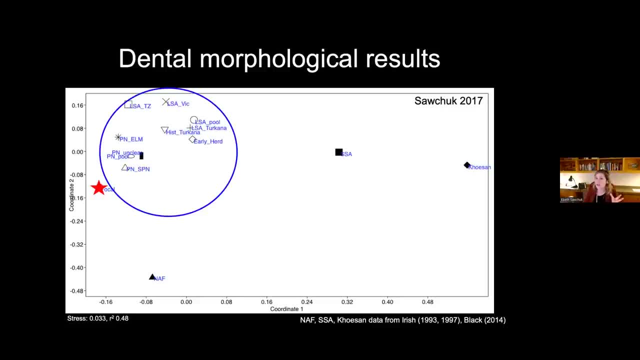 So there's really no statistically significant differences in dental non-metric traits. that would indicate that we have a big break in continuity with the spread of herding. Interestingly though, all of these ancient Eastern Africans are quite different than contemporary sub-Saharan Africans and Southern Africans, but not that different from Northern Africans, which I guess. 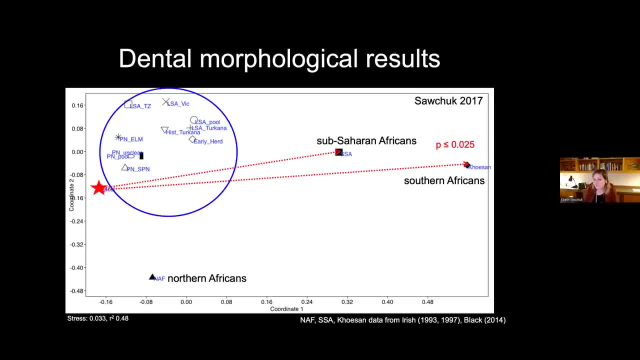 makes sense if you consider that. So I wanted to compare these people to see if there's any big difference in the way that we consider the direction that livestock is moving. So really, what does this all mean if we want to understand population history? 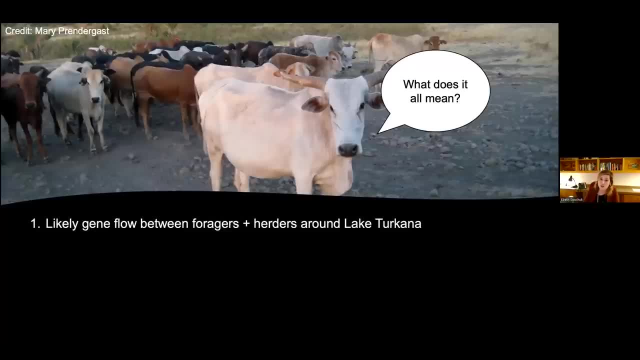 One that we're seeing likely gene flow between foragers and herders around Lake Turkana, which kind of makes sense If the lake is shrinking and fisher foragers who've been living there for thousands of years are losing access to some of their fishing resources and, at the same time, 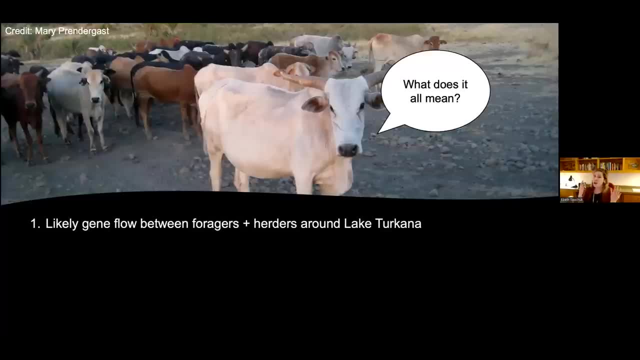 you have a new economic strategy coming in, you have potentially meeting between people and the birth of a new society which is the future of the lake. So I wanted to compare these people to the origins of East African pastoralism And that also kind of raises some questions about the 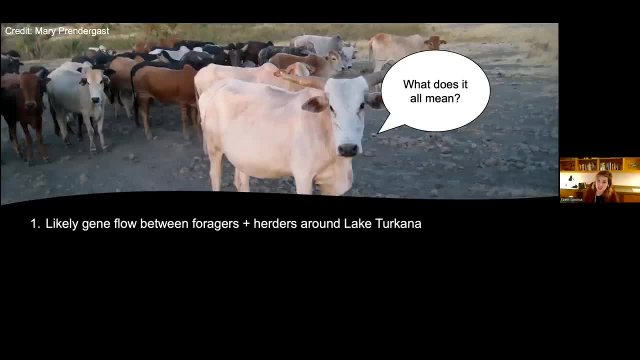 pillar sites because, although we can never truly know the motivations for why people created these sites, they were obviously a huge sink of labor And it occurs to me- and I've published before- that one of the biggest displays of unity that you can have between two groups meeting one another. 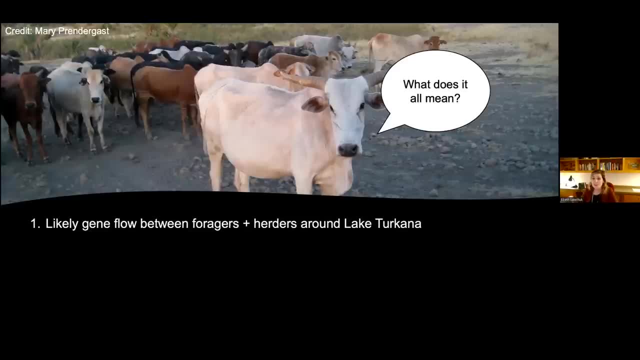 and saying that you're the same is burying your dead together. So perhaps this is part of the motivation for creating these sites and creating these permanent fixtures on the landscape that people could start to rally around. We also know from this data that early herders around Lake Turkana probably help transmit herding. 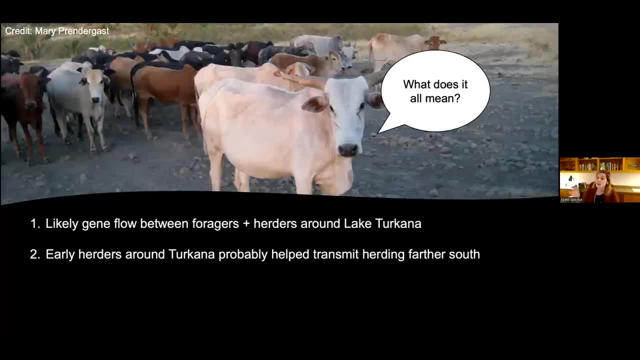 further south, since we don't see any major dental differences between the early herders and then the pastoral Neolithic individuals. It suggests to us that culturally distinct people might be biologically related. when we get into the pastoral Neolithic and we start to see a lot of different. 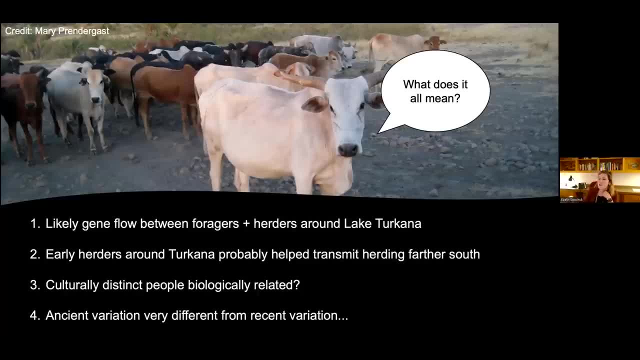 herding cultures, kind of working at the same time. And then, of course, the thing that no one likes to hear is that ancient variation might be very different from recent variation, And so this is part of the rub with ancient DNA: We cannot extrapolate more ancient patterns from living. 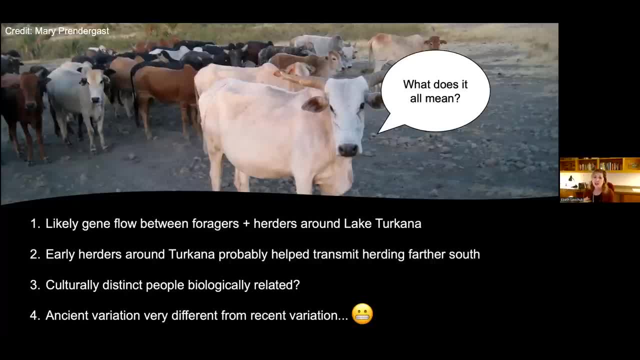 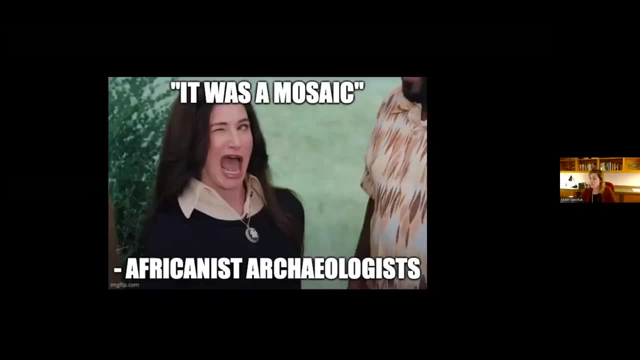 people because of that fussiness of the past 5,000 years In order to look at more ancient patterns of variation. unfortunately, we truly do need to study ancient human remains. So what we take from all of this is kind of a trope in African archaeology, which was that it was a mosaic. 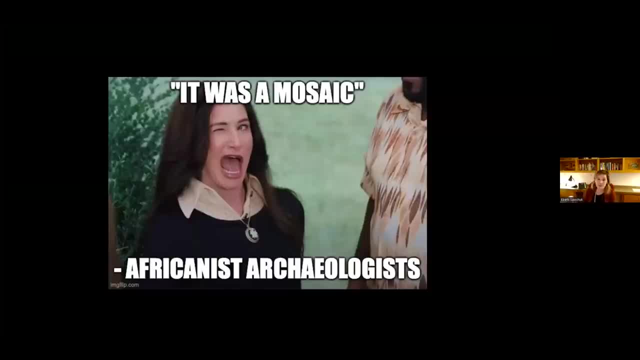 Definitely there's many people with different cultural and probably biological identities who are coming together and creating these complex societies And these complex patterns that we see in the African archaeological record. but as a millennial, I will say again with another meme, that's not very interesting to say that it's. 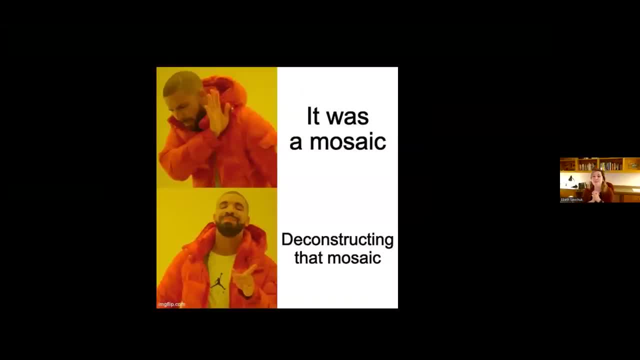 a mosaic. Of course, now we want to start picking apart this mosaic and understanding what the human behavior is under this pattern, the biological patterns that we're looking at. So this adds a lot of different questions and the kind of things that my team and I are working on right now. I 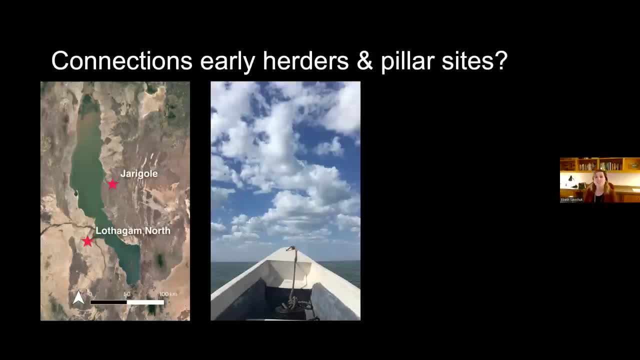 don't have time to get into a lot of them, but maybe a little teaser of some of the projects that we're currently working on. One is trying to understand how people at different pillar sites were related, So it's always struck me as interesting that the two earliest pillar sites, right at the beginning, 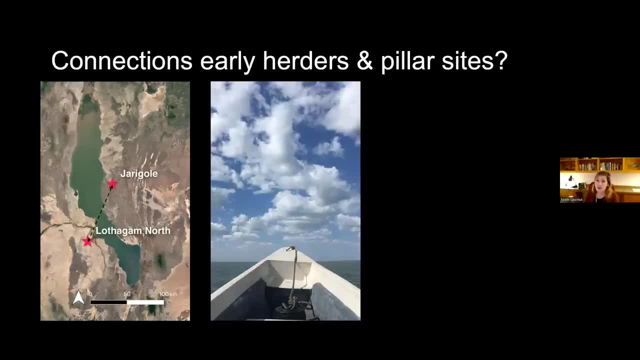 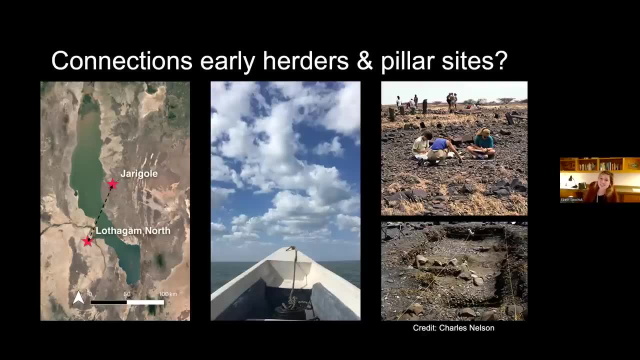 of that period, when we find cows are 300 kilometers apart, or 150 kilometers across a hippo infested, very terrifying lake that I've made the journey myself, And so the kind of question is: you know, are these the same people, Is this one culture, Or are these different? 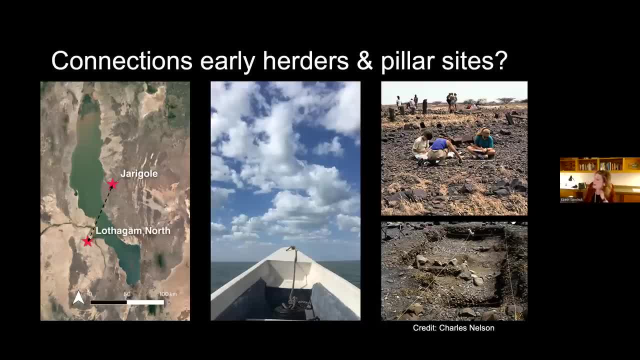 expressions of monumentality around the lake. You know it's a bit of a copycat situation And one of the things that's always been interesting is that the only site to be excavated previously was on the east side of the lake, called Jarigole. It was excavated by the Kubi. 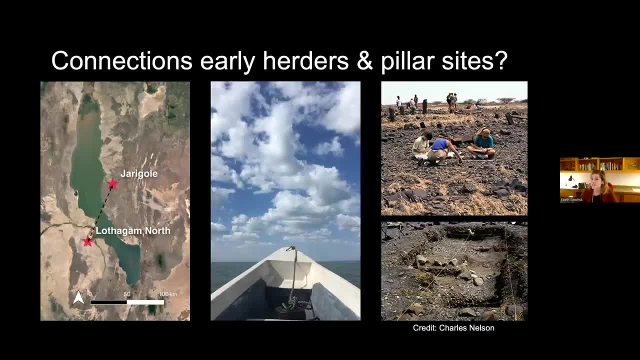 Fora Field School for over 10 years, between 1985 and 1995.. And essentially what they found was something completely different than that big mortuary cavity we found at Lothicum North. Instead of finding primary burials, they found tons of isolated human remains, kind of mixed into. 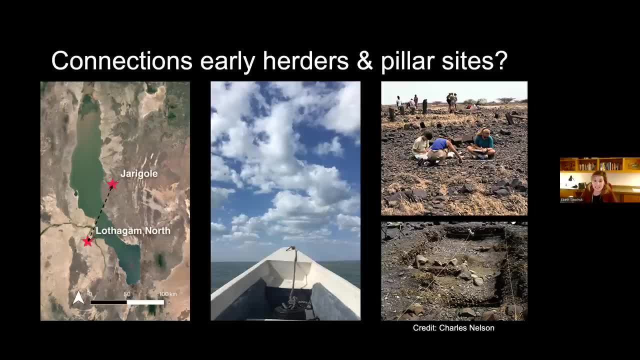 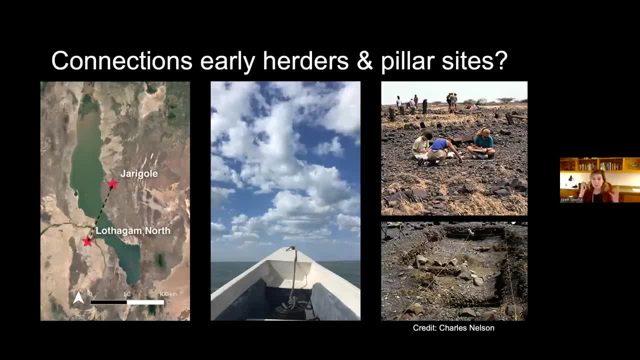 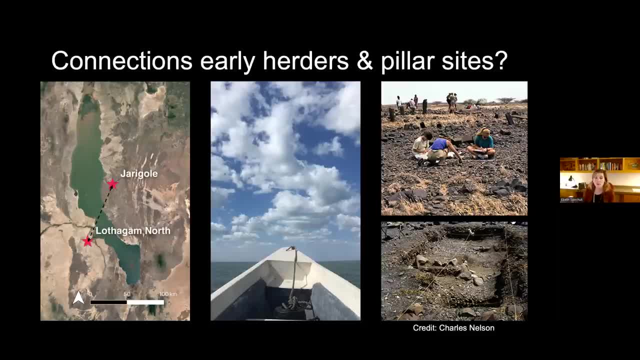 they were constructed completely differently because that could suggest two different groups kind of doing the overall same thing but with slightly different intentions, And that would be really interesting for understanding that mosaic. The problem is because it was a field school and for other reasons, the dig had to stop. They didn't dig very deep, they only dig about 50. 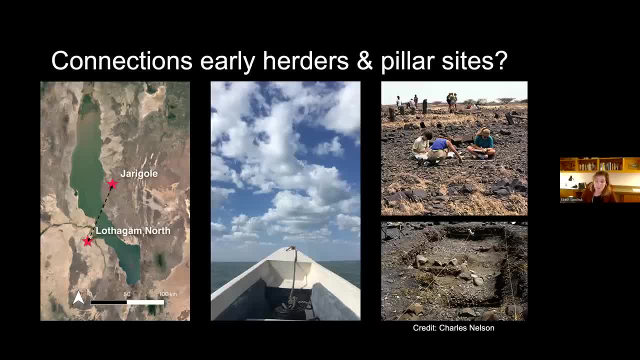 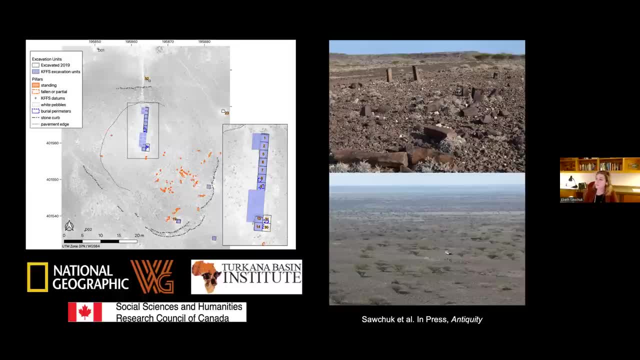 organized a team to go back to Gerogole, which happily had not been disturbed because it's in a national park. So this is from our 2019 excavation and should be out next month in one of your UK journals- antiquity. But essentially we refound the original Kubi Fora field school trench and we deepened part of it. 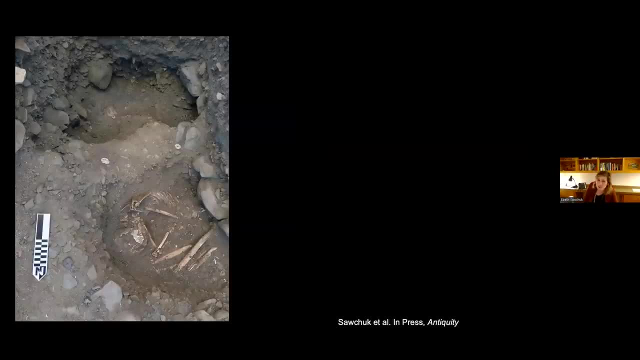 We also dug a new trench, And, in fact, what we found is that in some cases, they've missed the skeletons by about 10 centimeters, And so, in fact, we're looking at exactly the same construction between these two contemporaneously built pillar sites, with the pits at the bottom and the mostly. 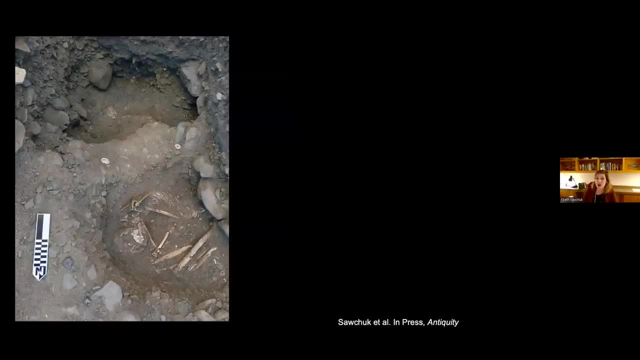 primary burials, And so that's really interesting to consider how people were moving around the lake And also the fact that these two sites are built at around the same time but finished hundreds of years later, and really understanding the continuity of this new culture developing around. 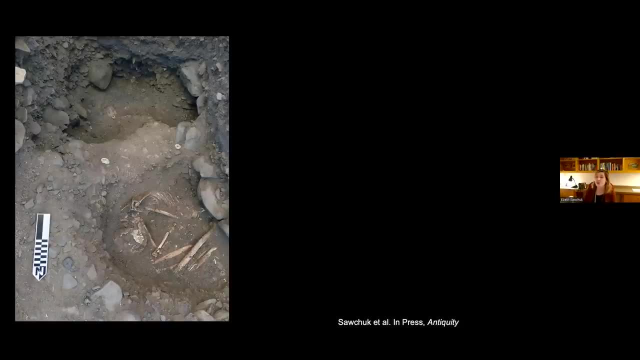 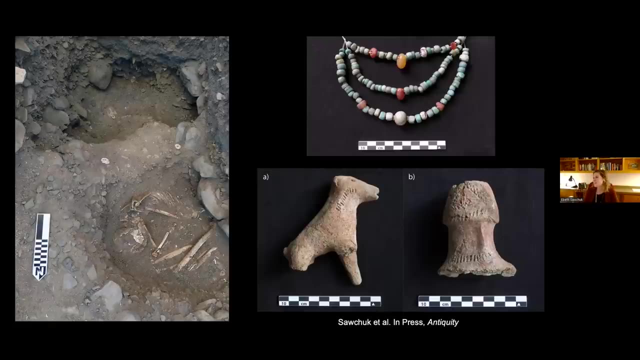 the lake and how people are moving and kind of sharing these cultural practices. We also found some other kind of cool stuff that kind of you know, enhances our understanding of culture at this time. So again, lots of stone beads here. This is an artistic reconstruction. we did not find this necklace. 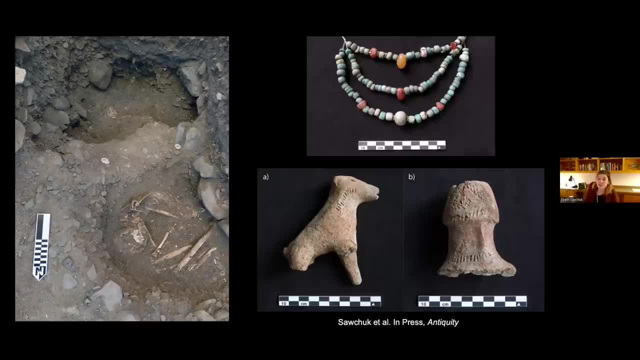 strung, But it was all around the neck of a woman who was about my age, died in her 30s. And then we also found some amazing figurines which we don't really find on the west side of the lake. Figure A: here is the debate if this is a topi or a dog, So weigh in in the comments afterwards. And then 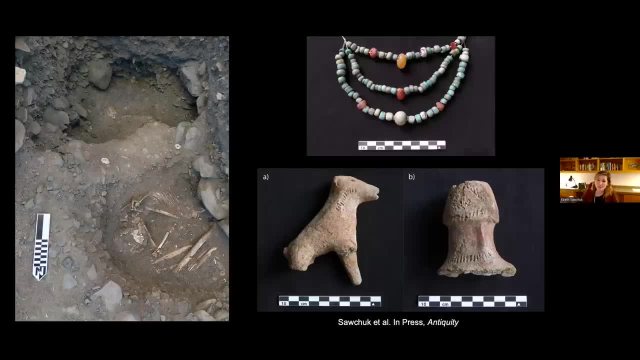 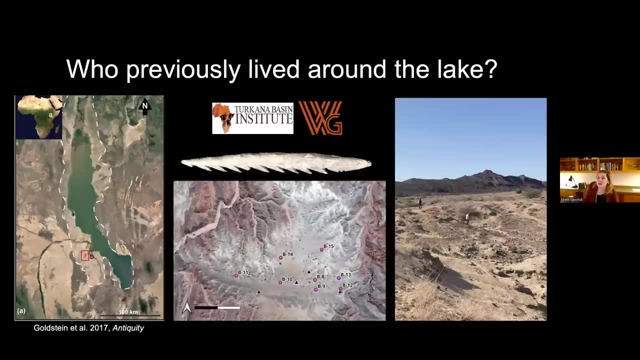 also, which I'm very proud of, the first phallic bottlehead of the pastoral Neolithic. So look for this stuff in antiquity pretty soon. Other things we're thinking about: who previously lived around the lake. So Turkana was not uninhabited before herding came, of course. 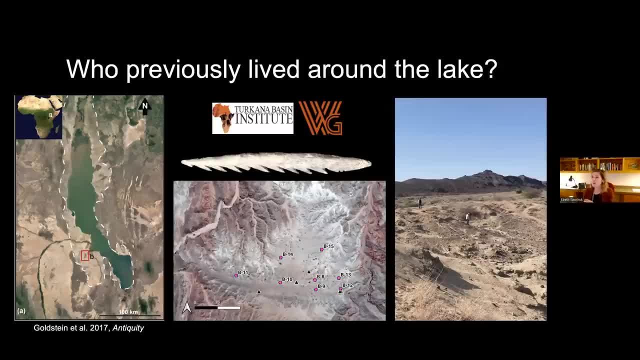 And of course, you know that if you've been following Mark Talar's work in your department. there was thousands of years of complex fisher forager societies around the lake, And so this is another kind of avenue that we're trying to understand. If you want to know what that mosaic 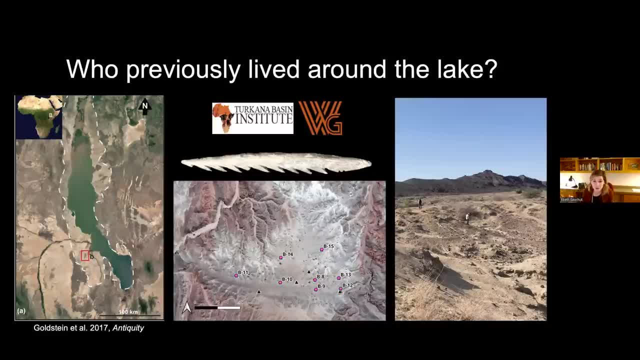 looks like when two different groups meet. we'd also like to know who was living around the lake beforehand and what aspects of their culture then made their way into this culture. And we know at least some, because evidence that we find around the lake from habitation sites are really just the one. 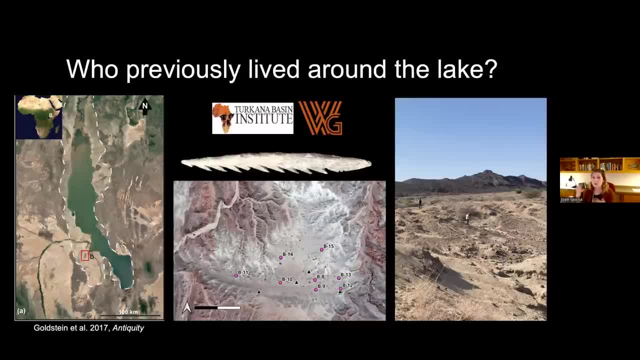 And then that. then Mimi Nagohana suggests this as a mixed economy of fishing and herding, So there's parts of this that are really getting folded into it. So again, seven kilometres away from Lothacum north, that pillars are just I told you about, there's actually one of the oldest fishing. 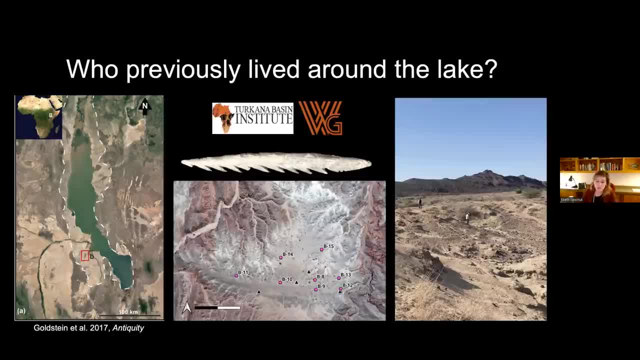 foraging sites in eastern Africa done called the Lothacum harpoon site. We're not suggesting calling it Lothacum locon, because there's many of the harpoon sites and locon is the name for it locally. We've been excavating there since 2017.. 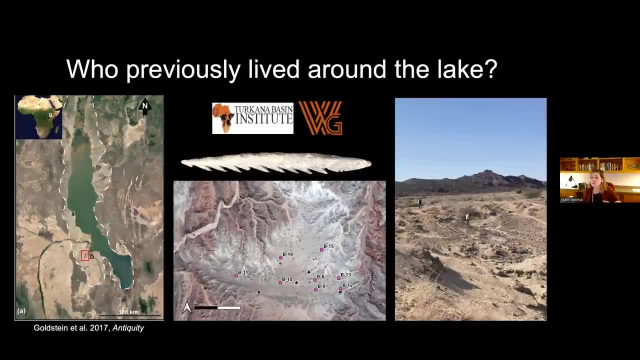 years ago, Lake Turkana was much bigger and Lothican was a peninsula that kind of jutted into it, So it's a really nice fishing spot. One thing that we've been realizing over the past several years is that erosion has hit this site really, really badly, And so individuals 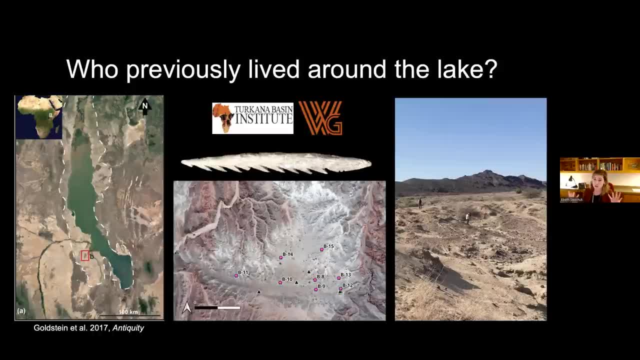 are actually kind of eroding onto the surface, which was also the case when the site was first excavated in the 1960s, but it's become a little bit more dire in recent years. So we've been doing some salvage archaeology and then also really understanding again what the occupation history. 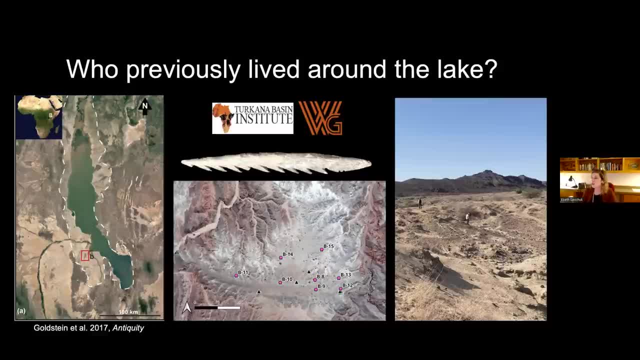 of the site is to try to put the human remains in context with the archaeology. So the map in the middle there is actually the number of individuals that we excavated this past season in 2022.. And then on the right is an image of what the site looks like today, Basically. 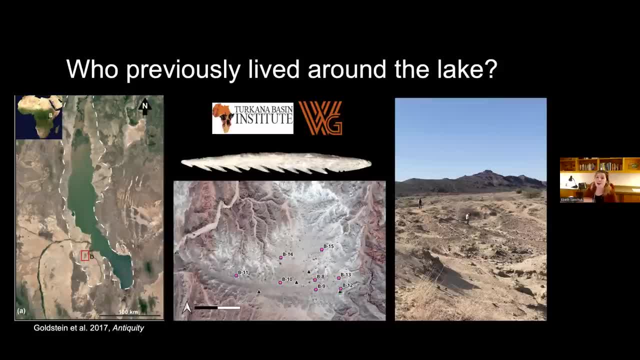 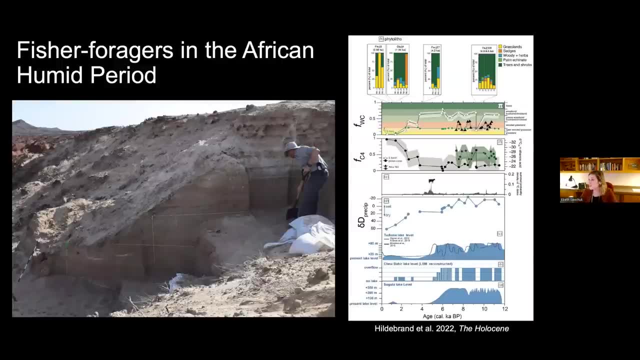 we walk around this giant, 100,000 meter squared site looking for evidence of people coming up. We've also done a lot of work with the dating at this site, And so not only do we have some direct dates on human remains now, which we will be sharing very soon, 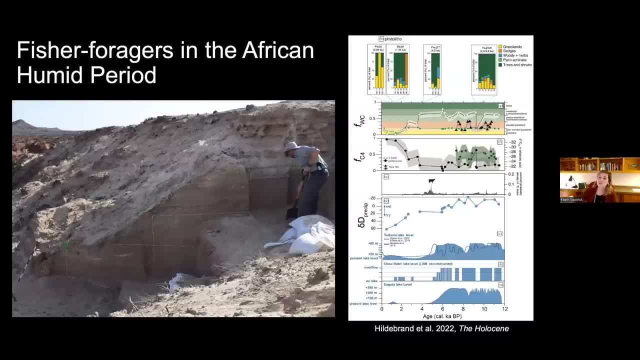 but we've also done a lot of geoarchaeology work to try to understand what the lake is doing. And what we found is, although the African humid period, the lake was higher than it was in the mid Holocene when herding came into the area. 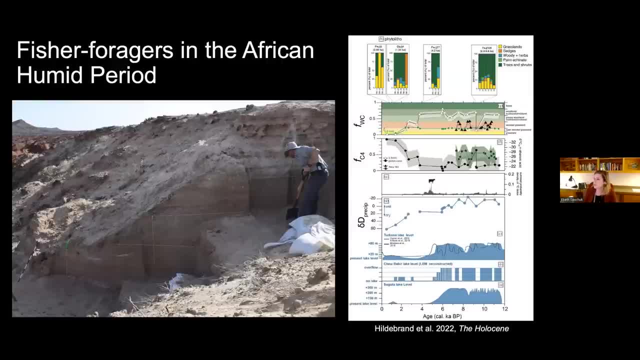 it was far from static. So this is a paper that's just been published in the Holocene recently by our team. We can actually see, based on paleoenvironmental proxies, that there was a fairly big dip in lake levels around 8,200 years ago, So 3,000 years before herding comes into. 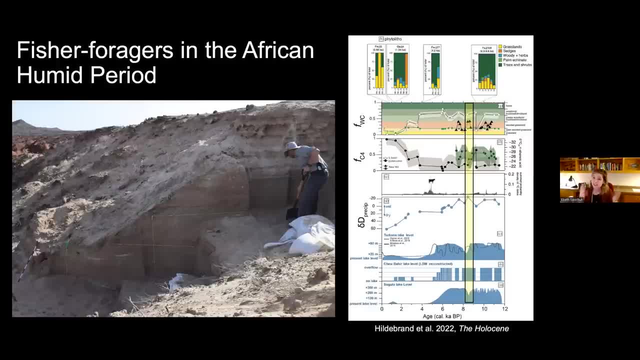 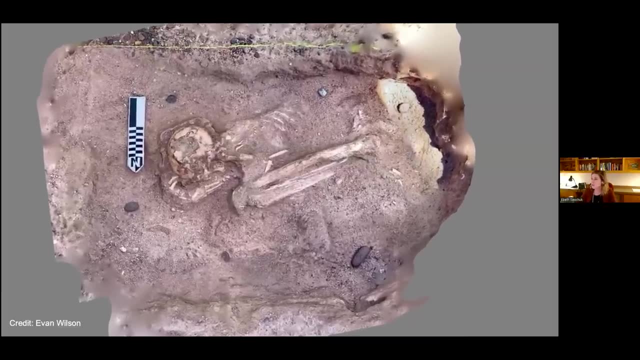 this area, And that also really helps us think about how existing fisher foragers may have already had experience With climate change and how this may have structured their patterns when the lake started to drop again. I also just want to show you a pretty photogrammetry image that was generated by Evan Wilson from 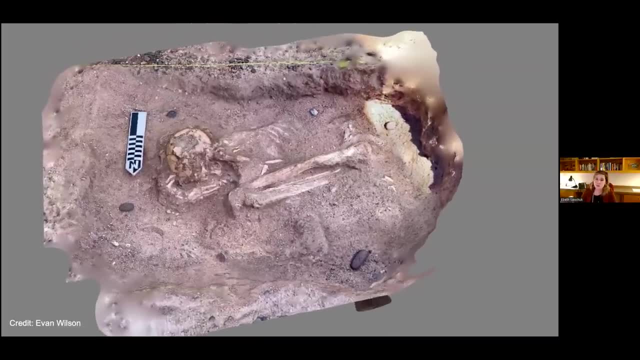 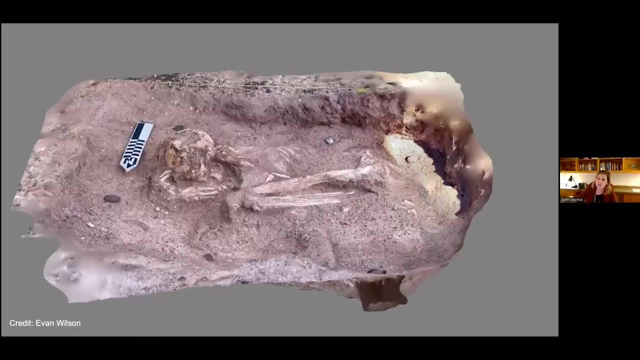 this 2022 field season. So these are the individuals that we're finding at Lothicum Locombe. This individual was just peeking up, based on the side of the cranium. There you can actually see where the damage is. It was on the surface. The human remains from the site are not. 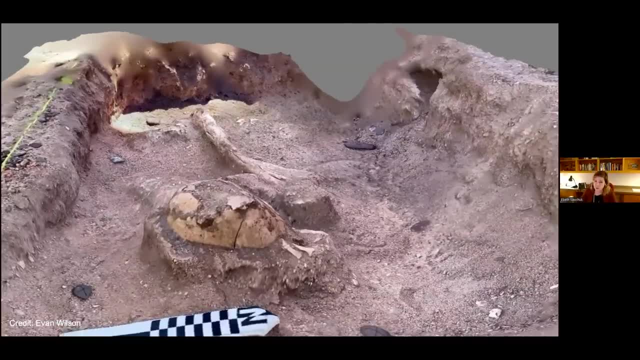 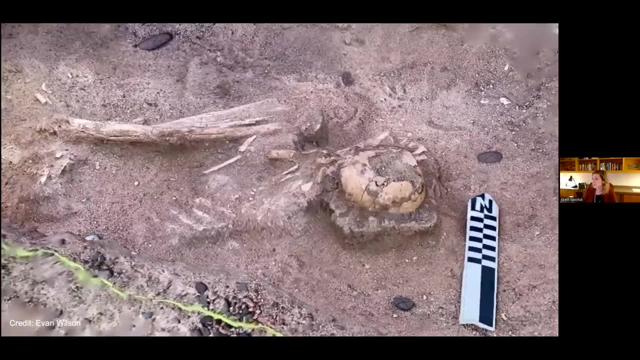 super well preserved, but they're still well enough preserved. That gives us a really great insight on what populations looked like about 10,000 years ago living around Lake Turkana. So this is really interesting to consider And this is fun stuff you can do with your iPhone in the 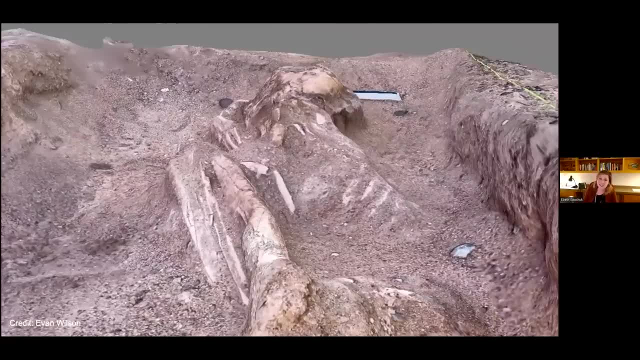 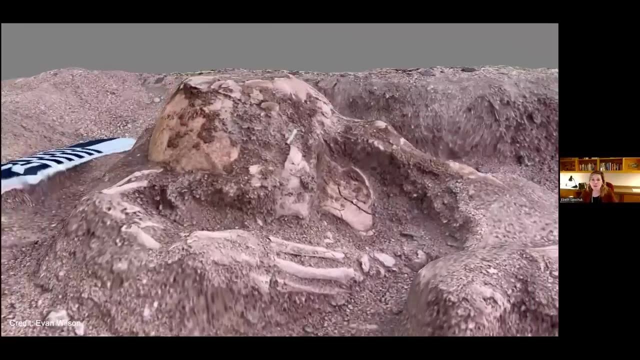 field now. So it's fun to excavate this site now, in 2022, because we have a lot of things that were not available to researchers who were there in the 1960s. There are a few other things that we've been considering again. So how did diet and mobility patterns change with the spread of? 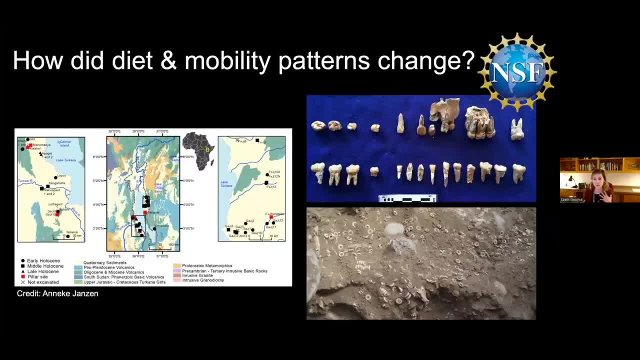 herding. So again, how mobile are these mobile herders? And, as a bioarchaeologist, one thing I think about is the logistics of these giant cemetery sites. So if we presume that people are living in small bands of herders and they're coming together when someone dies to come to these, 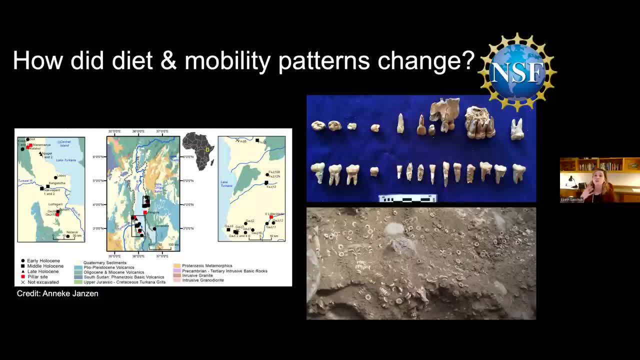 cemeteries and maybe this is a time to exchange information, to strengthen relationships, those kind of things. So how does the word get out? when someone dies, Does the person go into the nearest pillar site? Do they go into their hometown pillar site? We see both primary and secondary. 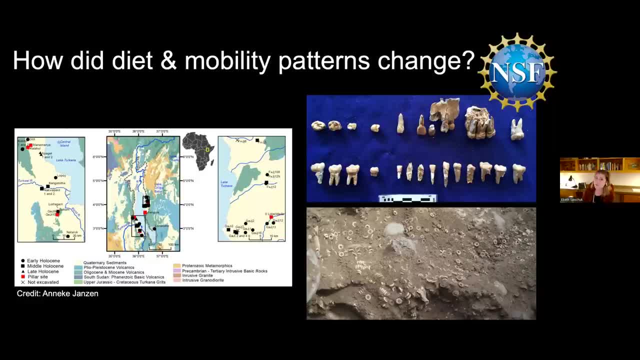 burials in these sites. So the question is: why are some people primarily buried in these sites? Why are some people primary and some people secondary? There's lots of questions, and getting at these questions is really going to require understanding, mobility, And so one of the 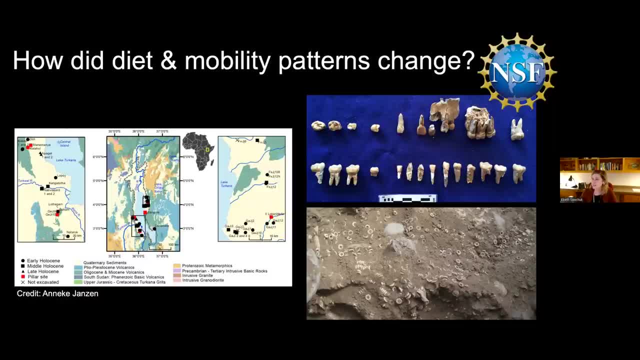 projects that we're currently doing- it's funded by the National Science Foundation here in the States- is looking at the strontium signatures of both the human remains through the teeth as well as the thousands of ostrich eggshell beads we find at these pillar sites, to try to get a 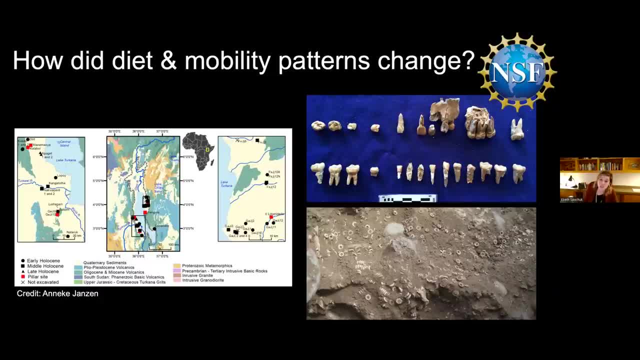 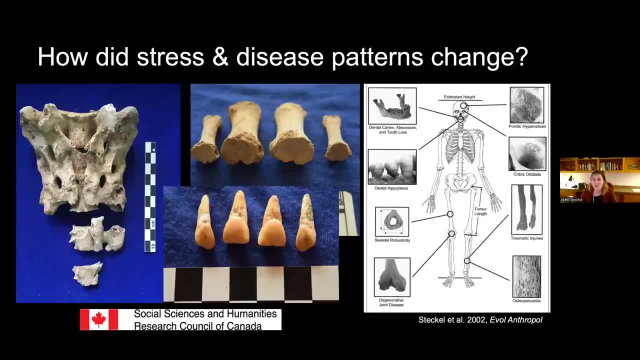 better understanding of how people are moving around that basin and also how their diet is changing at this time. I'm also interested particularly in stress and disease. There's lots and lots of bioarchaeological literature about food producers and how usually the adoption. 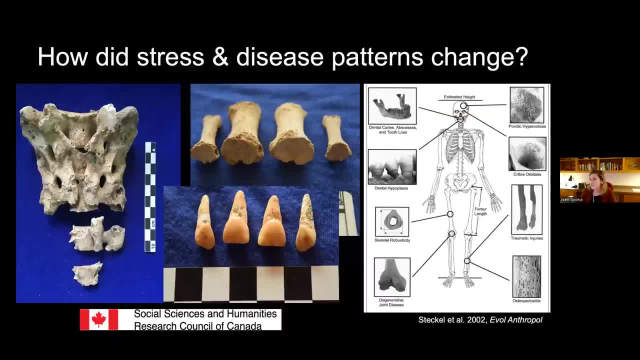 of food production makes people less healthy, but a lot of that is predicated on early farming in sedentary societies And we don't actually really have a good sense of what that looks like. that transition looks like bioculturally when people don't settle down and farm, And part of that is 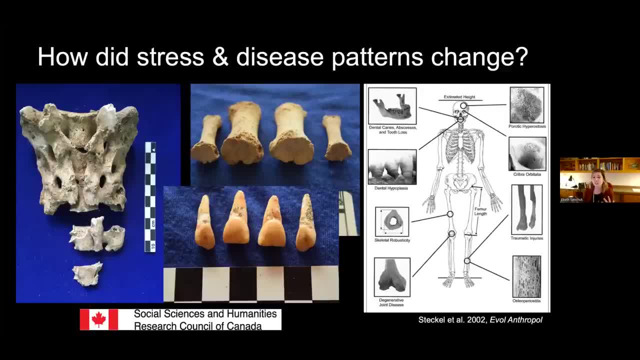 because there's very few skeletal collections that document a local transition from fishing foraging to mobile pastoralism And, of course, Turkana is one of these places that we have that. So we're really trying to understand if we see additional stress markers and disease markers in. 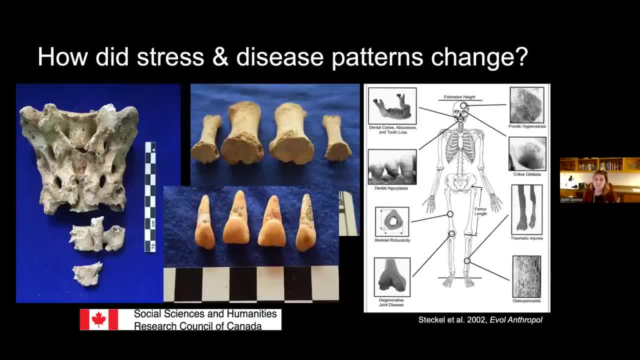 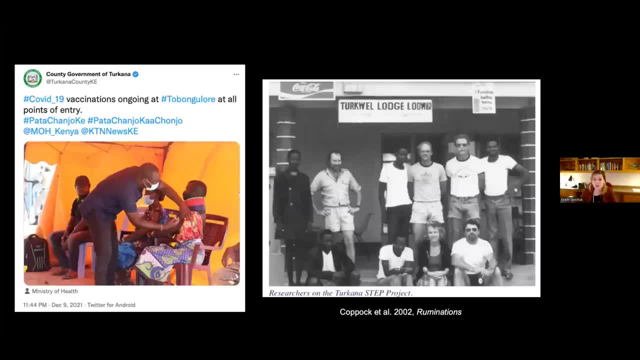 those early herding populations and then trying to consider what that means in terms of not only herding in the past but herding today. And, of course, this is really relevant because we continue to now live and going into the third year of this pandemic, And so health continues to be on the 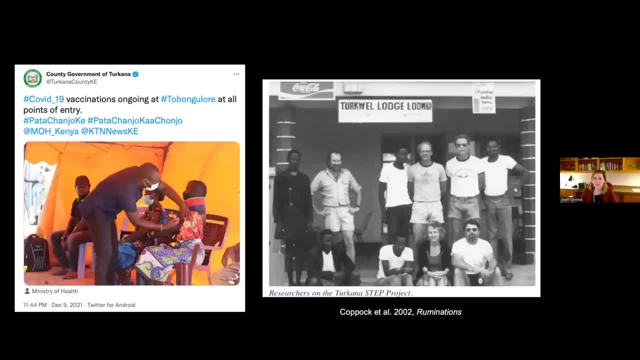 mind of a lot of us, And then also in Turkana. there's a long history of anthropological and biological anthropological research on pastoralism and whether herding is good for people's health or not, Particularly now with global climate change coming back to that. 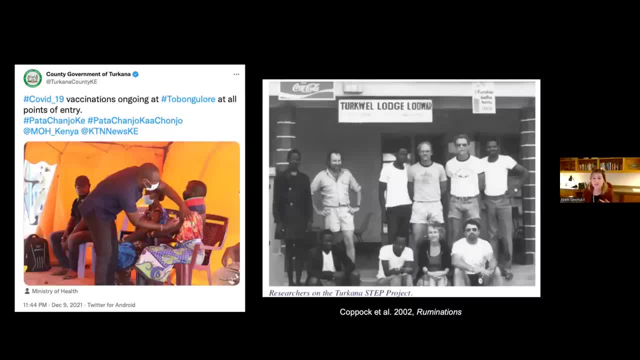 there's lots of questions about if people should give up herding lifeways and settle down and farm, or settle down and have a more sedentary existence, And anthropological writings on it have generally said no, that herding arose in a period now we know of instability and it functions best in those. 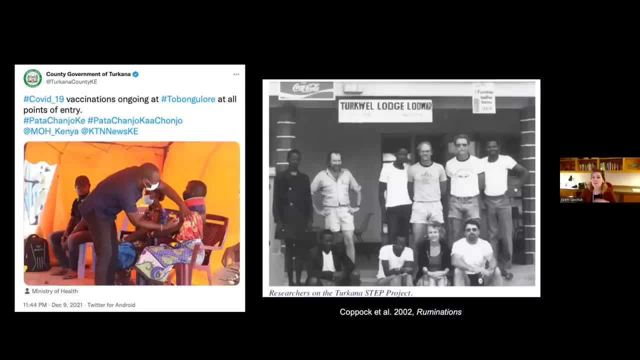 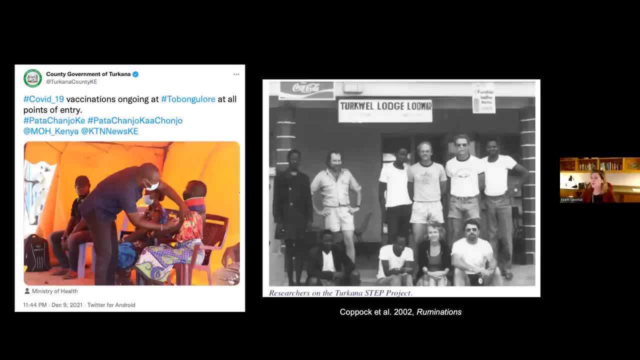 Thank you. So I said: what can we do? And so you just threw it together as one of your different perspectives on herding, but also thinking from a traditional cultural point of view and potentially even an indigenous point of view, but also understanding that this system is meant for this environment and it arose in 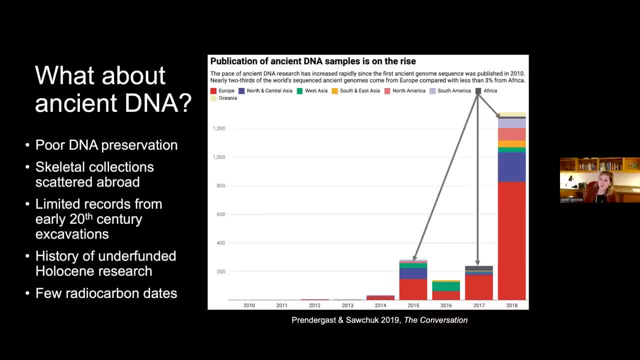 this environment and really thinking about how we can support pasture lists as they continue to live the life that they choose. So talking about archaeology and biological lines of evidence, but obviously at this point in the conversation you're interested in ancient DNA, I would think. 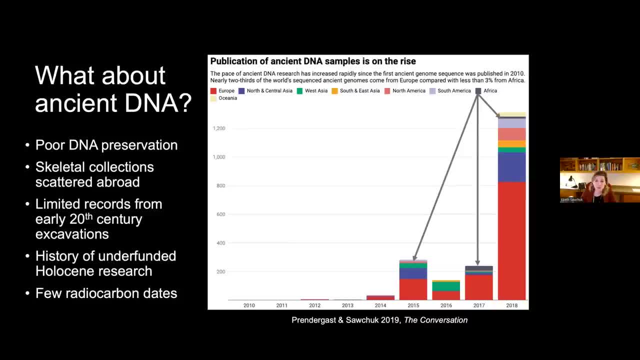 So let's talk about genetic lines of evidence of the spread of pastoralism. We're looking at the biological anthropology, the teeth. we're looking at chemical markers, but why wouldn't we just answer all of these questions with DNA right? 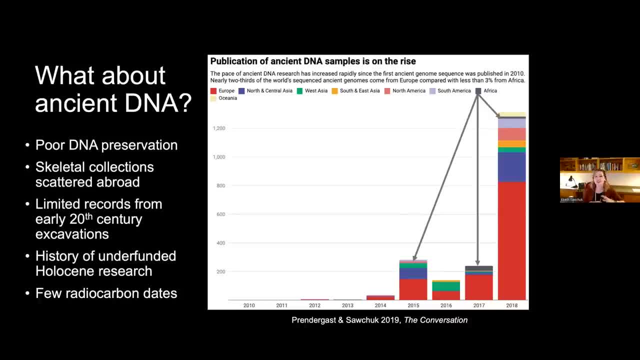 And that's always the kind of question that I get as a bioarchaeologist, you know: do we even need archaeology anymore? We're just going to answer all the questions with DNA. Everyone on this presentation, I'm sure, is laughing, because we've all realized that that's never going to happen. 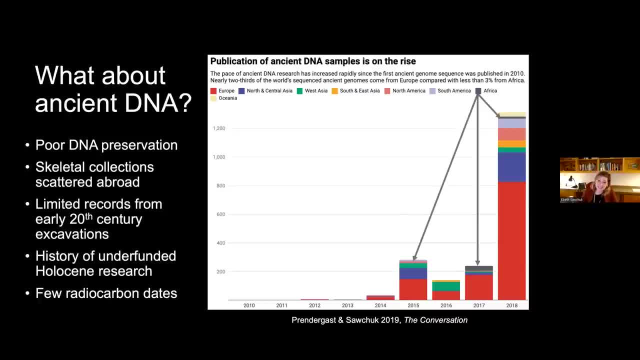 but it bears mentioning why that's not going to happen. It's because DNA is really hard to study in Africa. It's ancient DNA hard mode, And so I always like to remind everyone that this is not a very old science. You know, the first fully sequenced human genome was published in 2010,. 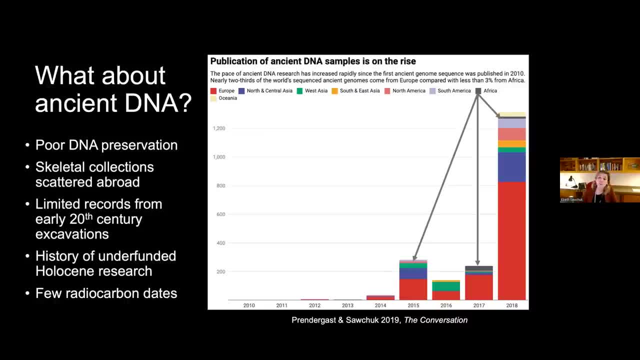 and the first African fully sequenced ancient human genome was only published in 2015.. And so this is a little bit of an out-to-date figure at this point. They published in the conversation. but you can see, not only is ancient DNA fairly new, but in fact Africa makes up an. 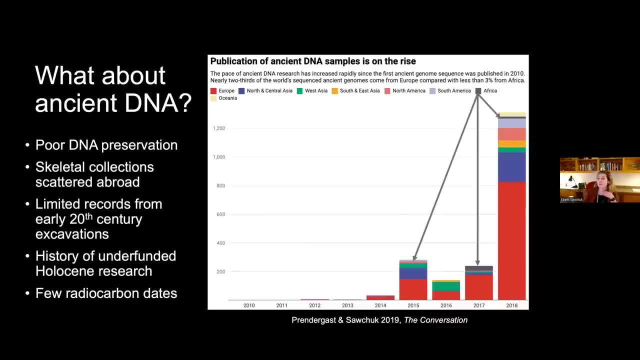 extremely small proportion of the number of ancient DNA sequences that are available, And that's for a few reasons. One: Africa is really hot and DNA doesn't like well many parts are hot, doesn't like to be hot and wet, So the tropics are not great for DNA preservation. 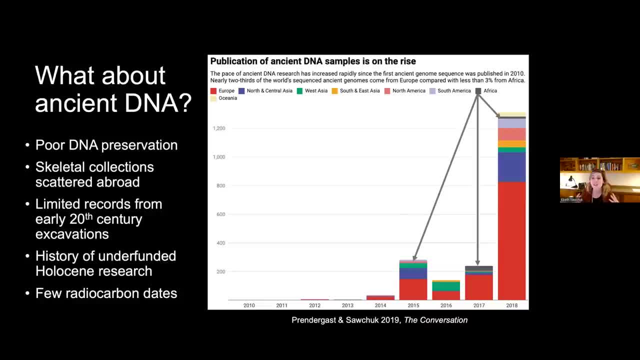 We see this at the pillar sites in terms of the physical preservation of the skeletons. The environment there is very, very hard on collagen. So many of the bones are extremely fragmentary and friable because there's almost no organic material still holding them together. 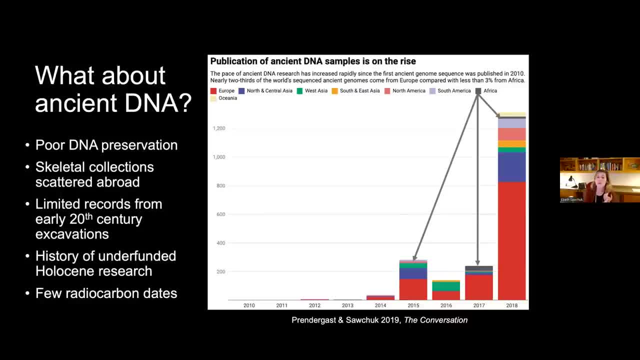 As a result, it's hard to get radiocarbon dates directly out of human remains. The work we've been doing at Lothic is really hard to do, And so we're going to talk a little bit about that. It's also really really hard to get ancient DNA, of course, because that is going to be in the 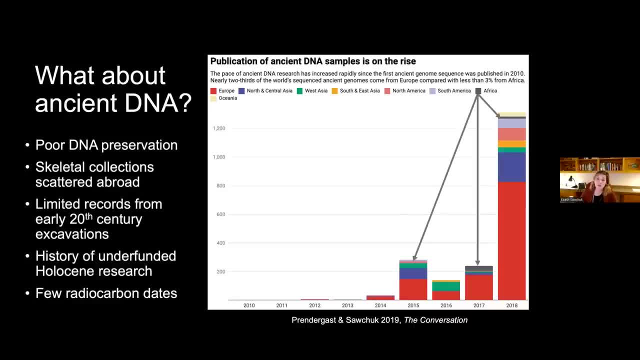 organic component of the bone. We see lots of impacts of the history of anthropology and archaeology in Africa. Many skeletal collections are scattered abroad. We have limited records from early 20th century excavations. And then, of course, as somebody who studies, Holocene events, 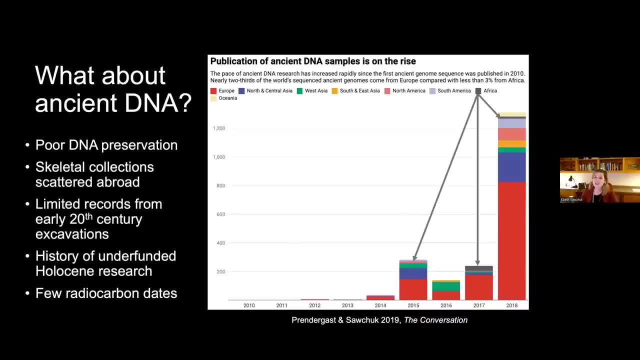 in an area famous for paleoanthropology, I can attest that we get a lot less money for Holocene research than paleoanthropology, And so we're going to talk a little bit about that. And then, of course, as somebody who studies Holocene events in an area famous for paleoanthropology, I can attest that we get a lot less money for Holocene research than paleoanthropology. 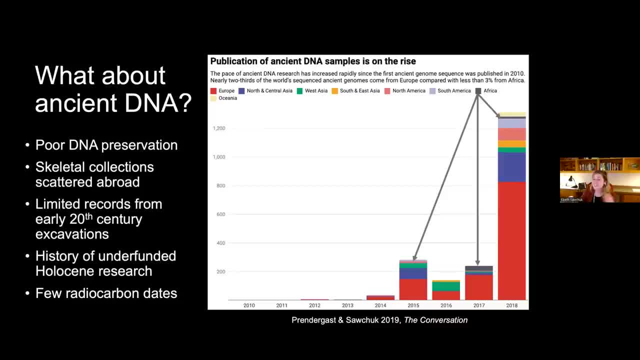 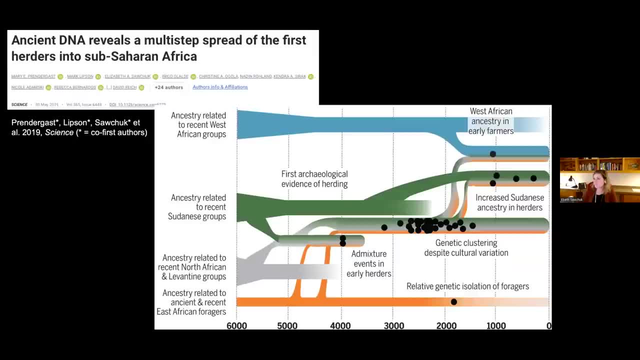 And so that's an issue. And then, of course, we have very few radiocarbon dates, which is both a result of that preservation and a result of funding. But we have been lucky in some situations And we have started to learn more about these. 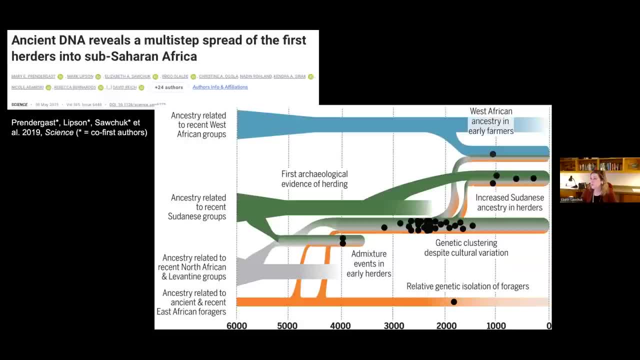 mosaics and been able to take them apart from a genetic perspective. So two years after I defended my dissertation, looking at all those teeth, I had the enormous privilege to go back and sample the ancient DNA from many of the same individuals, And so this is a paper that I'm going to share with you in the next couple of years. 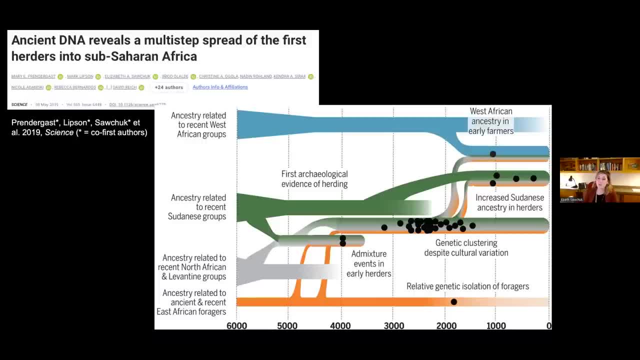 a paper that we published in Science in 2019.. I'm very sorry to say that none of the individuals from Turkana have so far worked, so that remains a bit of a black box, But we were able to sample 35 individuals from that golden age of herding the past- Sternlyolithic. that starts around 3,000. 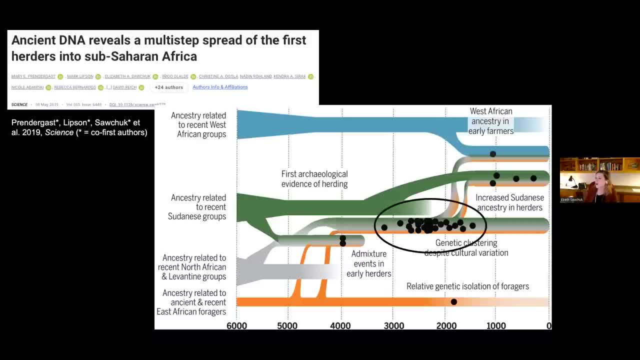 years ago, but really around 25 to 2,000 years ago. So here they are right now. We were able to look at admixture analysis to determine that all of these individuals are descended from both North African populations as well as East African forager populations, and we were able to. 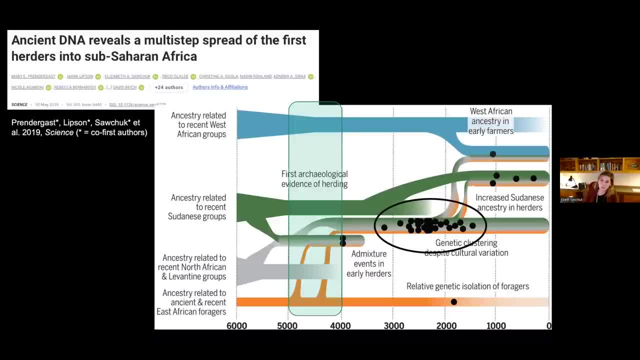 estimate the date of that admixture to be right around when we see the first archaeological evidence for herding. So now again, this doesn't suggest that this extensive gene flow happened around the Turkana Basin, but that's a now testable hypothesis that we continue to follow up. 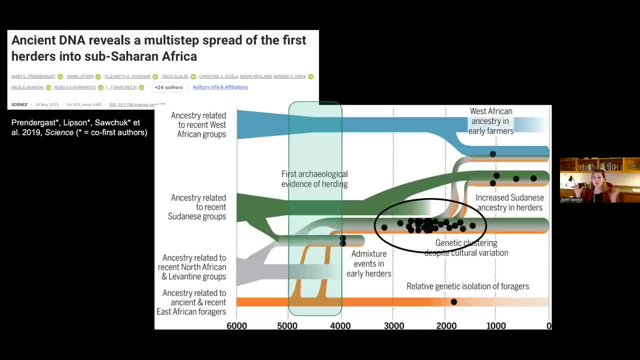 because it does seem that in that situation where you have groups coming together, you know you have the dental morphological evidence for potentially gene flow or at least biological similarity, and then you have all of this sweeping cultural change. maybe this produced the conditions where you start to see that gene flow in exchange. 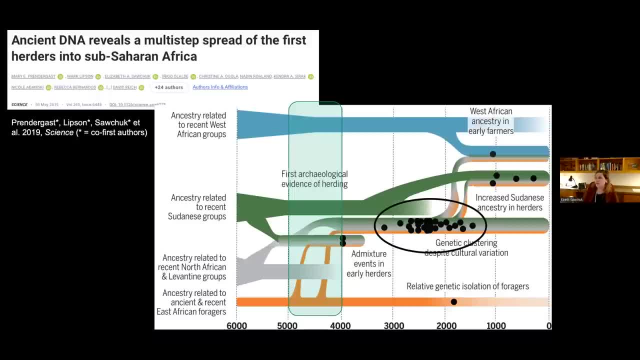 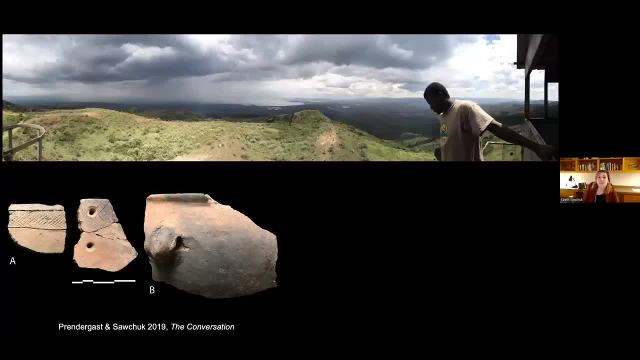 with the birth of East African pastoralism. So this is an image of the South Central Rift Valley where all those wonderful pastoral Neolithic sites are, some quite famous, some excavated by Lewis and Mary Leakey, And one of the things that we always talk about is in the 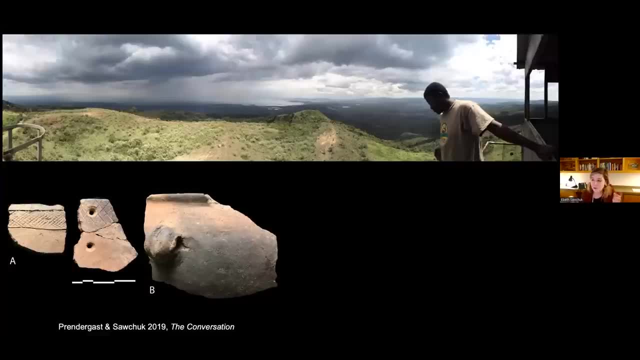 pastoral Neolithic. you have this great diversity of cultural traditions of people herding in the Rift Valley at the same time. On the left you have the beautiful savanna pastoral Neolithic tradition based on pottery, and on the right you have the slightly more lumpy almond titan pottery tradition. 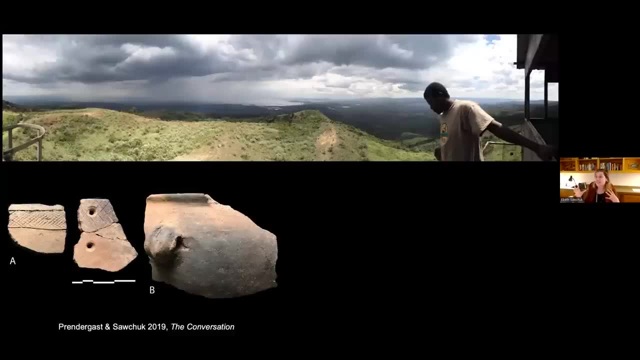 Because these herders are using different pottery in the same place at the same time. the assumption, archaeologically, has always been that they're very biologically, linguistically and culturally different. Different pots equal different people. When we were looking at the ancient DNA, we found womp, womp, that in fact. 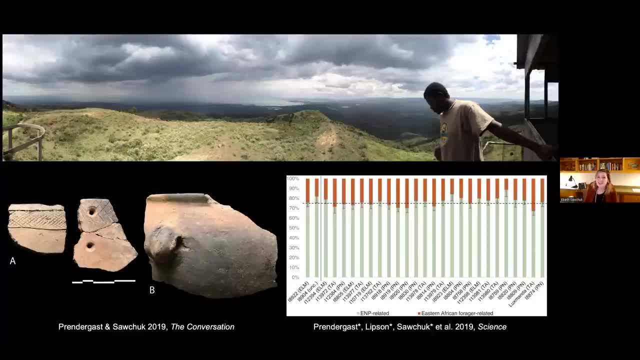 all of these individuals are extremely biologically similar, And so again it goes to that mosaic, again that just because people are practicing different cultural traditions doesn't necessarily mean that they're biologically unrelated, And so this adds some depth to that mosaic. 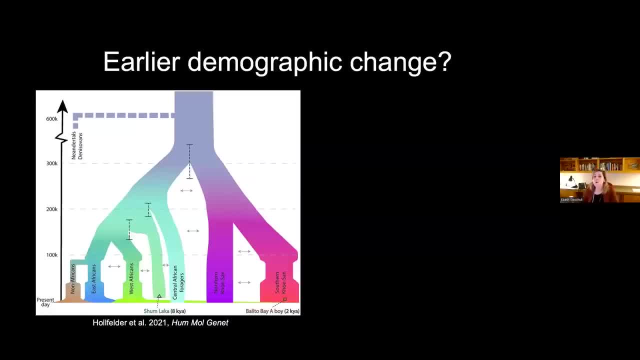 Kind of pivoting a little bit. ancient DNA has also let us look at some older, some older events in the population history of our species. So one big archaeological mystery in African archaeology for the past several, several decades has been the question of the middle to later Stone Age. 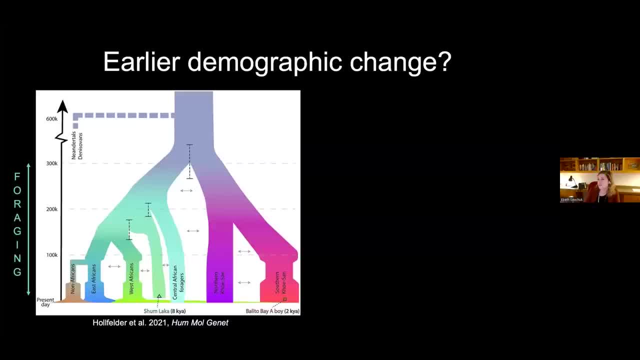 transition. So here's this fussy thing Again, and we can see that in fact the vast majority of our history is foraging. So all of that food production happens in the past 8,000 years in Africa, But most of our time depth on the continent. of course we were hunter gatherers. 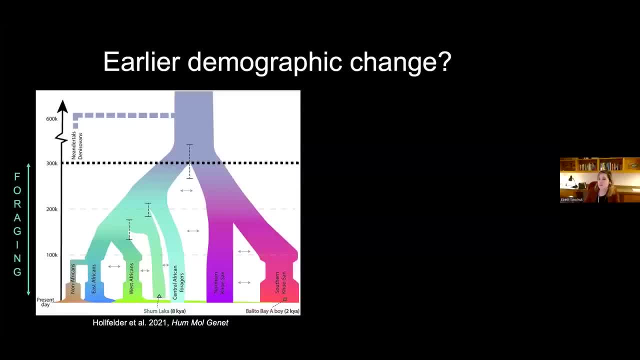 And so around 300,000 years ago we see a transition from the early to middle Stone Age And that lines up exactly when we think our species emerged. Great, Everyone's happy with that, you know great timing, But around 50,000 years ago we had this transition from the middle to later Stone Age. 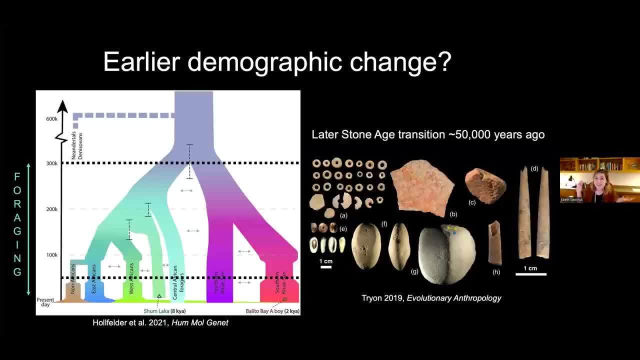 and it's not associated with any evolutionary events. It's not associated with any event that we can see in the fossil hominid record, But we see lots and lots of changes in behavior and the material culture. We see ostrich eggshell beads for the first time become a widespread thing. 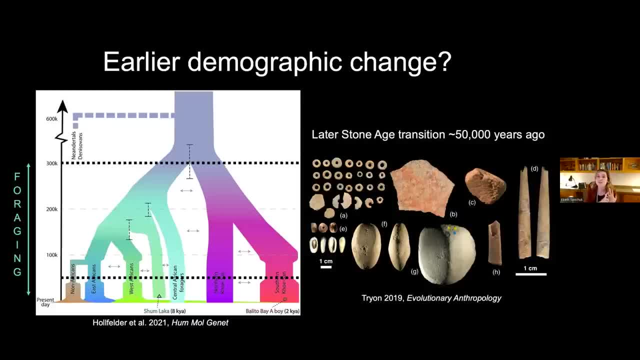 We see different forms of symbolic artifacts. We see different types of stone tools. We see evidence for long distance exchange networks. It's something really profound. seems to happen that in the past it had been suggested that maybe this is the invisible neurological change. 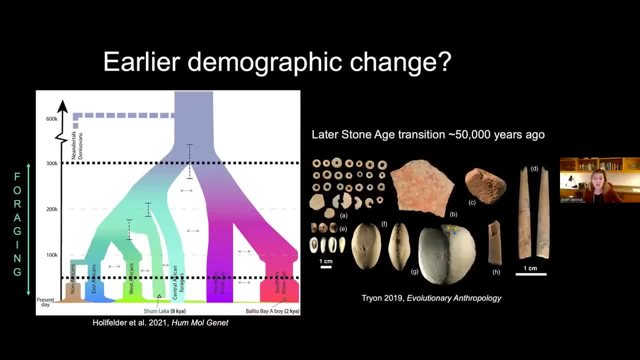 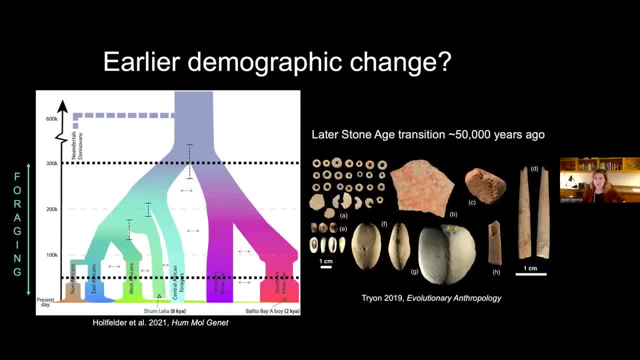 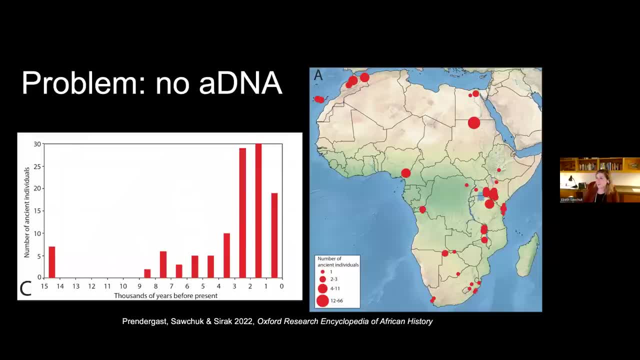 And that's when they were able to leave the continent of Africa. That's been a very unsatisfactory explanation for the past 20,000 years, but it still begs the question of what exactly is happening at this transition. So let's test this with DNA. 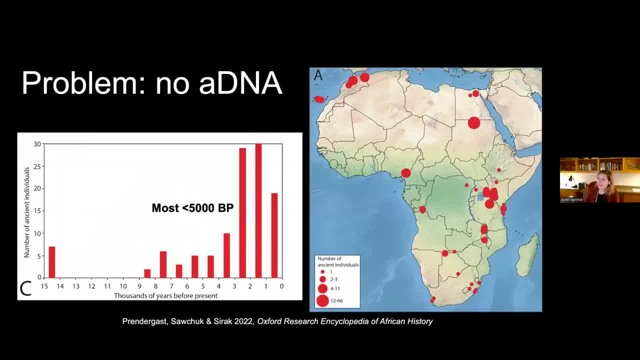 Unfortunately, it's been really hard because, in fact, most ancient DNA from Africa is less than 5,000 years old And, as you now know, the last 5,000 years have been very fussy. And then also there's just fewer ancient DNA sequences from Africa than the rest of. 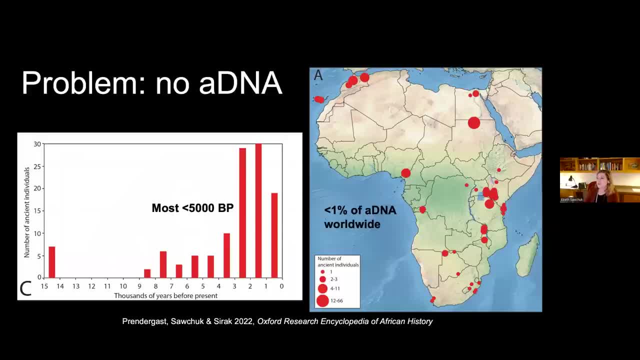 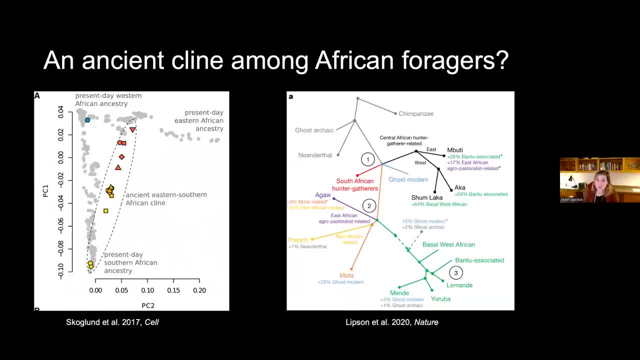 the world. We're looking at just over 100 sequences at this point, And so this is less than 1% of ancient DNA sequences worldwide, But based on the few sequences we do from ancient African foraging populations, we have seen some patterns. 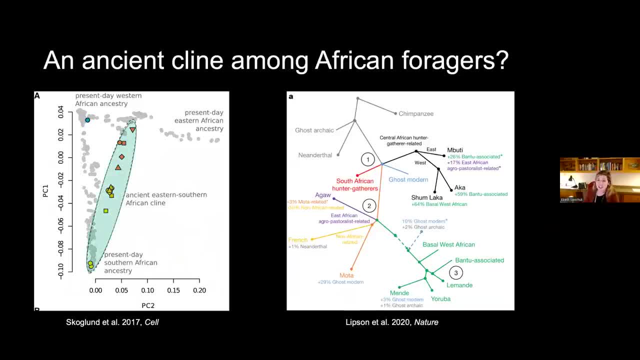 One is in this 2017 paper, There appears to be a cline of variation between eastern and southern Africa, which suggests that these populations were maybe in contact with one another, And the other thing from this 2020 paper is we see that there's deeply divergent lineages. 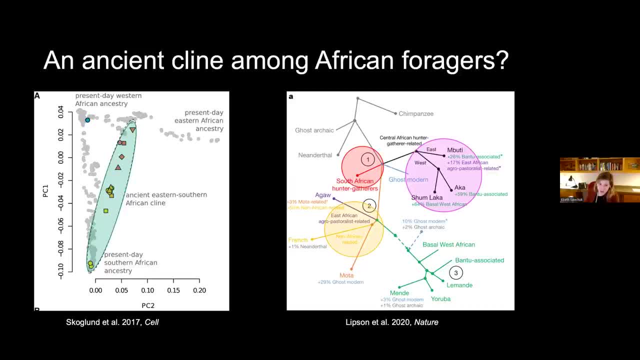 between eastern Africans, southern Africans And also central Africans that split pretty early on, And so it's really interesting to think about how potentially these groups may have split and then their interactions with one another. But all of this is based on very few individuals, who all lived within the past 8,000 years. 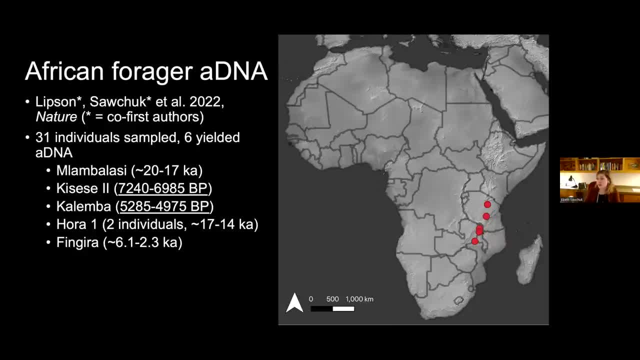 So a paper that we published earlier this year in February in Nature was trying to pull off the lid of what exactly is happening in the later Stone Age. So we sampled 31 individuals from a bunch of different sites that were specifically from the past 10,000 years old. 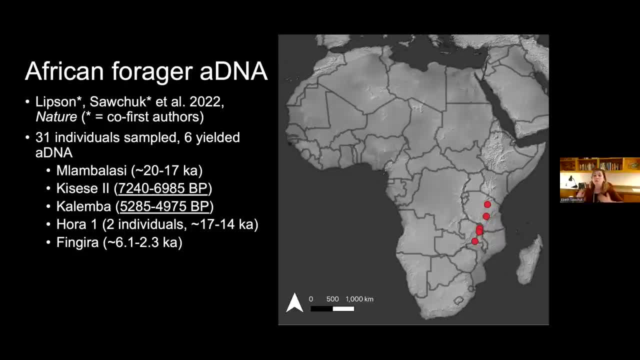 associated material culture from the later Stone Age that we believed was going to add to date the spread of herding into those various areas. Ancient DNA is really hard in Africa. so six yielded sequences and we were ecstatic about that, And so we have individuals from Tanzania. 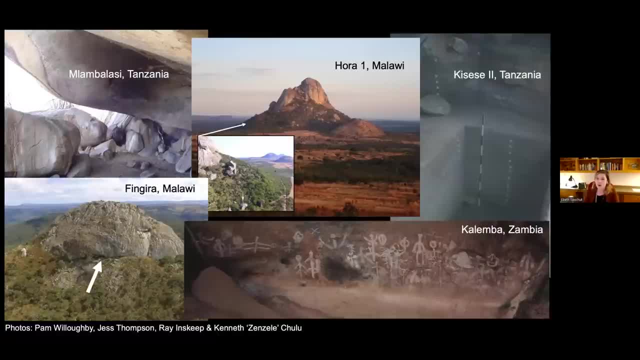 Zambia, as well as Malawi. These are the sites. They're all caves and rock shelters, which also tells us something about if we hope to get ancient DNA from different parts of Africa. that's probably our best bet for the older stuff. And then what we did was we compared these six. 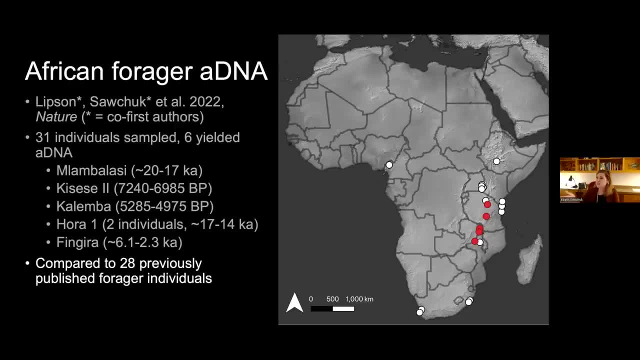 new sequences, and I forgot to mention the ones that are directly dated. there are Kisisi and Kalemba, but we compared them to 28 previously published forager individuals and we generated higher coverage for 15 out of 28,, so we're feeling pretty great about that, And so our final sample. 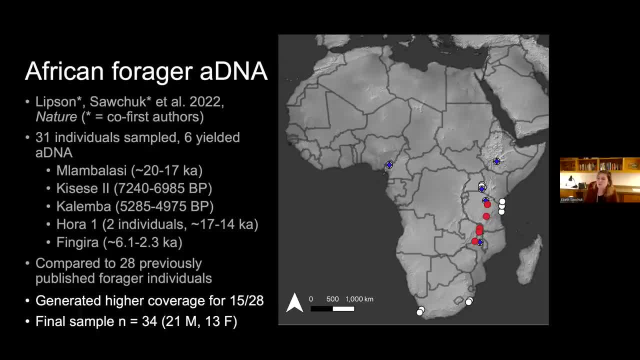 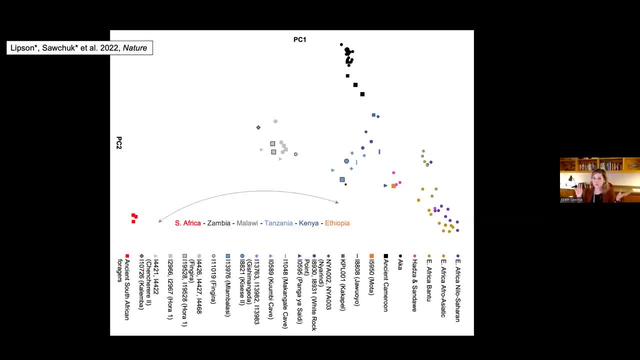 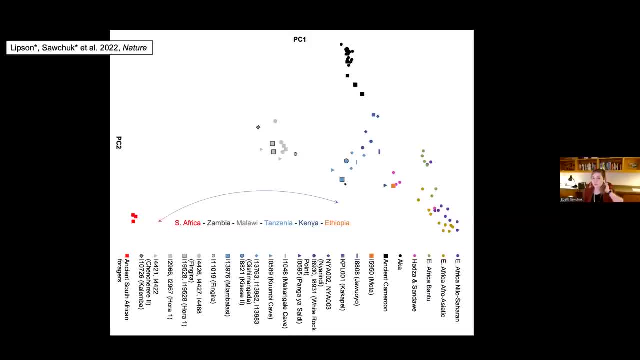 And what we did here was a little bit different than usual. We actually created a supervised PCA- and you can read more about that in the paper, in the methods- where we projected a two-dimensional axis of variation, with Southern Africans here and Eastern Africans here is defining that variation. 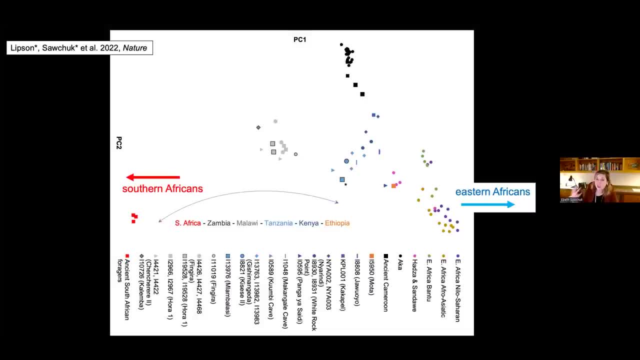 as well as contemporary Central Africans, And then we projected our ancient individuals onto that supervised PCA. So here are our new individuals here, and what we can see is they clustered geographically with their neighbors, and then we projected a two-dimensional axis of variation. 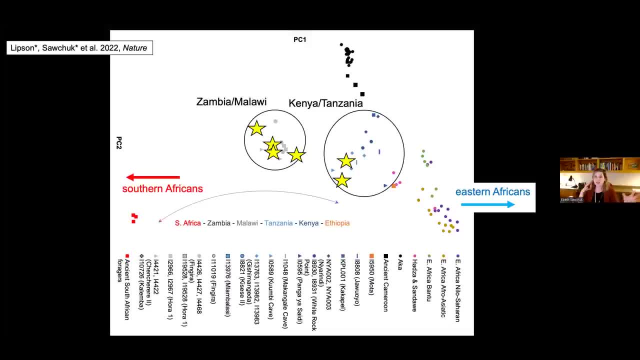 with their neighbors and then we projected a two-dimensional axis of variation with their neighbors, but in fact this doesn't look like it's a straight two-dimensional line, like that cline that we were thinking of that might exist between Eastern and Southern Africa. 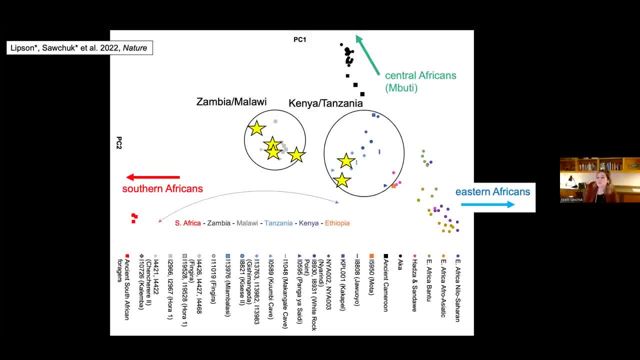 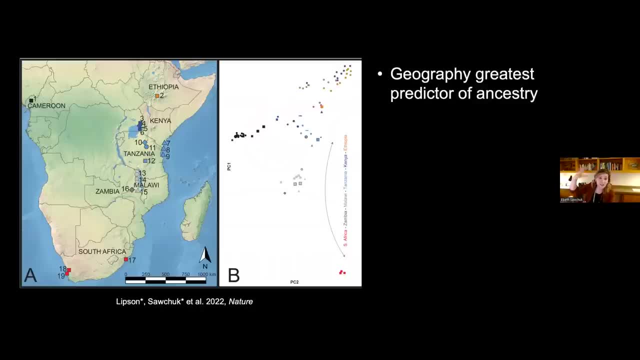 In fact, these samples are skewed towards Central Africa, so it's actually a three-way cline instead of a two-way cline. This makes more sense when we pop, when we rotate the PCA and pop it next to a map of Africa. So here is the individuals from Malawi and Zambia. here are the individuals from Kenya and Tanzania. 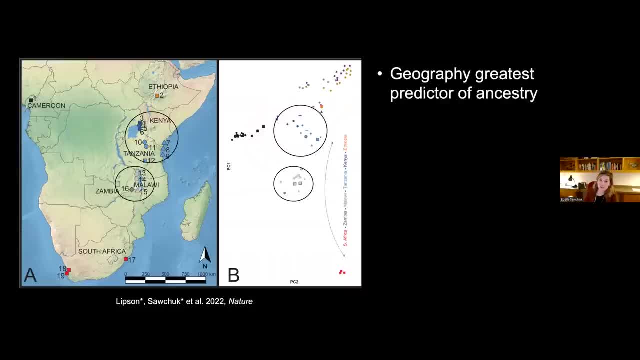 and what we find is that geography is the greatest predictor of ancestry of all of these individuals, So they were more likely to have children with people who are living close by them, and that this is really important to understand by the earliest time these samples were around, which is about 20,000 years ago. We also can see that they're shifted towards Central. 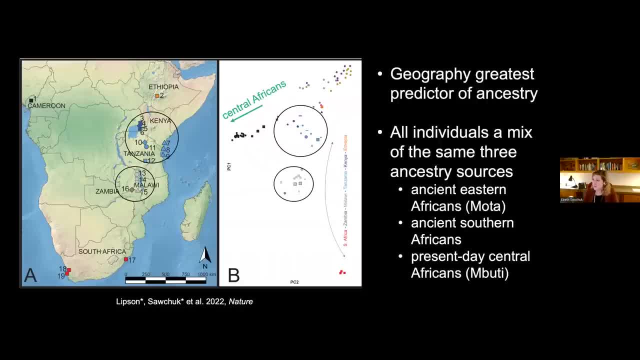 Africa. What we take away from this is that all these individuals are a mix of the same three ancestry sources that can be defined by ancient Eastern Africans, as represented by the Mota individual from Ethiopia, ancient Southern Africans and then present-day Central Africans, represented by the Mbuti. And so we did a bunch of statistical tests, but the key to this 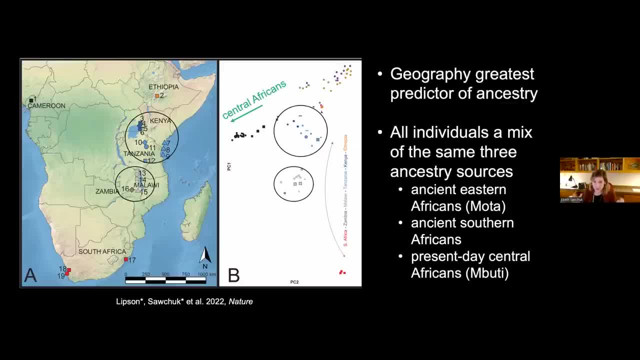 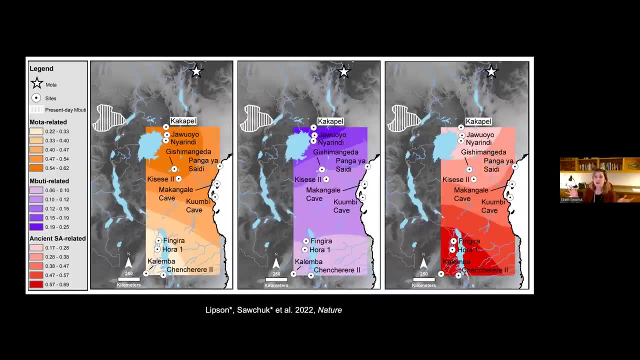 is that all of these individuals have the same three ancestry contributors, but in different proportions, and this is really important for understanding patterns in the past, because the only way that we would be able to explain this is if there had been extensive gene flow throughout this entire area. that would have moved Eastern African ancestry all the way to South Africa. 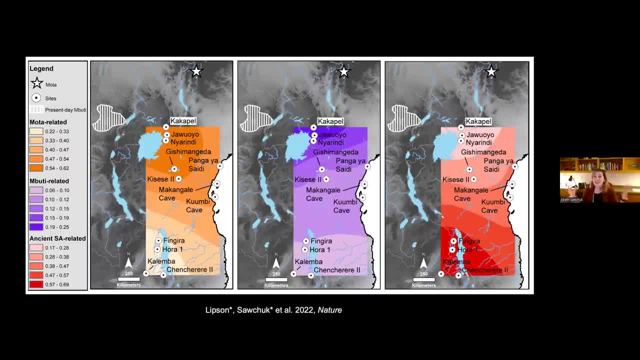 Southern African ancestry all the way to Ethiopia, and then also Central African ancestry throughout, And so this is also from the paper where we looked at these ancestry proportions in a heap map. summing them to one and you can see the ancestry proportions in different areas, is more likely to be closer to the geographic area we'd see. 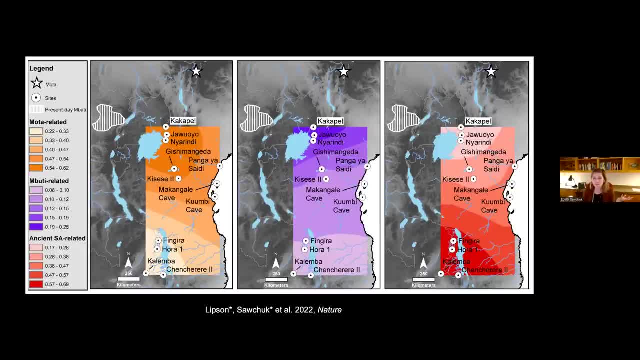 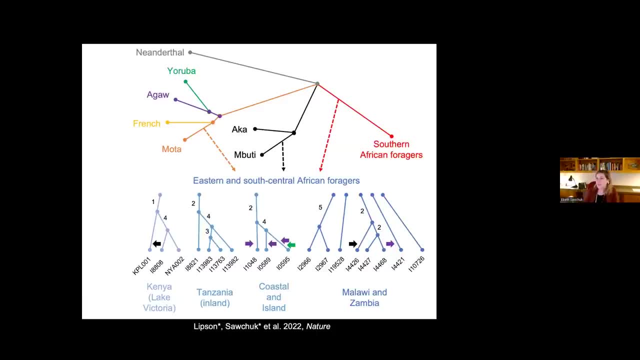 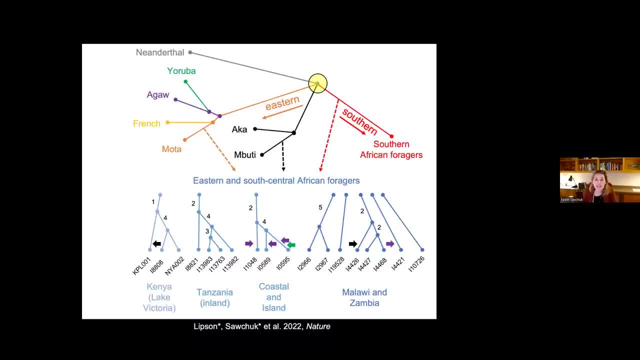 split between Eastern and Southern Africa happened. foragers happened around 80,000 years ago, and we know the split off from the Central African foragers, represented by the Mbuti, happened about 50,000 years ago, And so we now have a timing for when this gene flow took place. 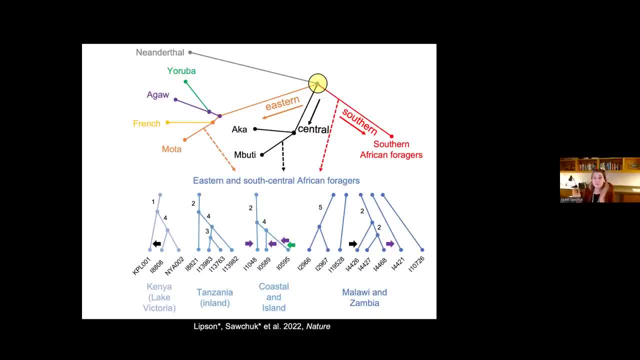 It must have happened after 50,000, but before 20,000, because that's when the oldest individual from the Lallamalazi in our sample was there and already this three-way climb had been established by then. So in fact this lines up pretty much exactly with the later. 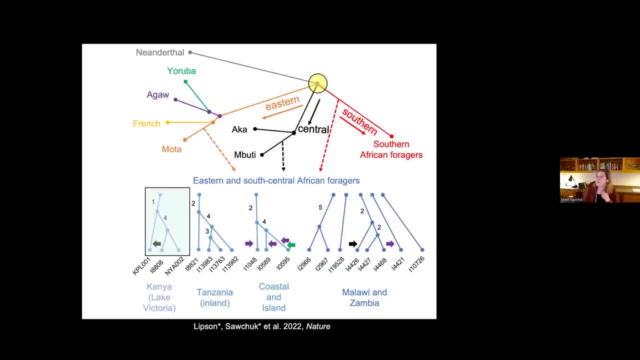 Stone Age Revolution, which is really, really interesting to think about. We also found that there's differences in gene flow in different parts of Africa during this late Pleistocene period. So in Kenya, Tanzania and around the coast we actually still see regional gene flow. 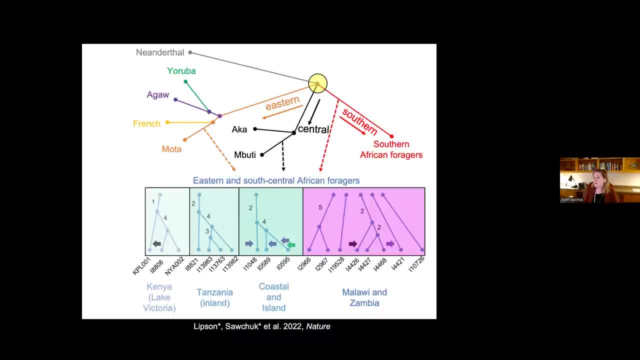 even as people are starting to live more locally And for some reason in Malawi and Zambia, people are no more closely related to people from other sites in this area than they are to individuals from Eastern Africa. So, truly, we're only seeing people exchange genes with people in. 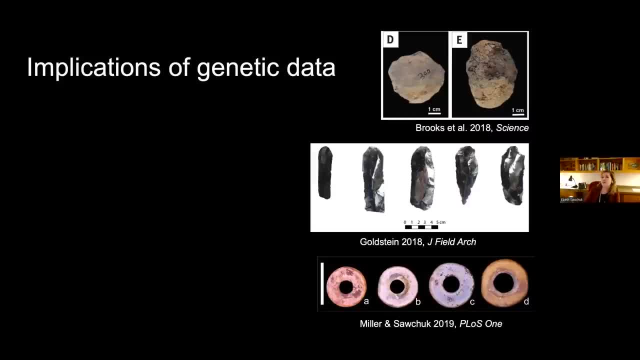 their extreme immediate area and time period, of course. So what does this all mean? Implications of genetic data. we're trying to understand this. So the fact that individuals are all a mix of Eastern, Southern and Central African lineages suggests there is a period of extensive human 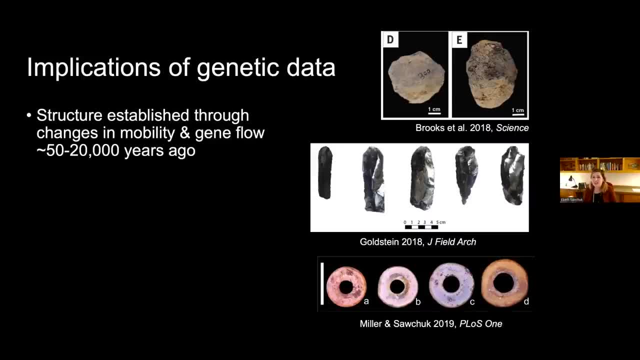 mobility and mixing in the late Pleistocene. We don't know exactly when this must have been, but it was between 50,000 and 20,000 years ago, So right during that later Stone Age transition Archaeologically around. this time we see. 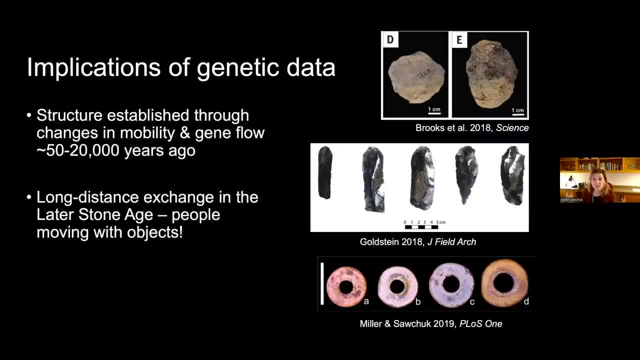 based on chemical markers, the movement of objects. So we see the movement of obsidian, we see the movement of ostrich egg shell beads and we see the movement of ochre, And so kind of a big open question to archaeologists have always been: how did these long-distance exchange networks? 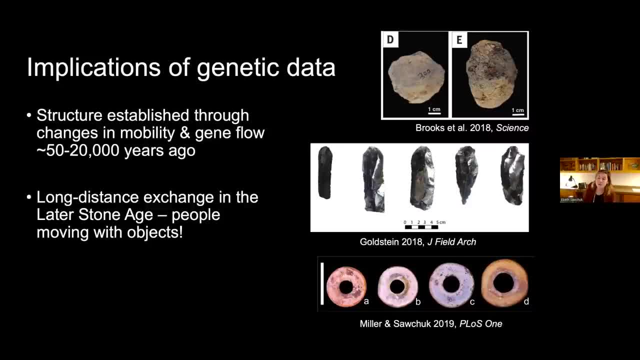 get set up. Was it just the objects moving or was it also people moving? And what we can tell now from the genetics is it really looks like people were moving, which is really interesting to consider. We also know that by 20,000 years ago, which coincides with the height of the last glacial. 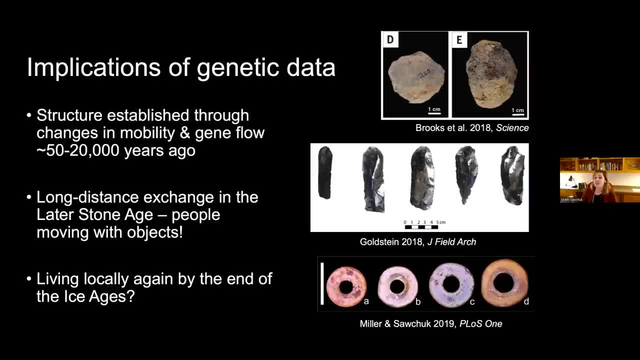 maximum. people have started living really locally again and having children with people who lived in their immediate area, And this coincides with the phenomenon that has been reported archaeologically known as regionalization, where different technologies of the later Stone Age start to get more regional. We start to see more variation culturally, And that is also lining up with now. 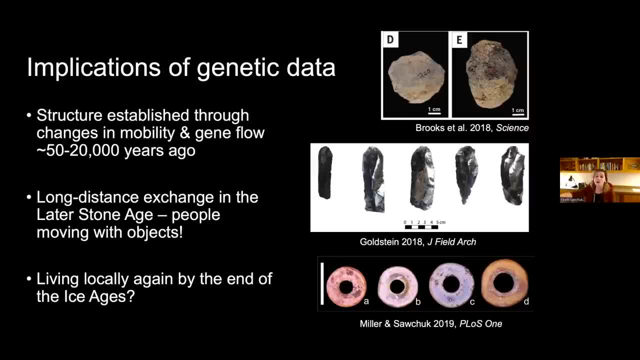 what we think is that people are starting to live more locally And even though we don't have a lot of longer distance exchange networks, people are still moving. But people are still moving. We see a huge increase in the rate of change in the last century. If we look at Jaeger's map, we can see that. 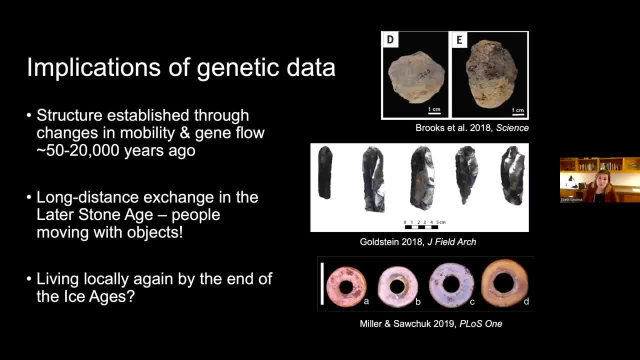 people are still moving. even if all of those long-distance exchange networks are still in play, people aren't necessarily moving as much as them, And so this is really, really interesting when we consider how humans survived the last ice age, The way that populations coming together and then 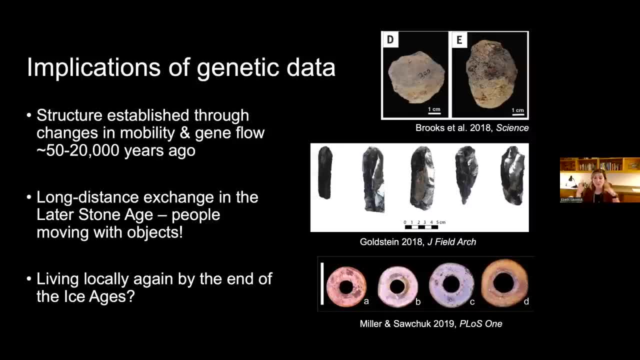 staying apart would have structured genetic variation. We can think about this in terms of the archaeological record. We can think about this in terms of the linguistic record, the historical linguistic record, And this is really, really interesting when we start to think about what. 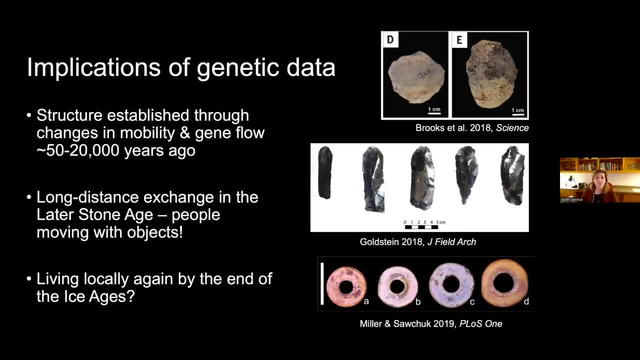 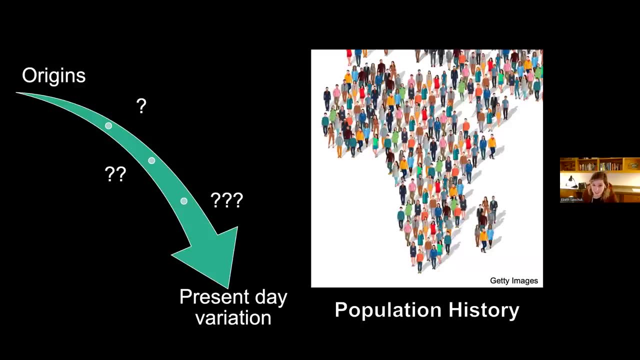 people are actually doing during that time period in history And where that time period is really looking forward. Yeah, about what people are actually doing during this time and how that structures the variation that we see today. so you know, this is all coming back to population history and me trying to convince, 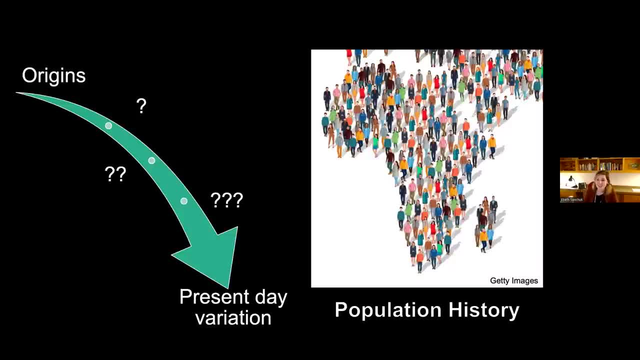 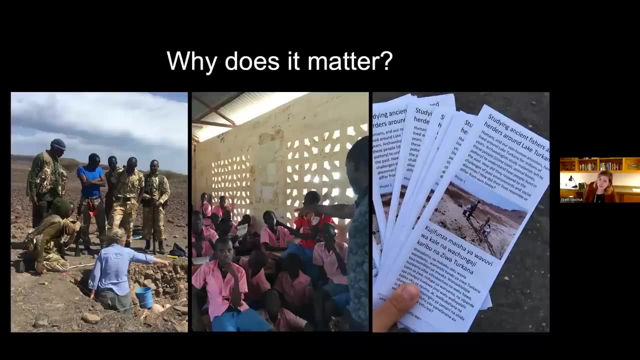 you that, although human origins and evolution are really, really exciting, we really have to think about humans in terms of the entire story. i'm really understanding that population history because it's really important for understanding not only the history of our species but also the world that we live in today. and at the end of this presentation i always want to end up with: 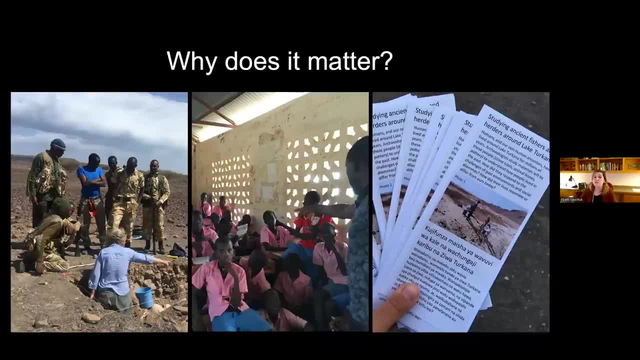 talking about living people today. why are we doing what we're doing as archaeologists and biological anthropologists, and what impact does our work have, not only on the people living today, but also the people in the future? and then, of course, you know what is our responsibility of doing this research. 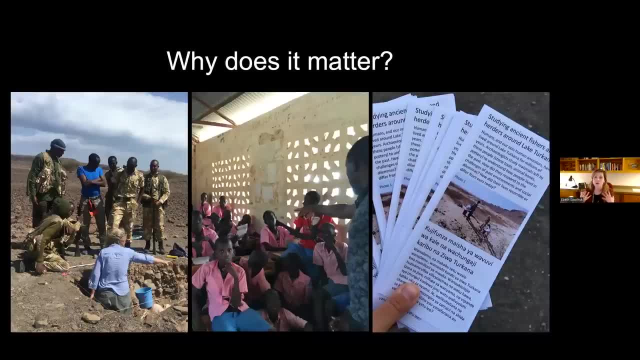 because it comes at a high cost, and that high cost is that it involves a lot of research on ancient human remains. so, of course, most archaeological teams, including our own, engaged in a lot of community engagement around our sites, you know, talking to people about what we're looking for, trying to make sure that. 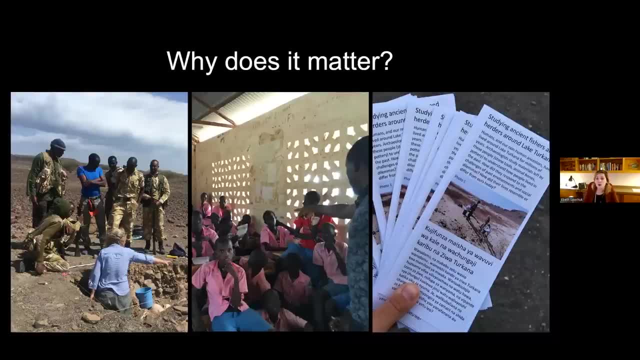 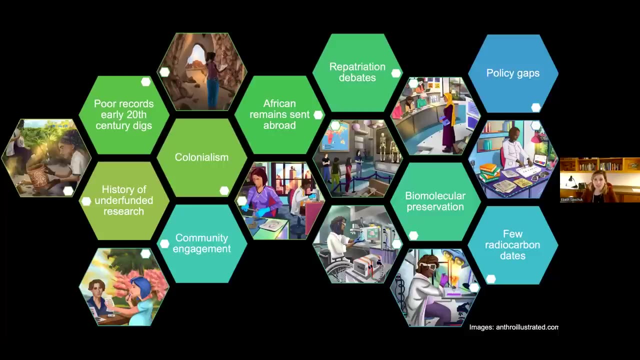 our results get out, and then, of course, partnering with local communities and partnering with local researchers as well, to try to co-create this knowledge and ask the kind of questions that are more interesting from a local perspective as well as from the kind of perspective that we would bring into that area. but everything that we do is enmeshed and nasty in a history. 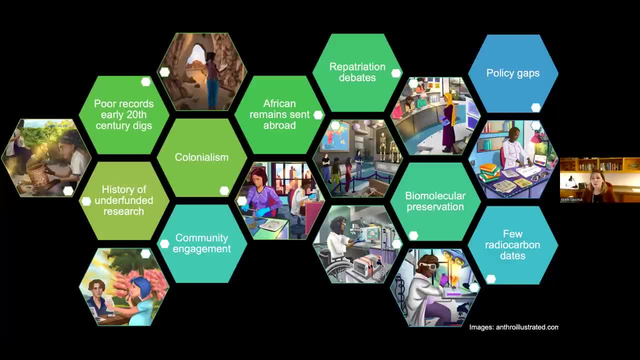 of colonial archaeology anywhere you go in the world, and that's something that, of course, is nothing new, but something we have to think about, particularly when we work in africa. these are all the things that make uh doing ancient dna difficult in africa, but it's also something important that we have to think about when we're doing contemporary archaeology. 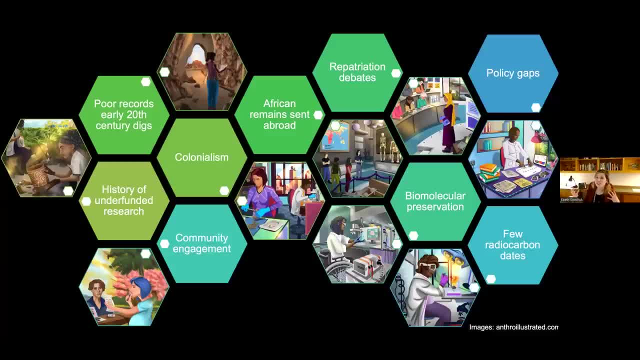 because we're working in a system that has already been set, like this, which has a series of barriers for us actually doing this work not only in the best possible scientific way, but in an ethical way, and it's really important particularly to think about ethics in the terms of ancient human. 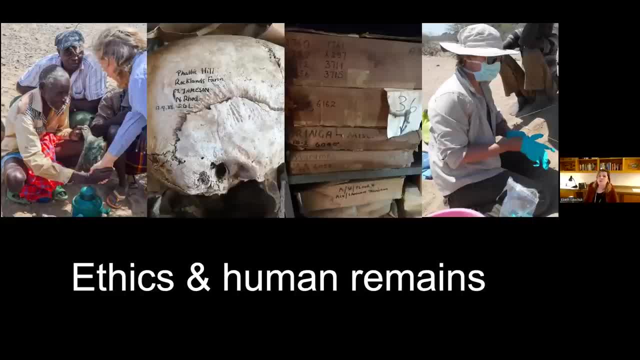 remains, and my experiences in the field, and also now working in a museum, really make me think about how we interact with local descended and guardian communities to seek permission to do excavations and study human remains. what do we do with colonial era skulls that we do not have good? 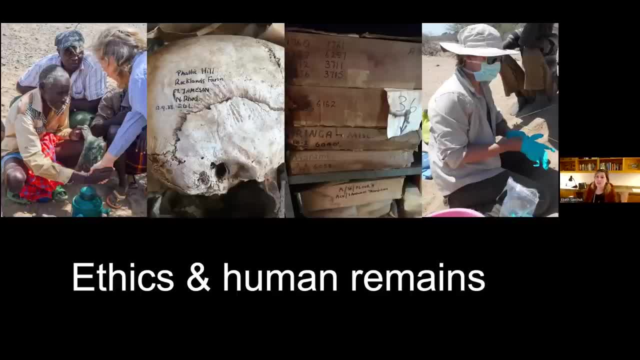 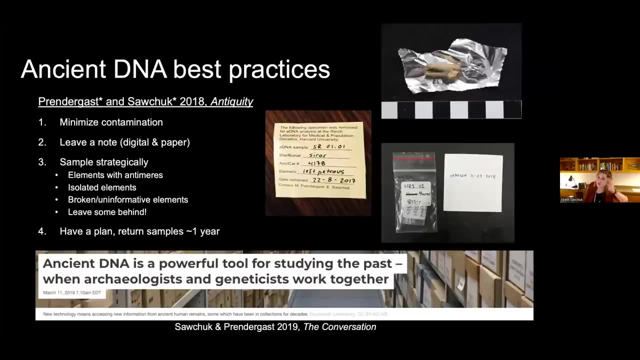 information, for how do we support local museums in africa beyond just leaving our artifacts there and working with local curators? and then, of course, the questions about ancient dna and how we balance scientific research with destructive sampling for new and existing collections. and i'm not going to really belabor this point, but one thing i want to share particularly. 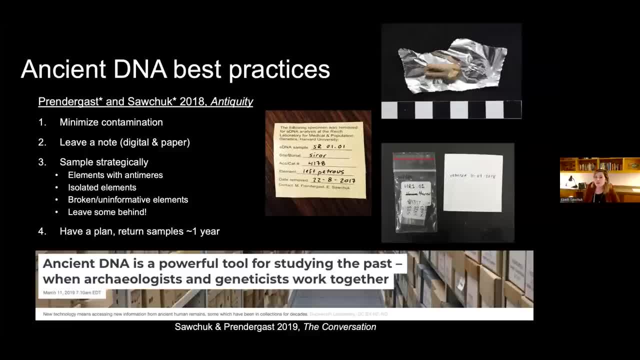 because this is um- you know there's lots of students in this group- is that we all have a role to play in ensuring that research is done better in the future and your particular skill set is going to find a place in terms of the bigger conversation about how we shift our field. 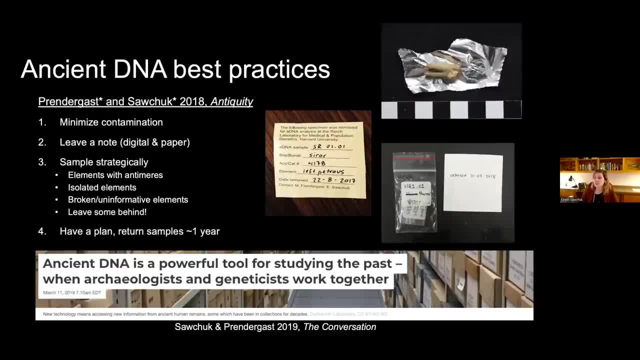 one thing that became immediately apparent to me when i started working in ancient dna is that there were no protocols for sampling ancient dna and, as a bioarchaeologist, things to me were pretty obvious. for example, if you're going to take a sample and consign it to destructive analysis like wear gloves. 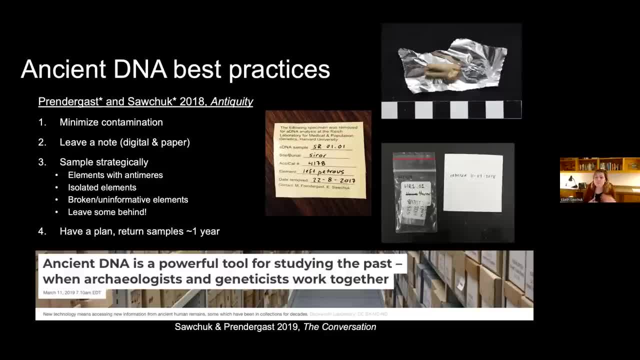 wear a mask before it's cool. don't leave your dna on it. um, leave a note. you know it's great to also leave a an excel sheet with the curators at a museum, but leave a physical note in the tray, return things within a year and then say on the back that it's been returned and was it sampled? 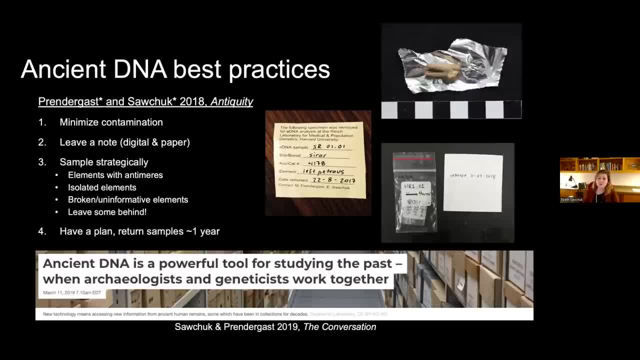 or not sampled and then finally sample strategically. so again, as biological anthropologists, there will come a time in your career where somebody asks you for samples or access to ancient dna samples, and these are the kind of things that you should be saying: pick an element with an. 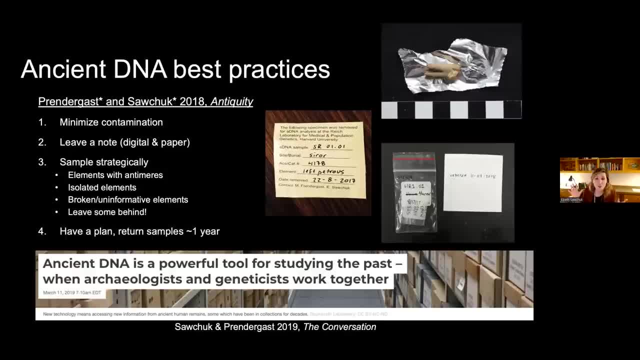 antimer. you can use a busted tooth. you don't have to pick the prettiest tooth from an individual. in fact, ancient dna goes up through the root and samples of pulp cavity, so you can use something that would not be useful for morphological studies. um, you know, take broken and uninformative elements. 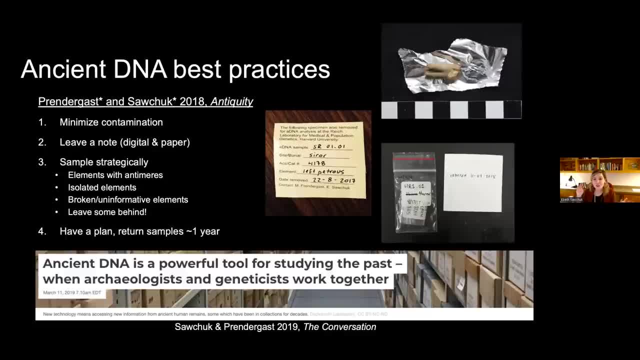 you know you don't want to have something that has a unique non-metric trait or that has evidence of pathological changes. leave those behind, unless it's part of your research design, and then, of course, always, always, always leave something behind. you know we, 10 years ago we didn't have ancient dna. 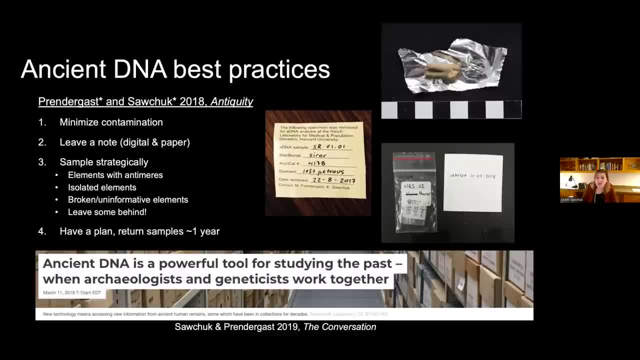 from africa, and things have changed so much, and so particularly now as a curator. but it behooves all of us to think about what's going to be possible in the next 10, 50, 100 years, and what are we doing now to ensure that that research can proceed not only in an ethical way, but also 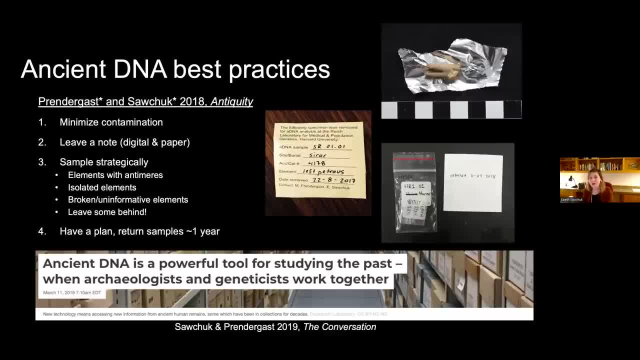 logistically and make sure that the right documentation, the right records and the right anti-contamination protocols have been taken now, so that we don't- uh, we don't- stop any research in the future. so anyway, i wrote this all up with mary prendergast in antiquity. 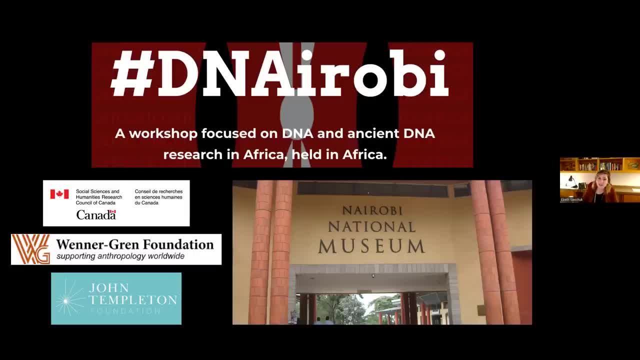 so you can also check out that. and then, as a final plug, you know, we obviously also have to start having conversations in different places. uh, having these virtual seminars is so amazing because people from all over the world can attend, but one of the things that we're not so great at is talking. 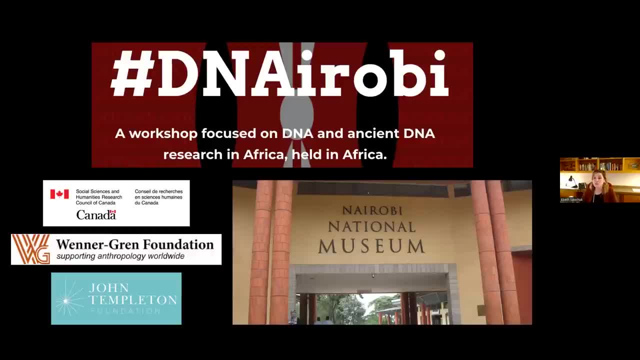 about african dna in africa. most conferences are in the global north in europe, north america and australia, and so one of the things my colleagues at the national museums of kenya and harvard and rice and i are doing are actually holding a workshop on ancient dna about africa in 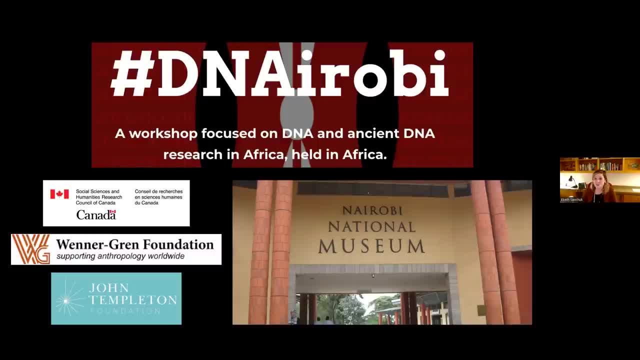 africa happening in nairobi in may and so happy to share more information on that. but truly it has to be a community level thing as we start to consider not only the kind of research we're doing but how we're doing it. so with that i want to thank you all and i want to acknowledge the so 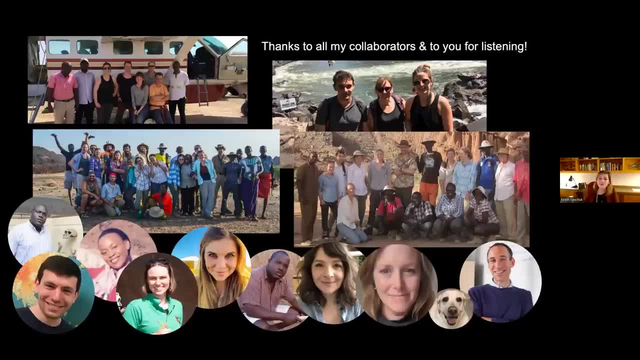 so so many people that went into creating all of this knowledge for me, and i'm so happy to take your question, thanks. thank you very much for that fascinating and really interesting talk and yeah, so if anyone has any questions, then you're more than welcome to unmute yourself and ask, or you can pop them in the chat and then i 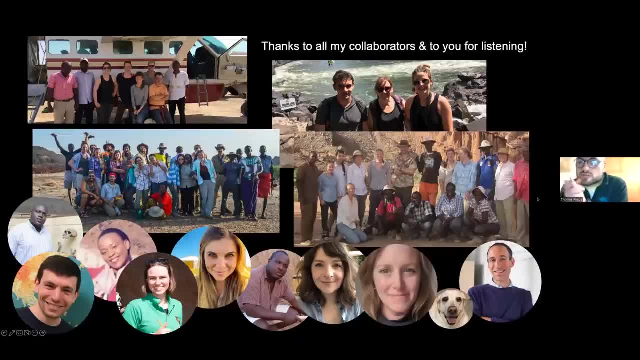 can read them out for you. so got one from jared here. hi, you bet. thank you so much for that awesome talk and your contributions at the end. um, and going back to that kind of community engagement part, so i was wondering: um, obviously there are still people living in tucana today. 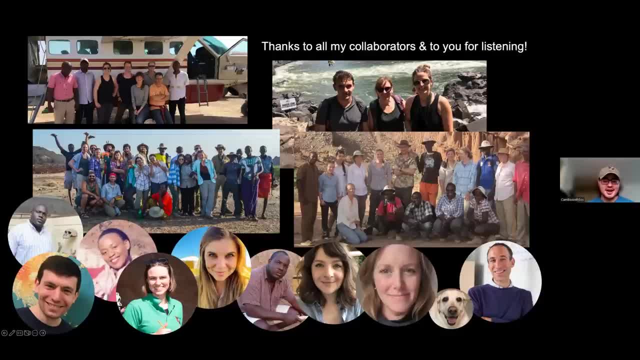 if you've asked them about these burials and maybe learned, maybe about, i guess, more about the burials from them? um, one of my questions was: um, do you know anything about the status of the individuals buried there? um, i know they're buried with lots of artifacts and um you said people were moving long distance with them and i know, i guess, for me. 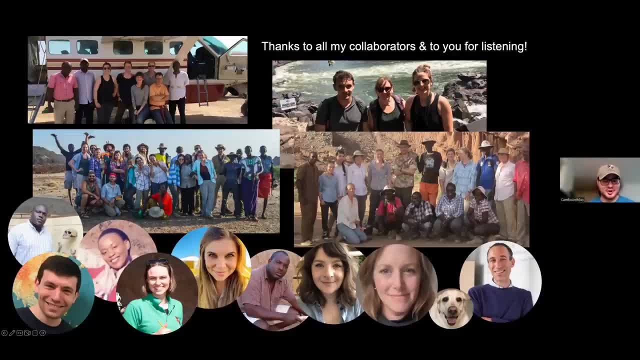 if i moved a long distance with something valuable from far away, maybe i might be less inclined to, you know, leave it behind, um. so maybe that goes to say, maybe it's like: um, some people just like put down the death of some kind of, uh, very old animal, and not really even ostrich eggshell necklace or or, um, some hippo teeth. 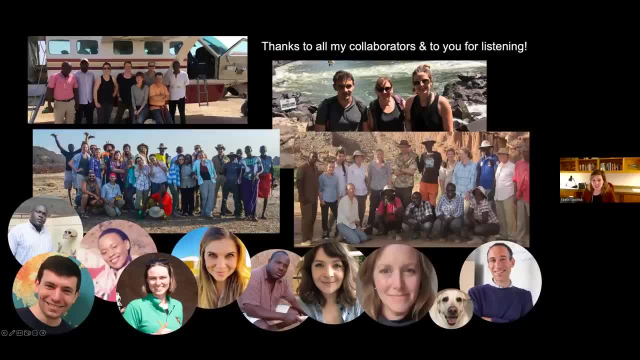 they're very hard to get. uh, maybe these people had some status, so i was wondering if you had anything to say about that. yeah, there's kind of two parts to that question. one is, um, talking about people, uh, talking with our community partners in turkana, and actually i see one of the master. 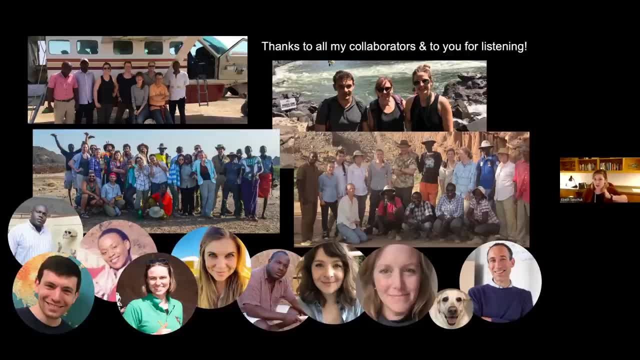 students from turkana university colleges here. hi, christine, you don't have to say anything, but i'm work in Turkana. is that the people who live around the lake today, which is not just one group, there's many groups- but the Turkana people do not consider themselves the descendants of the people who made 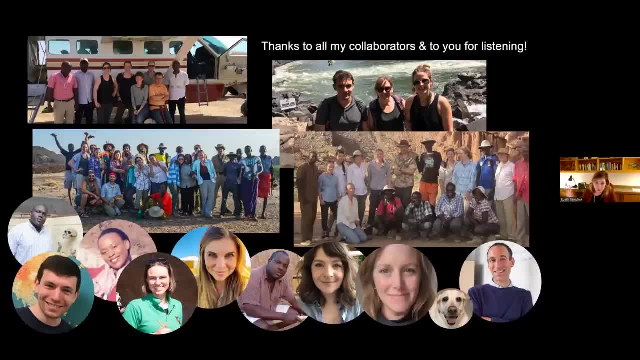 the pillar site. in their own oral history they came from Uganda like 300 years ago, but they are- they do consider themselves- or many of them do- kind of guardians of the sites and they want to work with the National Museums of Kenya. they want to work with Turkana Basin Institute and Turkana. 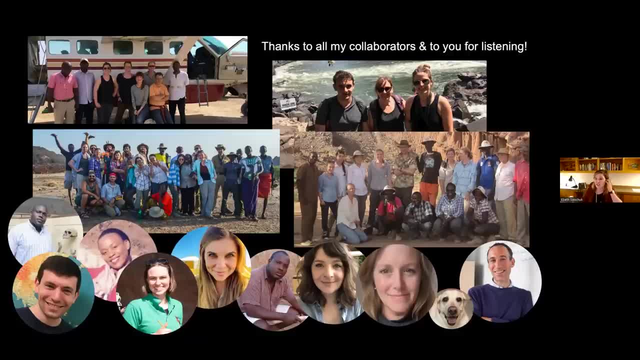 University College to try to protect these sites for their cultural heritage, and so so far we've been really really lucky and having great support for doing this kind of research. a lot of excitement about the same kind of questions we have and actually getting some questions, a lot of my work. 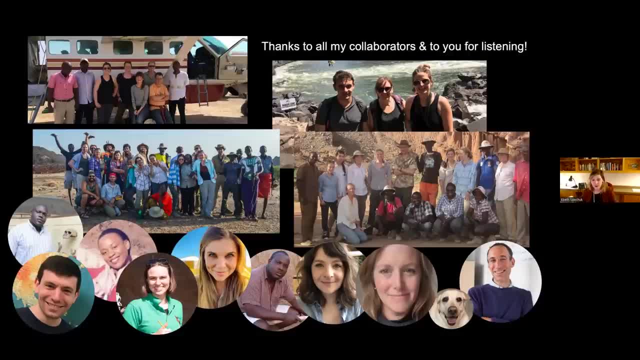 on health has come directly from the conversations I've been having with people out there and so so far we're really lucky. but we do this work with support and of course you wouldn't do this work if we didn't have that kind of support. but in terms of the sites themselves, they're kind of 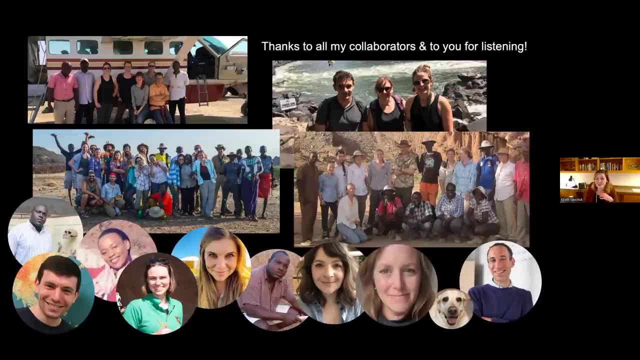 discovering with us what these sites are about. you know, the folklore of these areas is that the pillars were dancers turned to stone by an angry. you know the folklore of these areas is that the pillars were dancers turned to stone by an angry deity. but um, there's lots and lots of great knowledge, communication and co-creation there. 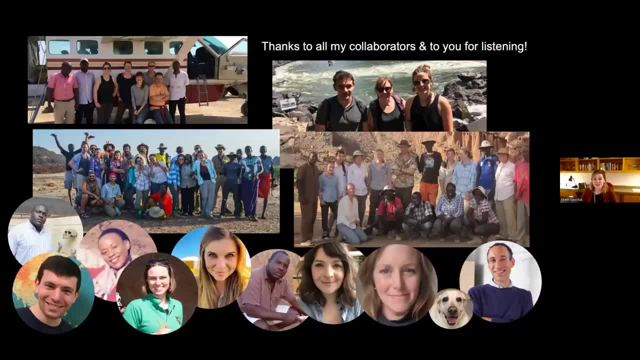 about, you know, the archaeological evidence of what we're finding with these sites, and a lot of pride thinking about the absolutely amazing complexity of these places and the amount of effort that went into them in terms of this being in this part of the world. um, in terms of your, 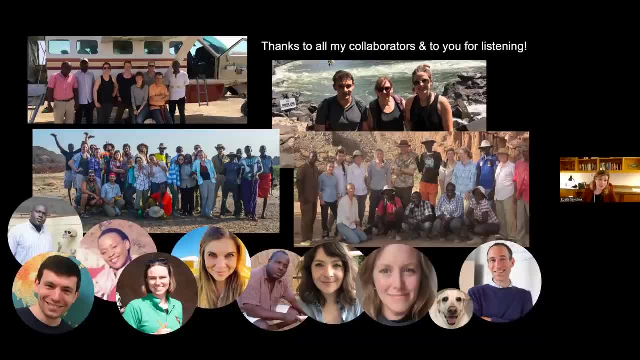 second question about the status: yeah, so this is a real pickle because we don't really have habitation sites from this time period. there's this one called Dongodien, which is public in the 1980s, and Emanuel N Diemes continued his work at that site and it is very culturally. 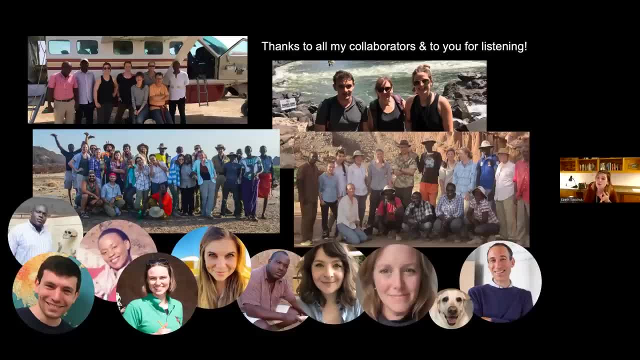 connected to the pillar sites in terms of the type of stone tools, in terms of the pottery that we see. again, we've got animal bones and it's really hard to infer kind of quotidian things from the pillar sites because it's like trying to understand, you know, like Italian society from the Sistine Chapel. 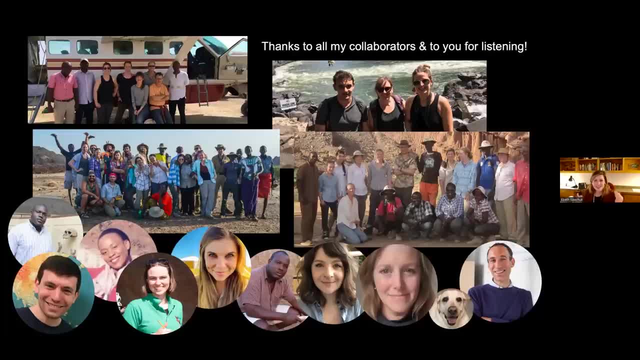 like they're the most amazing places. it's really hard to look through the lens of that mortuary site and we also haven't excavated a large proportion of the sites, of course, which is intentional, because it's really hard to look through the lens of that mortuary site and we 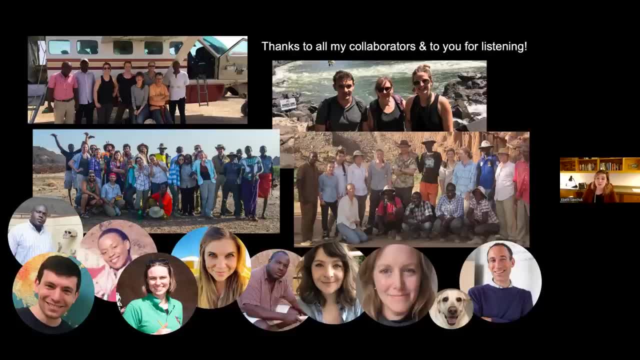 want to leave most of those people, uh, in the ground, which is why we're using things like ground penetrating radar. but what we've seen so far is that it really does look like the people buried at the site are a cross-section of society. so you know again, the the little, there's many individuals. 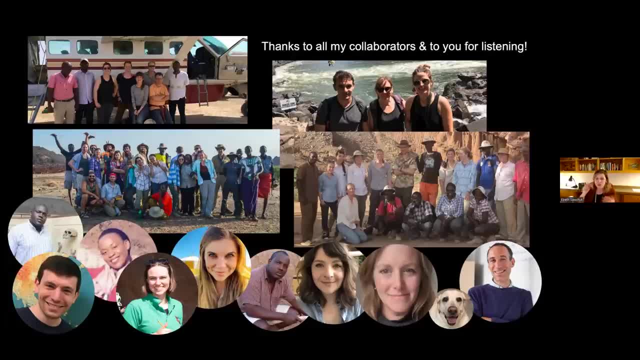 there who are like newborns when they died. so of course, at that point you know they don't have any of they don't. none of their status would be earned, it would all be ascribed status. but at the same time, like even they have little beads and almost everyone has something, but it's idiosyncratic, it's. 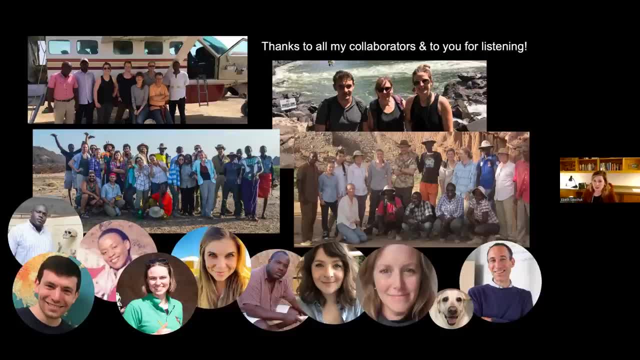 like the number of beads, it's not that kind of thing. so it really just does look like these places were super important for a people to be included and be a little bit of themselves, to go into these sites as well. but that remains kind of an open question and it's structuring a little bit. 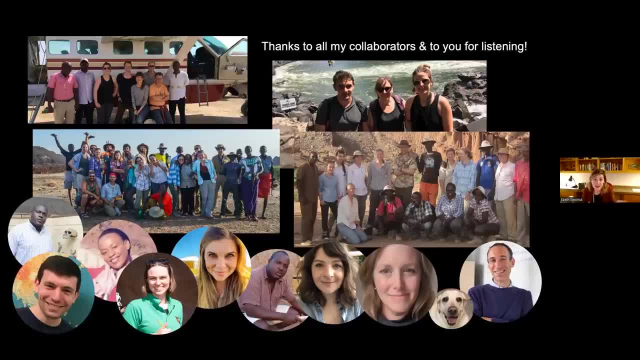 more. we're very careful thinking about which, what we want to dig now and if we're going to disturb these sites. it's much easier to do salvage archaeology, like at Locom when things are already coming up. you have to think very carefully how we want to dig these sites. but that one woman. 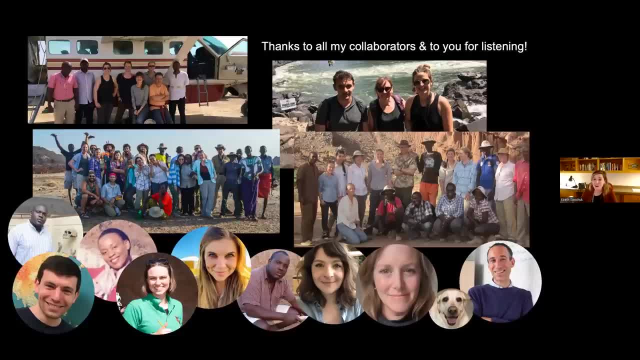 from Monomania that had all of those beads is kind of a big open question for us, wondering if we would start to see variation between these sites and variation between individuals. but so far we have no evidence that these were hierarchically organized people. it really does look like this. 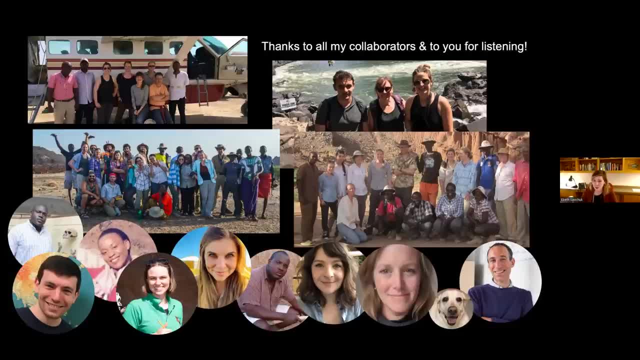 was a community works kind of thing where everybody got together to create these sites and then make sure everybody was buried with like something special that represented them. so it's still a work in progress, but no, we're really. I mean it's. it's a fascinating thing, just like one stone bead would have taken how many hours to construct. 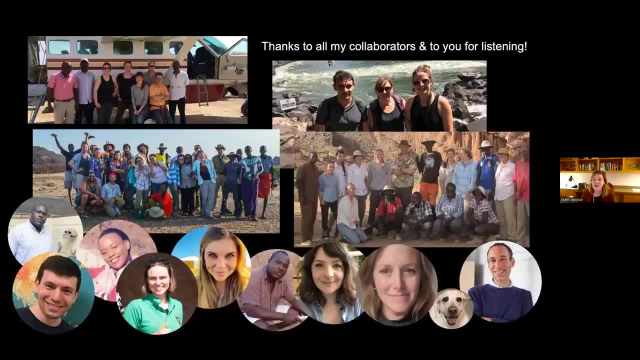 and then somebody's buried with like a hundred of them around her neck. but it also really lets us think about that mosaic, because all of those stone beads- based on some work that's soon to be published, but it's also in my 2019 paper about the sites- it looks like all the sources for the stone. 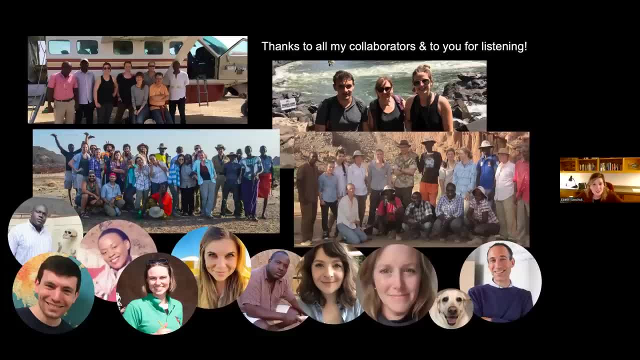 beads are local. same thing. there's new types of stone tools, but all the obsidian looks local. so it's this, is this complicated mosaic where it seems like you know herders coming in wouldn't really understand that environment. but if there's a lot of stone in there, it's going to be a good. 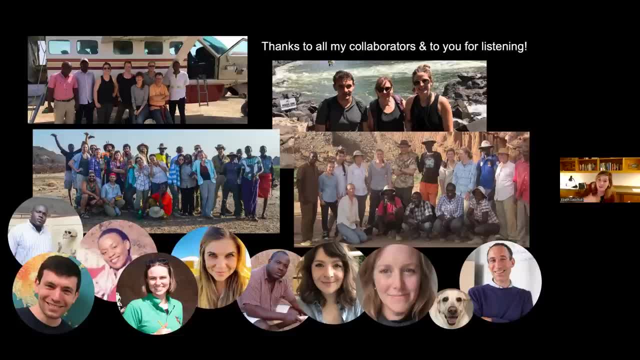 little thing to do. so it's really interesting and we're gonna know a lot about it in the meantime. so- and this is a really interesting topic and a lot of the work that's being done about the ook and if we can take a look at, what are the sort of the, what are the kinds of the? 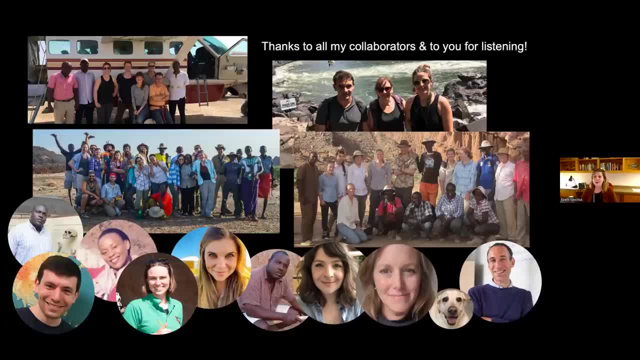 kinds of the main points of interest and the kind of the kind ofات are in the work of the Texas uptake. so what do we know about the history of theみ? I think we really need to know that the, the, the kind of the, the work that has been done around the local. 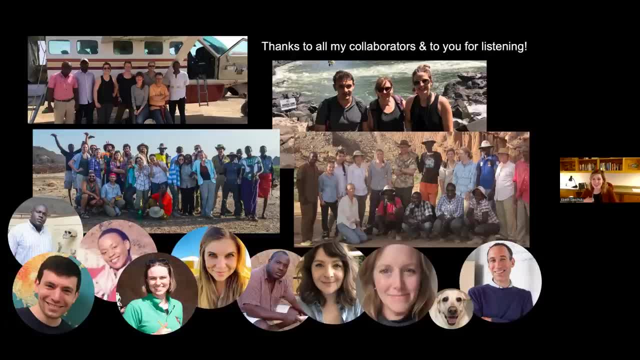 mosaic is the one that's needed to do it. and also, I think it's important to know that there's a lot of evidence that you can find that I don't have ten years ago about this, because there's not a lot of evidence that we can find about this, but you can find a lot of evidence being 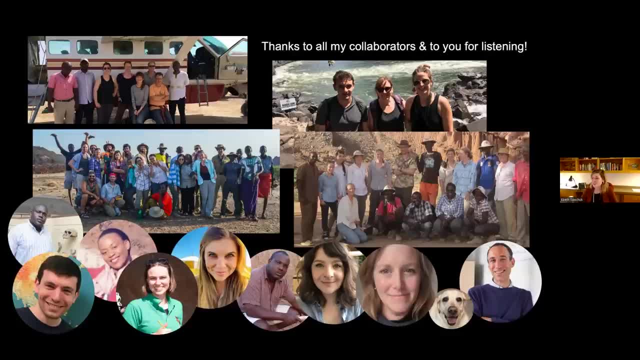 but it sets up a bunch of research and i think this is one thing that's really important: once you, you know, solve the mystery of the pillar sites, you're just at the beginning of the story, because now you have all of these next level questions to really understand. yeah, what does? 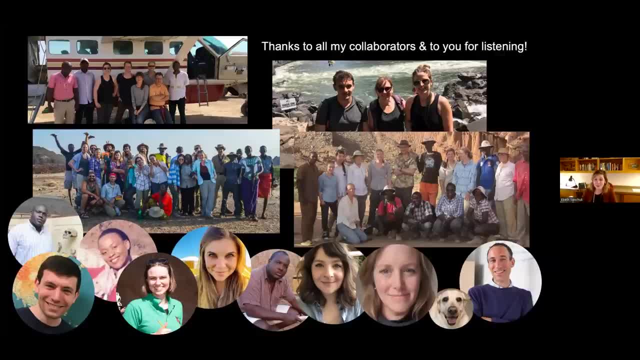 life look like in this time period. and and i always say- and people make fun of me because i work in a natural history museum with dinosaurs, but if i had a time machine, this is where i would go back to see how these sites are constructed. forget the dinosaurs, this is way more interesting. 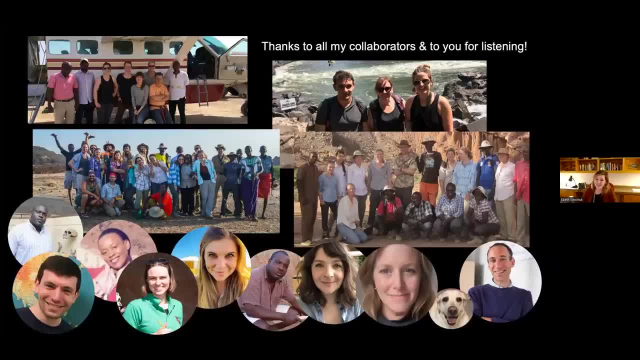 thinking about the humans. well, thank you. wow, thank you very much, jared, and we have another question from peter, if you'd like to ask um sure. thank you um fascinating talk. subject matter: i'm peter annick from brandeis university in massachusetts, and i had a question also about 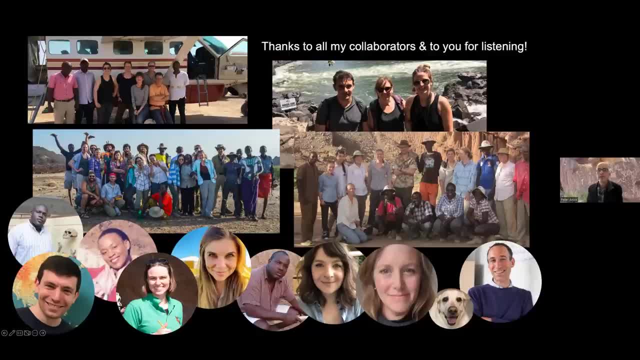 the pillar sites. um, you said that there was no evidence that cattle were used in moving the stones, and i was just wondering what uh such evidence would look like and whether such evidence does occur at any other megalithic sites. good question, i mean, the problem again is we really only have the one uh? 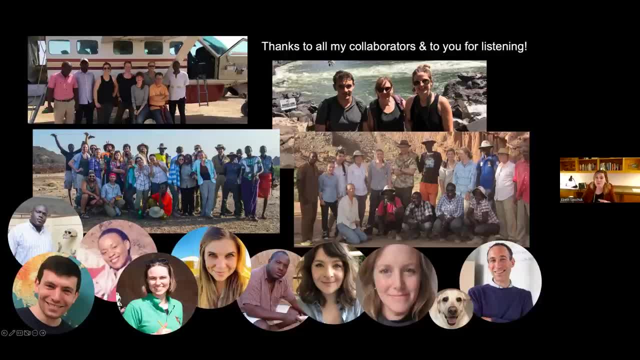 the only one habitation site, so it's not like we have multiple sites around the basin. so i guess there's no evidence. but also, an absence of evidence is not evidence for absence, of course, that we always have to remember. but at this point we're not seeing any indications of 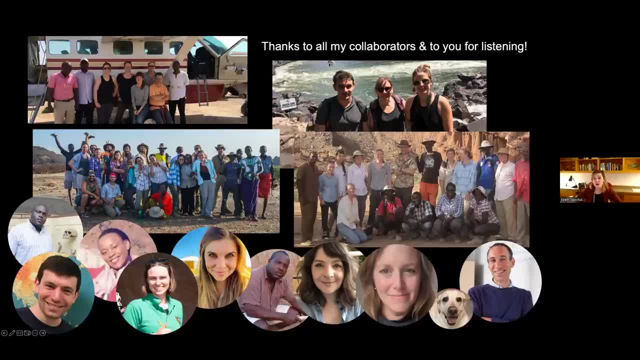 anything complete enough that would be able to assess that any animals dragging- and a lot of this idea also comes from, you know, talking about how herders today use their animals in these kind of areas of the world and that they would be using them from this kind of thing- and so far we haven't found anything that would suggest to us that. 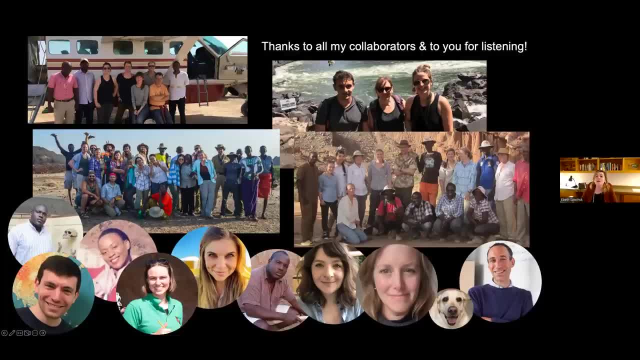 people are using animals to move the pillars. it's possible. um, usually, if that's the case, it would be donkeys, and we don't see donkeys quite here at this time, so it would just be cattle, sheep and goats, and we think mostly sheep and goats. um, but yeah, i think i've. i skirted over that for the sake. 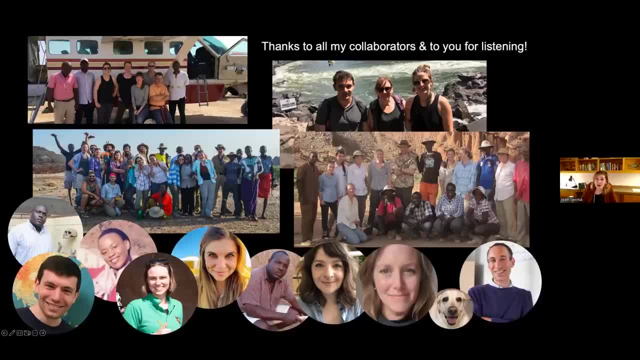 of time, but in fact that itself is a whole big question about how people were quarrying and moving these pillars. i think also important to remember is the pillars were actually put on as like a final aspect of these sites, so based on the radiocarbon dates, uh, throughout. 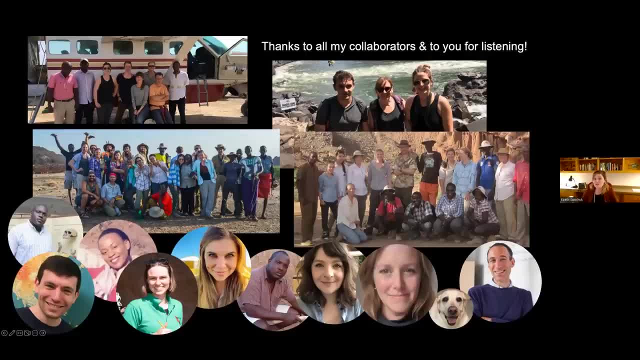 these mortuary cavities and we have several of these sites pretty well dated at this point. you know, it really looks like the sites were conceived and started around five thousand years ago and then used for several hundred years. so the people at the end who filled up the cavity, who then capped the cavity with a 50 to 50 centimeters to a meter of sediment, 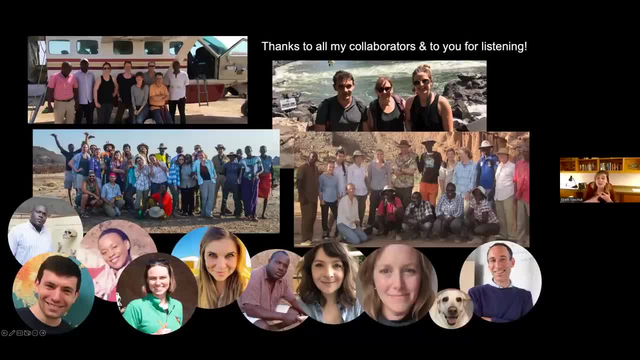 and in that sediment we see other things like oxygen, eggshell beads, we see broken pottery, we see actually some isolated human remains and then, as a final thing, they're going to put the pillars. they're going to emplace the pillars in these platforms and then actually put on this beautiful 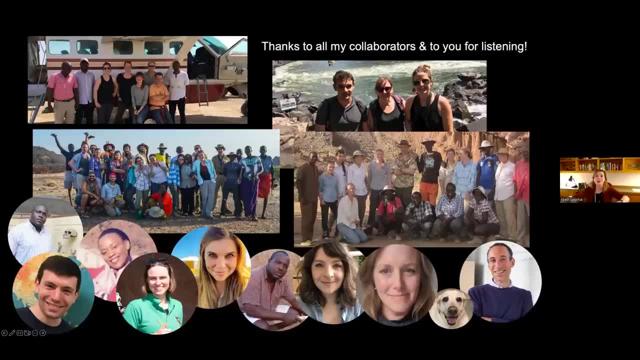 shiny black basalt pebble layer on top of these platforms and then potentially create these structures and then actually put on this beautiful shiny black basalt pebble layer on top of these structures and then actually put on this beautiful shiny black basalt pebble layer on top of these stone circles. 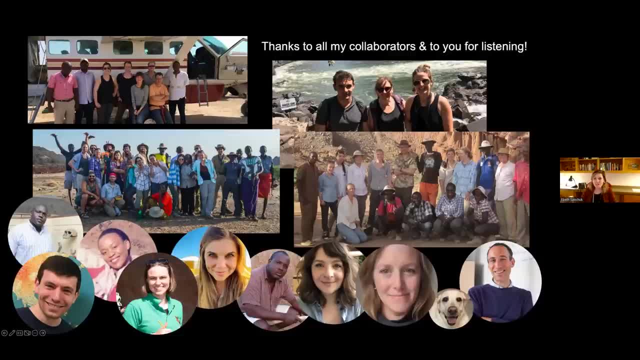 um, that happened like hundreds of years later, and so you know it's also hard to look at a habitation site from the earliest time in that period and look at that and then infer what people were doing with those animals a few hundred years later. so the big issue we have here is a lack of 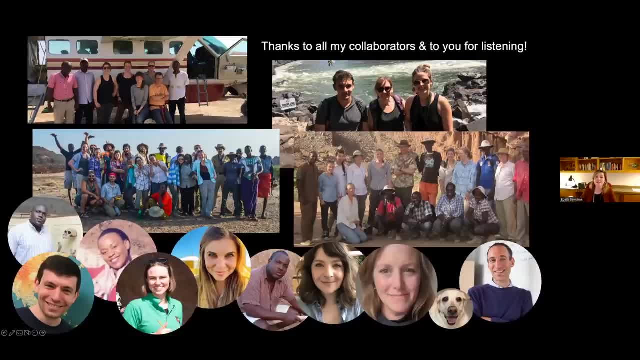 habitation sites that would indicate to us what exactly people are doing and what kind of like you know, the everyday tuesday looks like, not just when you put someone in these sites. and uh, actually, i will say again, this is work that that Christine Chepkrier, who's a Turkana University College student, is working on. 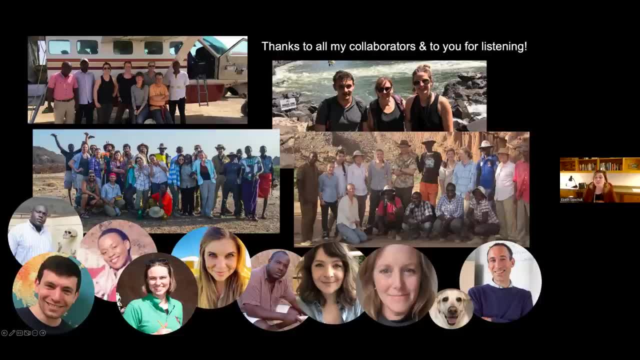 right now trying to understand one of the potential habitation sites in this time period and really understanding what people are doing. that would give us a much better sense of what it looks like in the everyday. So good question. Yeah, I would imagine that the bones of the 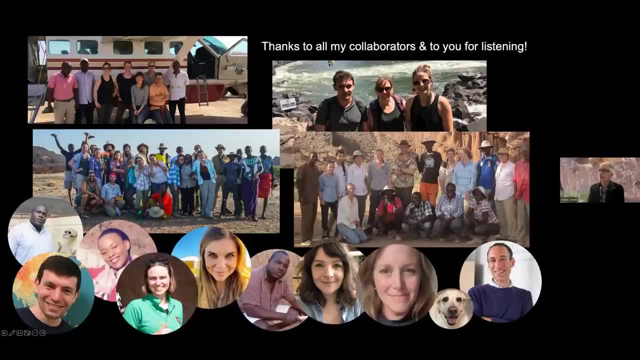 animals might give you some idea where they're used: as beasts of burden, right Yeah, and so far, the vast majority of cattle remains, especially from this time period, are just incredibly, incredibly fragmentary. One of our zooarchaeologists on this project. 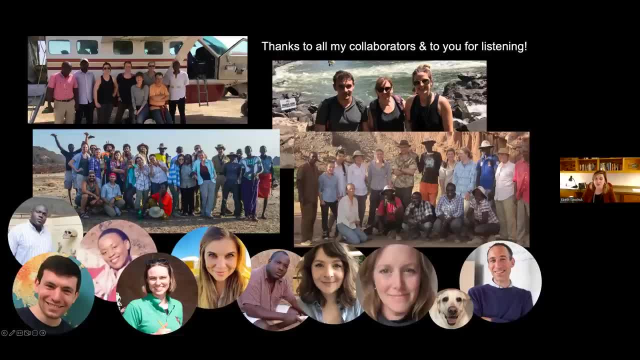 Annika Janssen from University of Tennessee, Knoxville, you know, basically categorizes most things as like ASB, angry shard of bone. So you know, the preservation at these sites and intercana in general is just really horrific in terms of keeping bone together. And then we 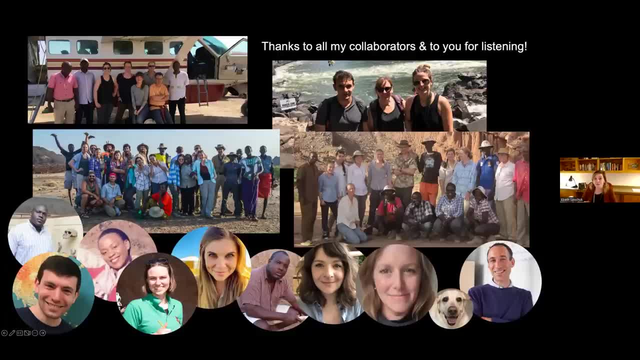 also see, of course, a lot of processing by the time those animals enter the archaeological record, because you know, we think many of them were probably eaten. Looking also at pottery residues and understanding, there's evidence for meat cooking at this time period, exactly, kind of. 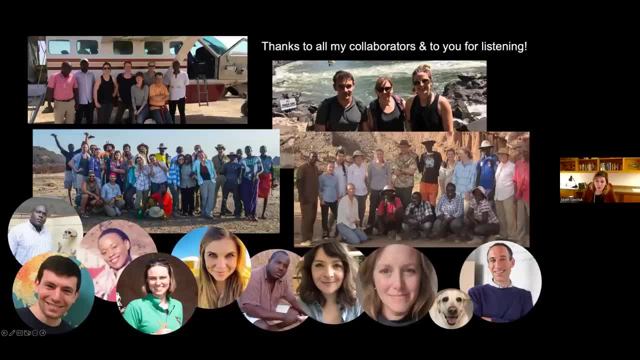 what we would expect. That's Kate Grillo's work from the University of Florida. We're just not finding a lot of whole animals. So not only do we have not a lot of sites with animals, but we have in those sites no whole animals And it's kind of confounding that whole thing, But it is really. 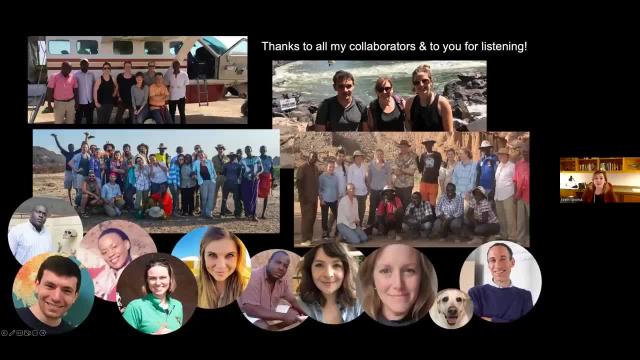 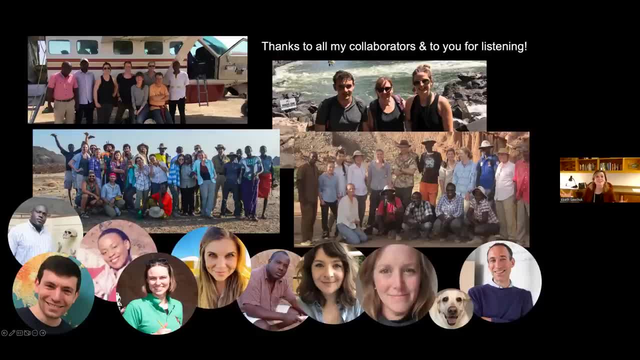 contemporaneous with the pyramids. You know we're not seeing a pharaoh here dictating. We don't have any indication of that yet- that we're seeing some kind of organized- you know labor situation here. And if we look at contemporary pastoralist social structure we would expect 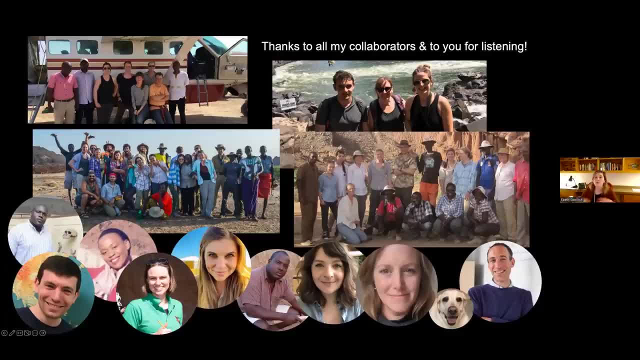 to see something a little bit more heterarchical with, you know, a group of people who are making kind of decisions, But there's just so many questions now that we figured out that these are, you know, extreme, complex, amazing cemeteries, to think about the nuts and bolts and the logistics. 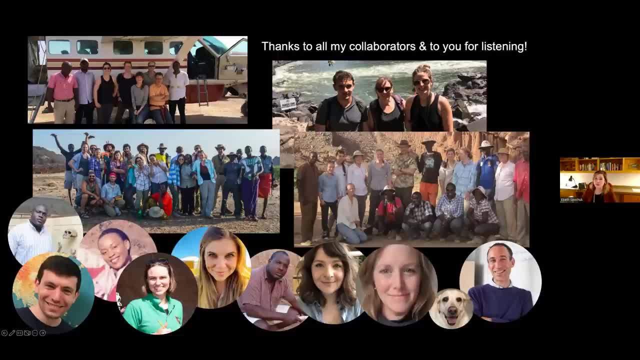 of how that actually went through. And the pillars are just. they're the most obvious signs on the surface of this is happening, but they're kind of like an afterthought to the digging out the giant mortuary cavity and everything else. So it's just one piece of a very complicated and 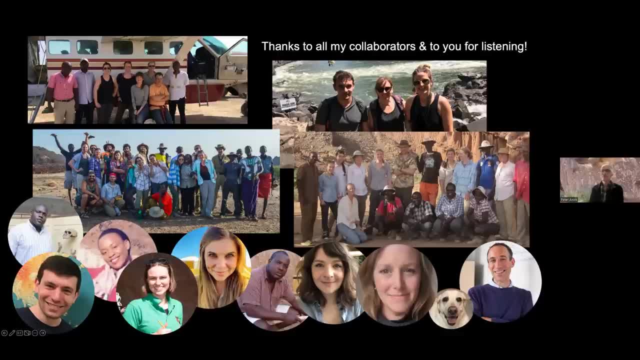 fascinating puzzle. Thank you, You're welcome. So do we have any any other questions? I do. I do have One myself, actually, about how there's- how you say there's this- this sort of episode of gene flow, sort of from 50 to 20,000 years ago in in sub-Saharan Africa. Is it? is it the case that 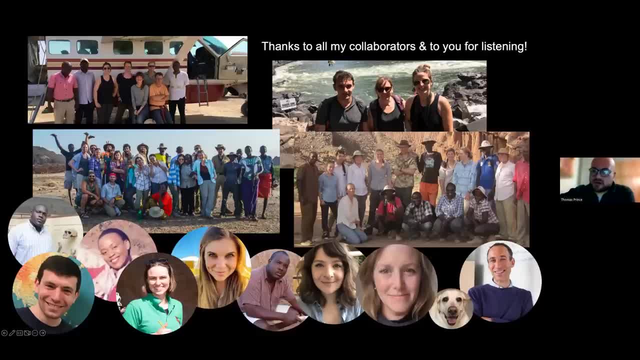 we don't see any gene flow between sub-Saharan Africa and and North Africa at all in that period, And is it just in sub-Saharan Africa? That's a good question And in fact that's something that there there are sequences from Northern Africa. 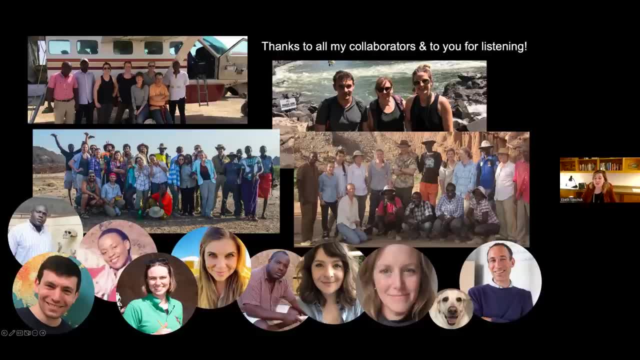 And they're actually sequences from Pleistocene Northern Africa, And you know my understanding- I would have to look into this more in depth- is that they're really quite different, And so for our paper we focused on sub-Saharan Africa because we were interested in the later. 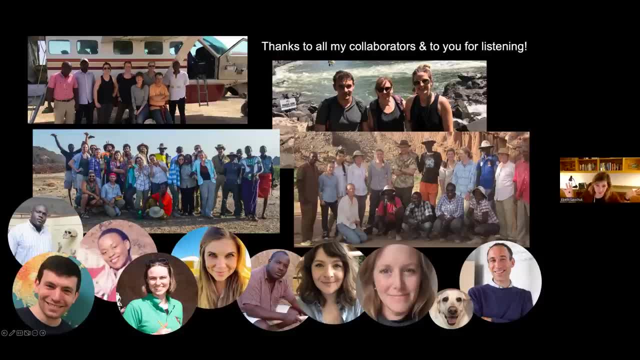 to the middle to later Stone Age transition and different things are happening north of the Sahara And of course, this is also a question of what the Sahara looked like at different times. If it's, you know, if it's a barrier geographically to populations coming together. 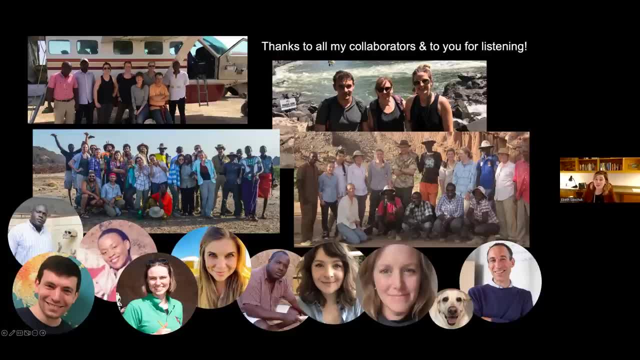 which we think it was at many different parts of, you know, the glacial period, But from what I understand they're, they're really different. but I think that there's some interesting work to potentially explore And I know there's been a little bit of. 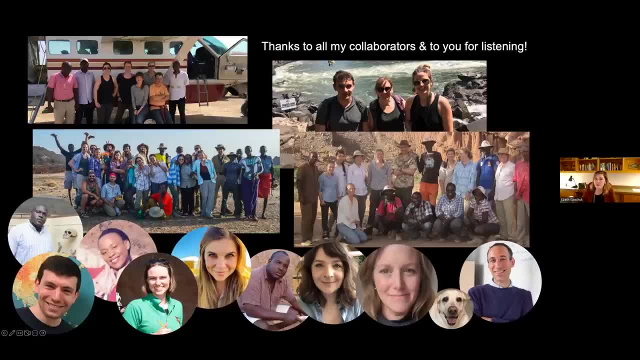 work done in terms of, like the margins of the Sahara later. But yeah, from what we can understand, the picture is quite different. but I would have to to look more into that And it's an interesting question Just in Southern and sub-Saharan Africa, though. just the fact that 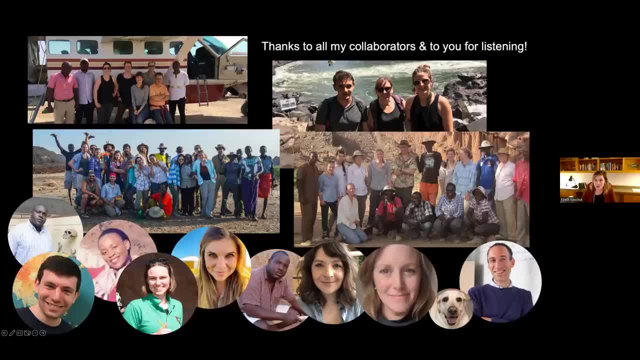 we do see that profound amount of gene flow really kind of opens the question about what we're, what we haven't considered before, that we might not be seen because of sampling issues. So one thing that came out of that was like Central Africa is actually a pretty major player. 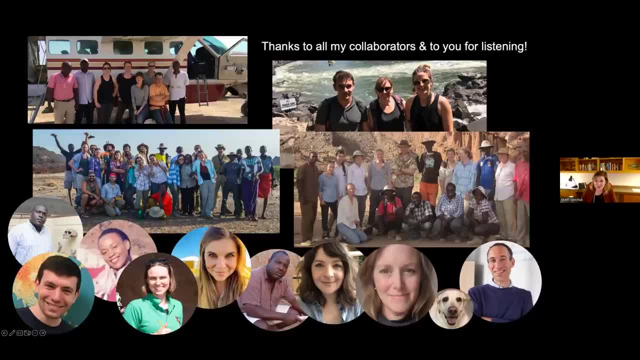 when it comes to understanding Pleistocene population relationships and human evolution. And you know there's a few dedicated archaeological projects which have really moved our understanding forward of what the Pleistocene looks like in Central Africa. but compared to like archaeology in Kenya, where you know you show up, 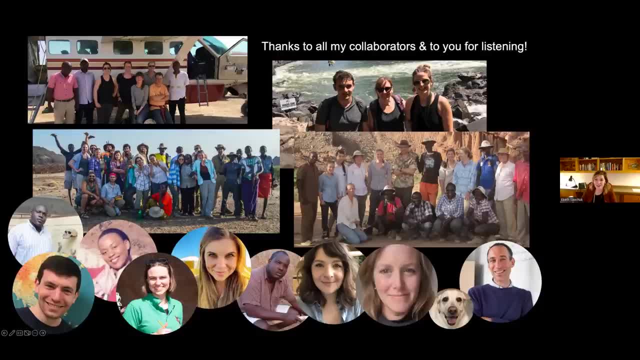 you know in the summer for your field project, and then you know around the cafe at the National Museums of Kenya and everyone's an archaeologist. You know. it's just we don't have the same kind of density of archaeological research in those. 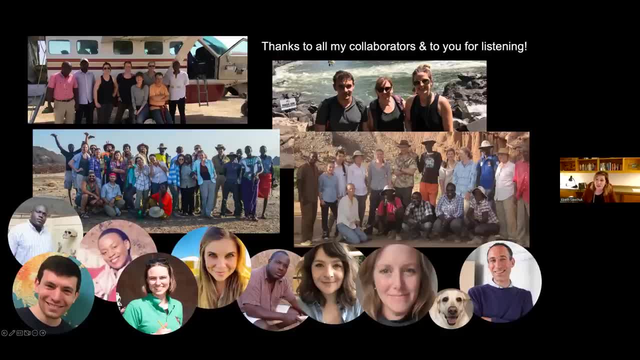 kind of areas, and part of that is because of funding, but also part of that is because of logistics- Lots of areas that we really would like to fill in the gaps of the African archaeological record right now are not easy to get to or safe to get to, and this is always kind of a factor we 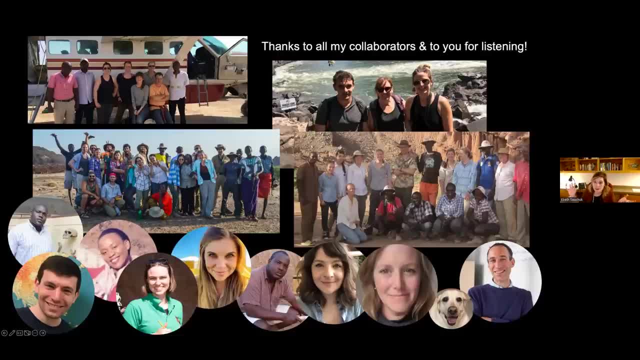 have to consider when we think about what continental scale processes look like. So the fact that we're able to see evidence of a lineage that looks like the Mbuti across such a huge swath of eastern and southern Africa also kind of really challenges us to think about what other parts of 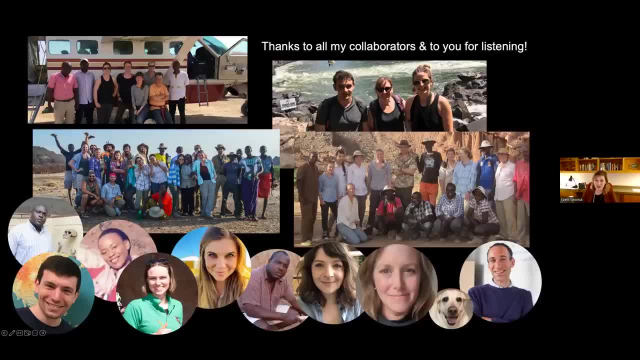 the continent might not be in the story right now. A lot of the work in northern Africa has been done, of course, in like the extreme north of northern Africa, where you're going to get better preservation. Obviously, there's huge areas of the Sahara that are not, you know, accessible right now, for 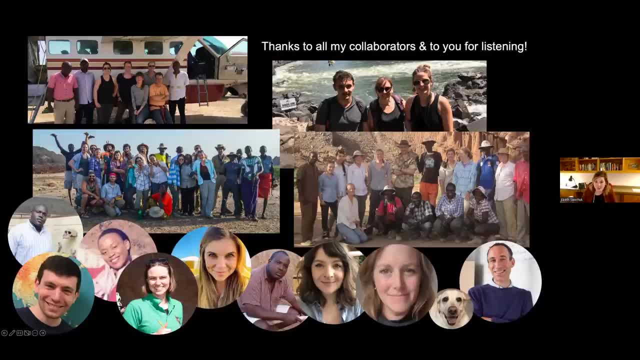 archaeological research. There's giant areas of West Africa that we know extremely little bit about in terms of the Pleistocene, and there's some very cool projects that are starting to look at that more. But this is where it gets back to, you know, this slide of the history of African. 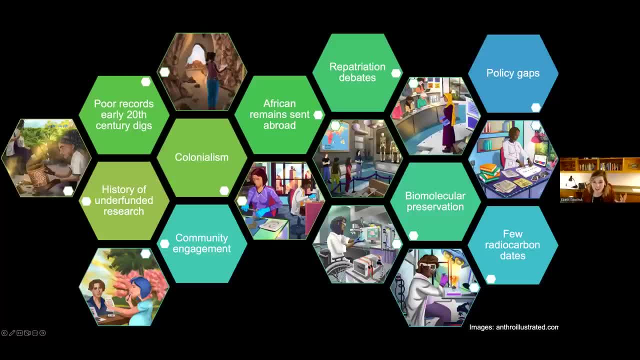 archaeology is actually having more of an impact on what we know about the past in Africa than sometimes. we're really quick to acknowledge That some of the stories that we're telling and some of the narratives that we're constructing, in fact we're really quick to acknowledge that some of the 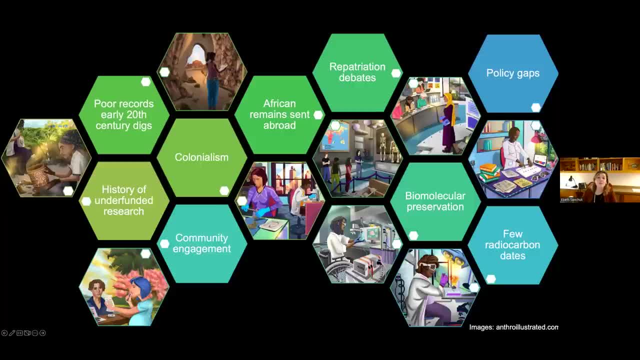 stories that we're telling and some of the narratives that we're constructing in fact have a pretty big confounding factor, which is that we just do not have sequences and we do not have samples, and we do not have artifacts and we do not have human remains from large areas of the 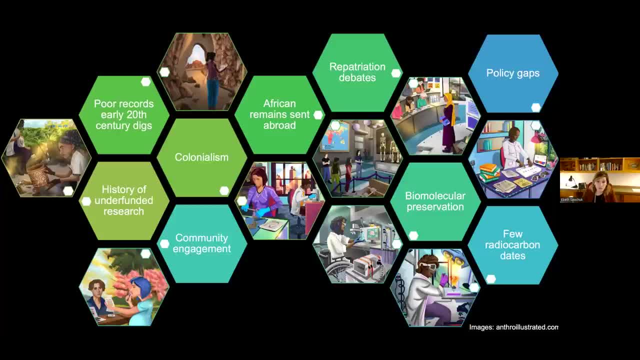 continent. And that goes back to my first point too, that Africa is really big and that you know. considering and comparing what we know about, for example, European archaeology and European ancient DNA, and then trying to look at what we know about Africa, it's just a completely different point. 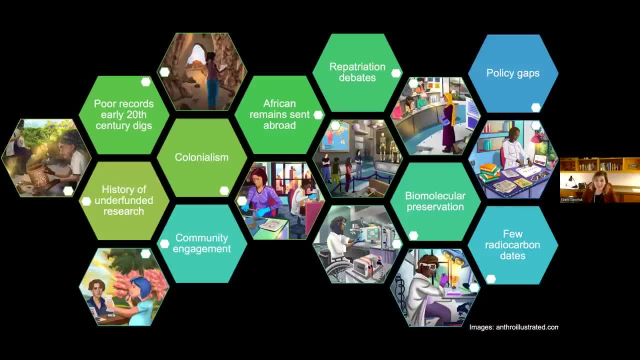 We also need completely different protocols to think about how we're going to do that work. We also need completely different protocols to think about how we're going to do that work. And again, with issues of the preservation and issues with, you know, the colonial history. 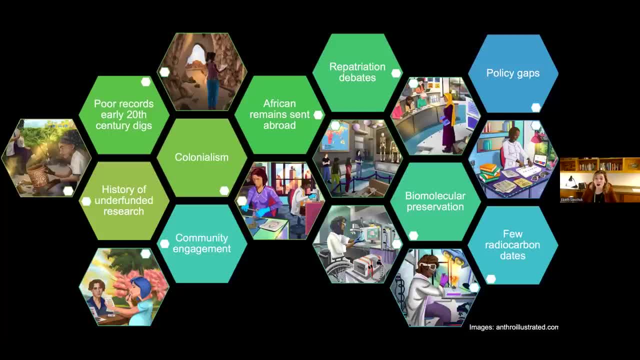 of many of the places that we're working. it's a complicated tapestry of doing archaeological research And I think that it bears repeating often that these are the limitations in all of our studies right now And then thinking about how to overcome those limitations. 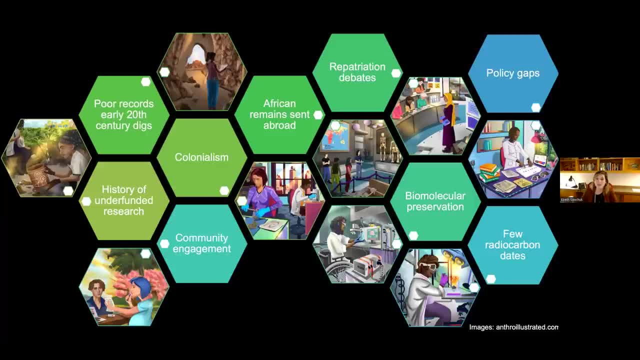 or, in some cases where we're just never going to get ancient DNA to some places, thinking about going back to how we can test archaeological hypotheses differently, Because we can't rely on things like ancient DNA. So it's a good question And I truly hope that that's.